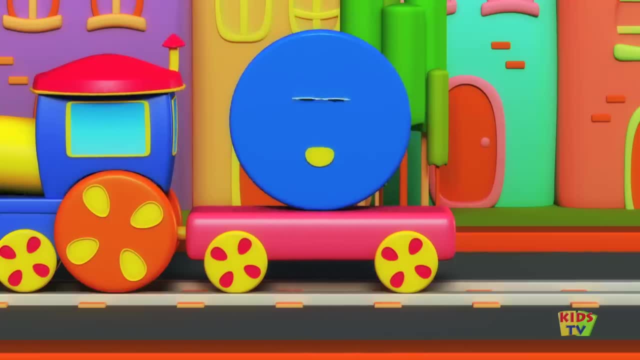 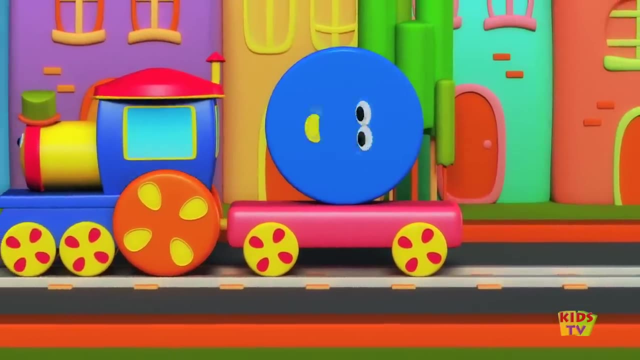 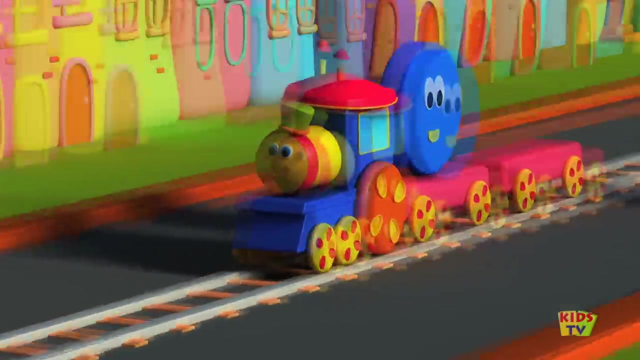 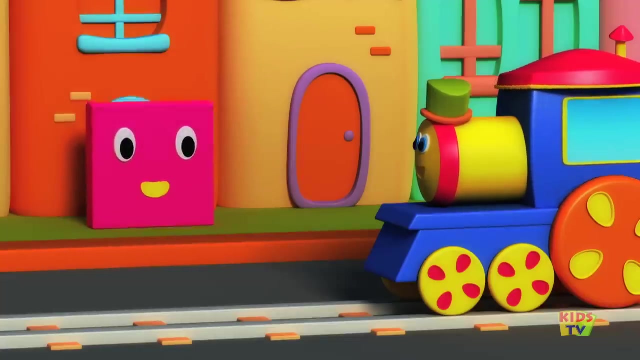 Mr Circle, Mr Circle. You're so round and round and round. You can roll on the ground, You can roll all around. Mr Square, Mr Square, Good morning. how are you? Take care of your four sides and your four corners too. 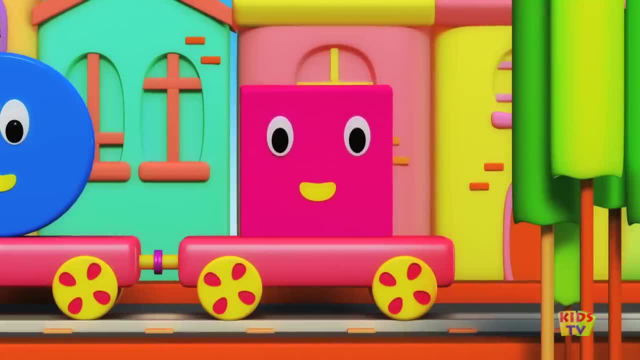 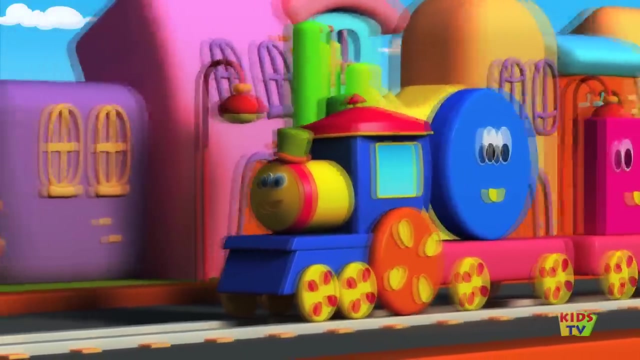 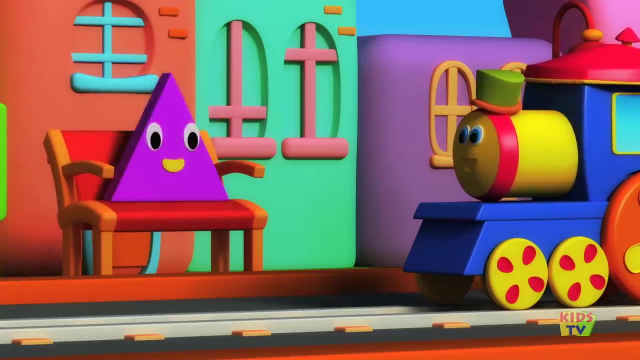 Mr Square. Mr Square, Good morning. how are you? Take care of your four sides and your four corners too. Mr Triangle, Triangle, You look like a pyramid. Won't you join me on my train, As Mr Square did? 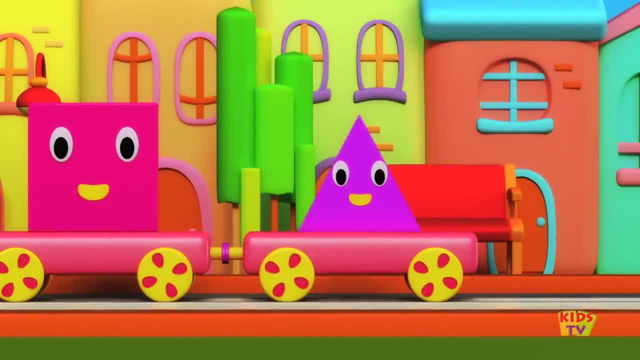 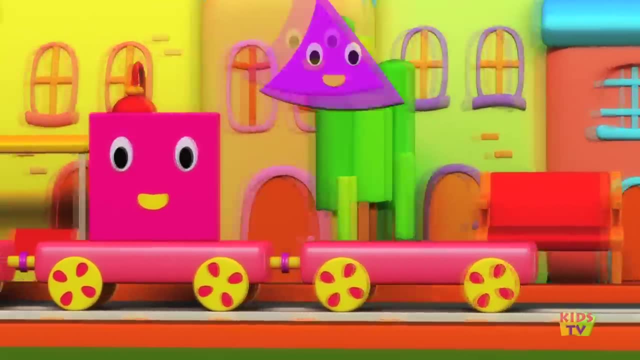 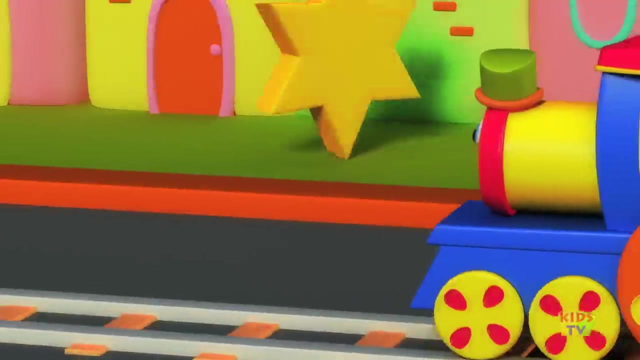 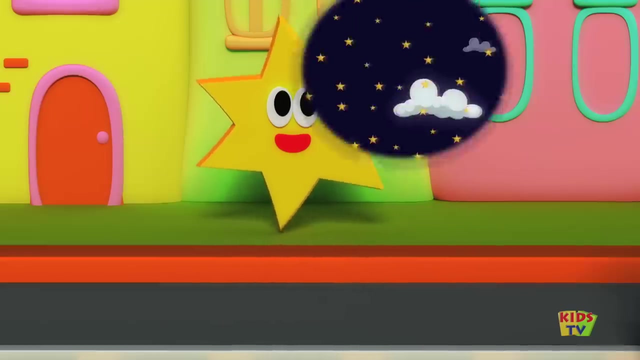 Mr Triangle, Triangle, You look like a pyramid. Won't you join me on my train, As Mr Square did? Mr Star, Mr Star, Are you looking at the sky? Your friends will come out in the night. So very high. 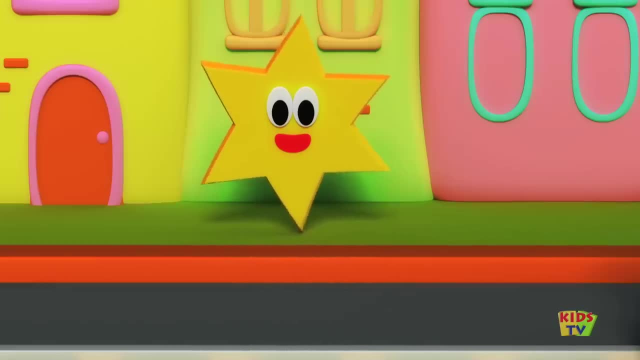 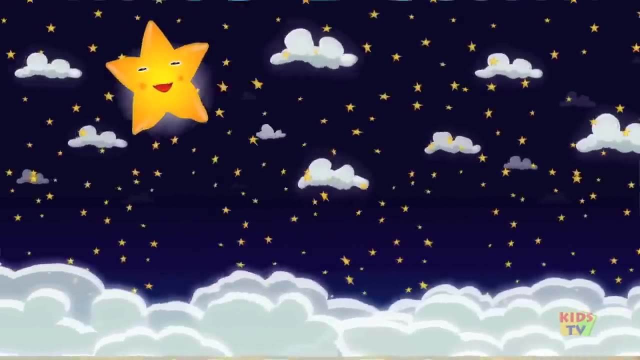 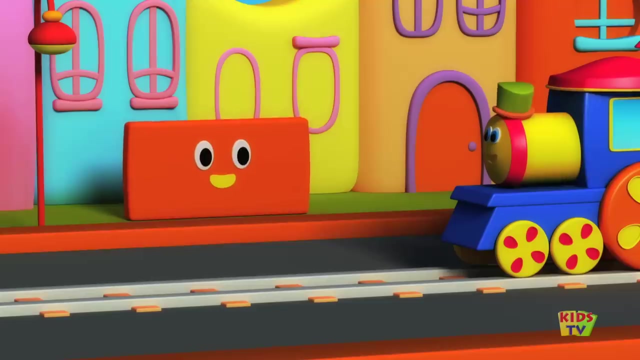 Mr Star. Mr Star, Are you looking at the sky? Your friends will come out in the night So very high. Your friends will come out in the night So very high. Mr Rectangle, Rectangle, Oh, will you join us too? 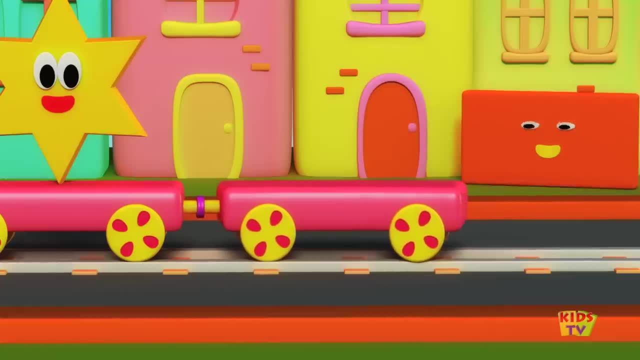 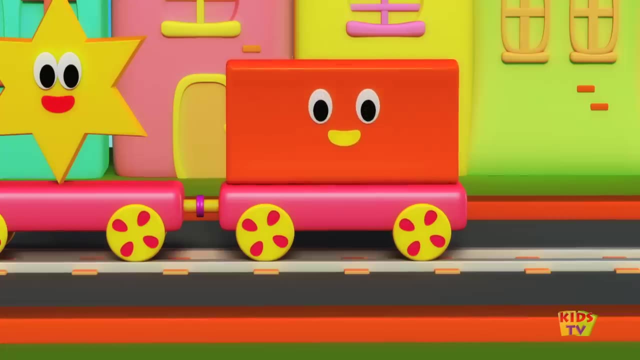 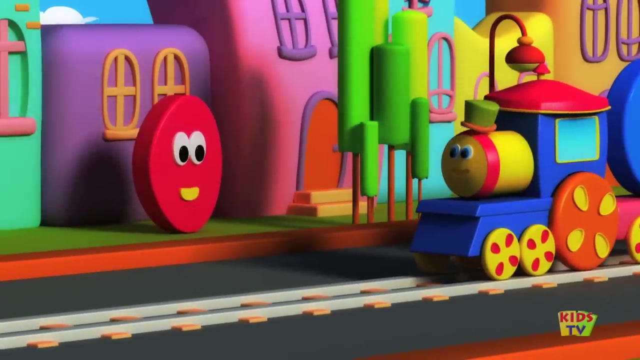 My wagons are comfortable and shaped just like you, Mr Rectangle Rectangle. Oh, will you join us too? My wagons are comfortable and shaped just like you. My wagons are comfortable and shaped just like you, Mr Oval. Mr Oval, Good morning. how do you do? 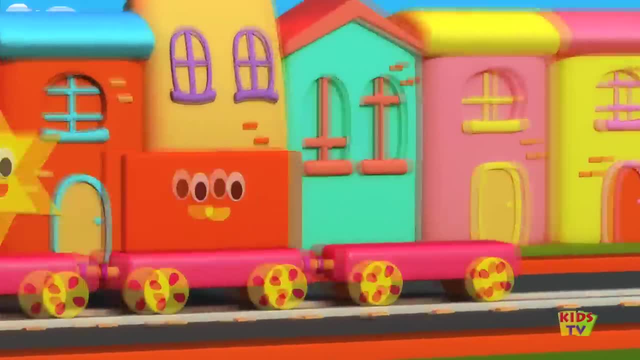 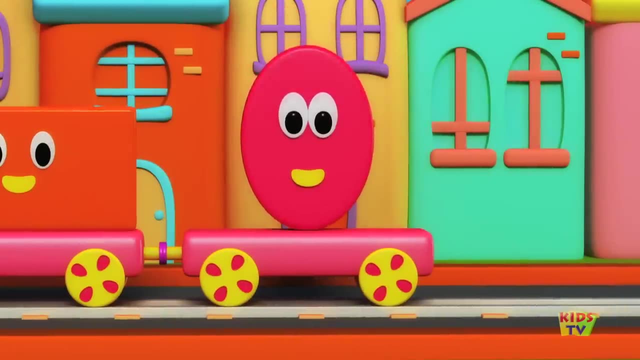 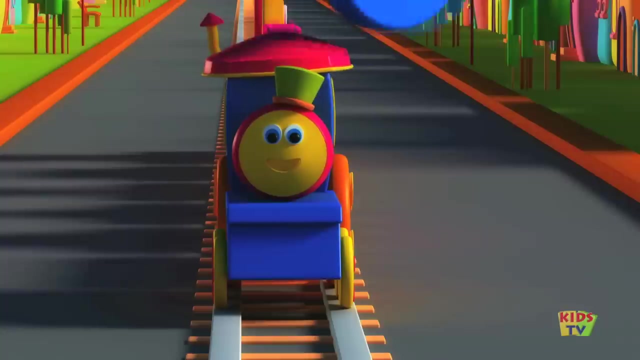 Look, your friends are all aboard. Won't you join us too, Mr Oval? Mr Oval, Good morning. how do you do? Look, your friends are all aboard. Won't you join us too? My wagons are comfortable and shaped just like you. 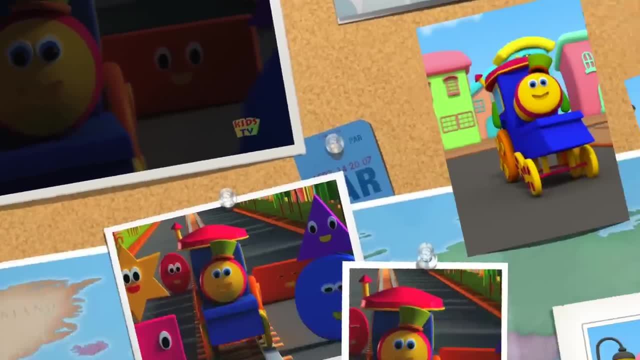 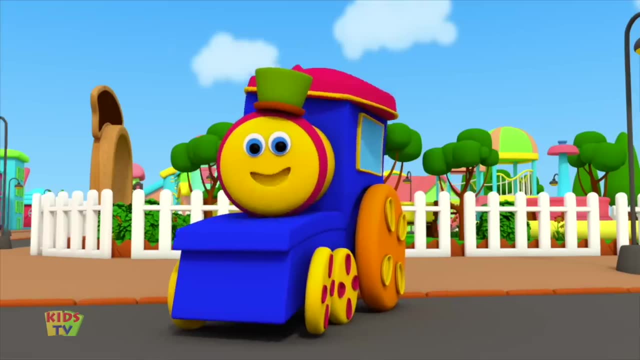 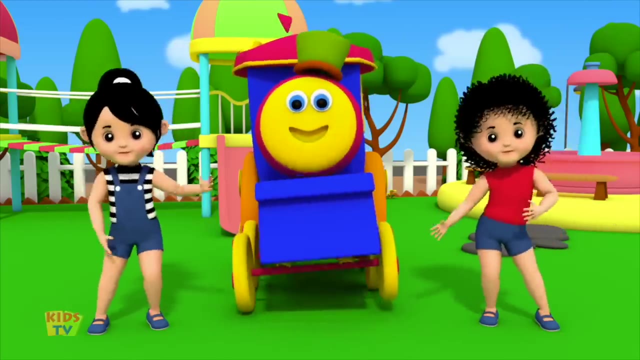 My wagons are comfortable and shaped just like you. Hey kids, welcome toità Bob Learning Street. Let's take our cameras and go click some colors. Let's take our cameras and go click some colors. Let's click some colors with our camera. 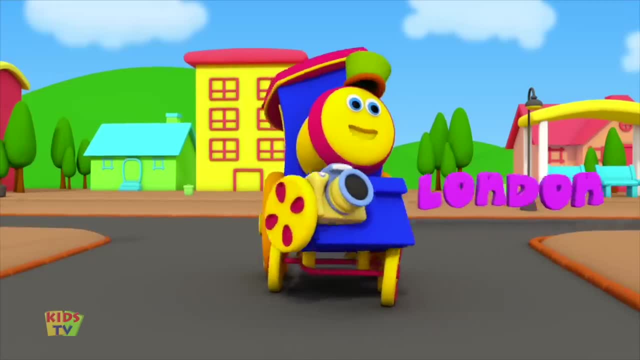 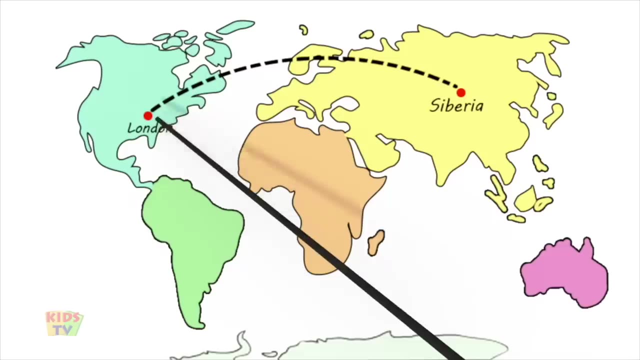 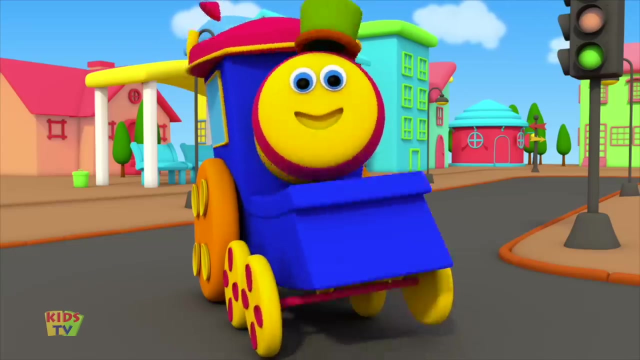 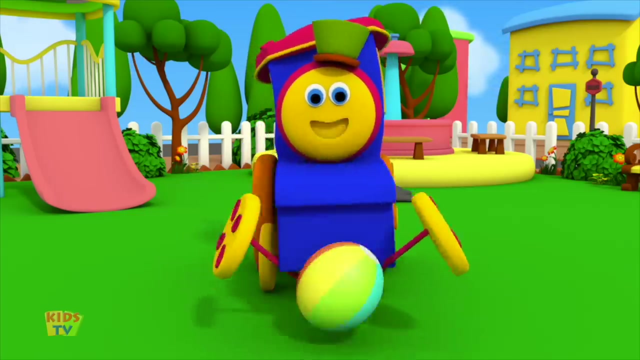 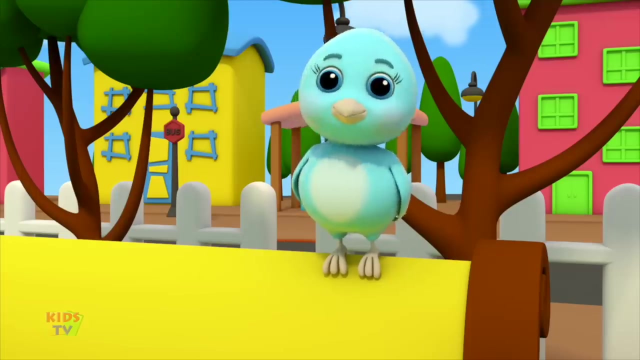 Where are you? from London to Siberia, let's click some colors with our camera. from London to Siberia. sunflowers in the garden are yellow. blue is the ball I'm bouncing. the wheels on the bus are black and white are the birds that sing. Oh, green are. 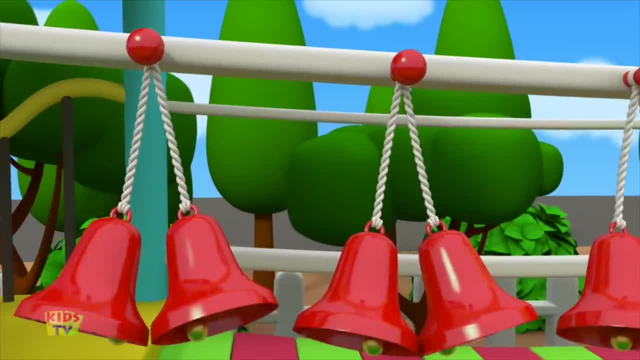 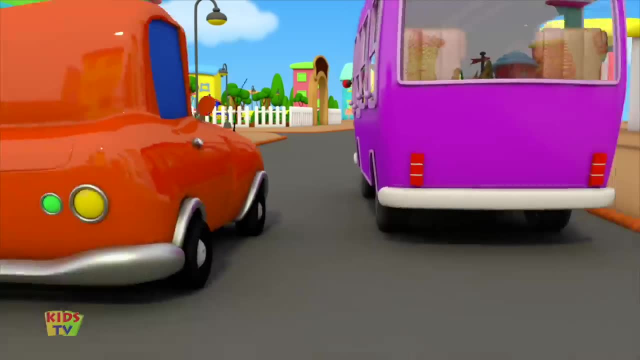 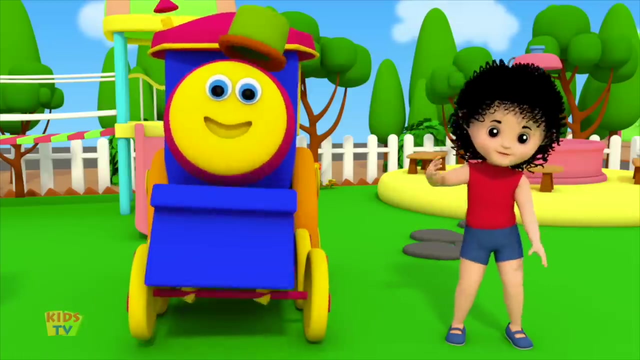 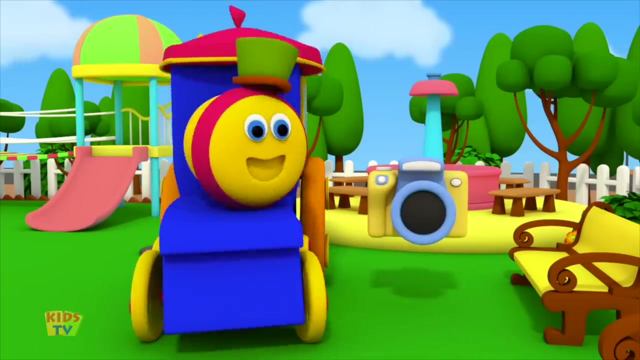 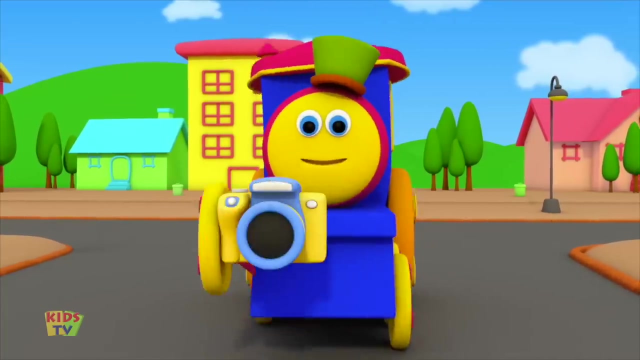 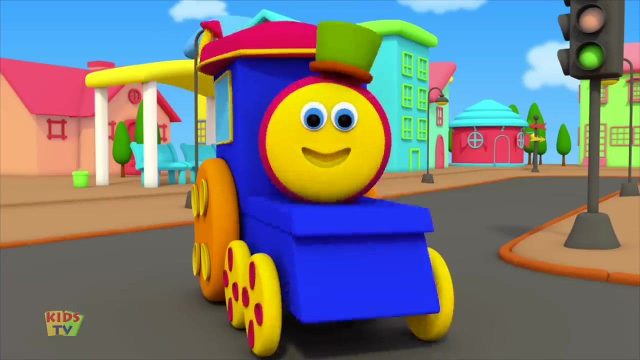 the veggies I am eating. red are the bells in a row, pink is the dress on the doll and orange is the car going slow. let's click some colors with our camera from London to Siberia. let's click some colors with our camera from London to Siberia. Oh, gray, are the dancing numbers. 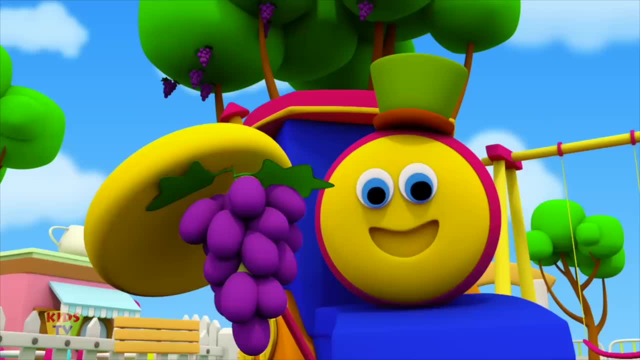 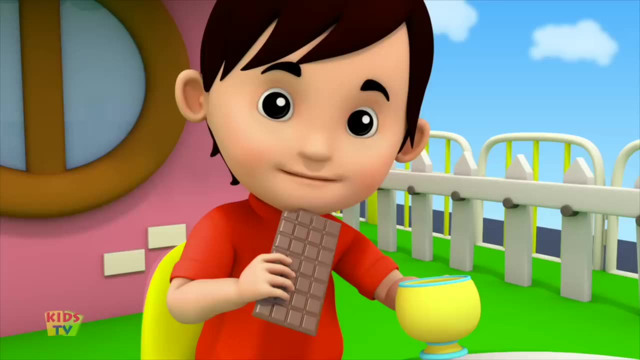 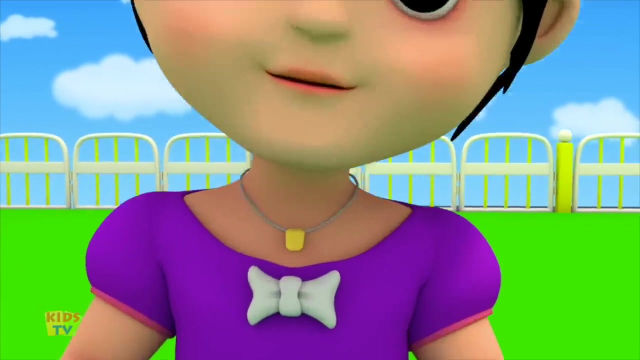 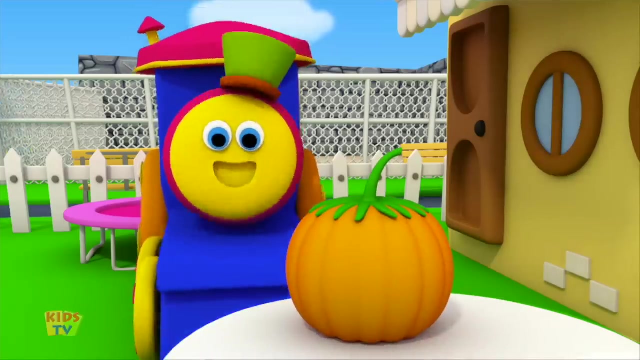 violet, the berries on the tree, cream are the doors of the house, cream are the doors of the house. and brown or chocolate and coffee. Oh, gold is the crown on the key, silver the necklace on the Queen indigo. the color of the bicycle, orange is the Halloween. 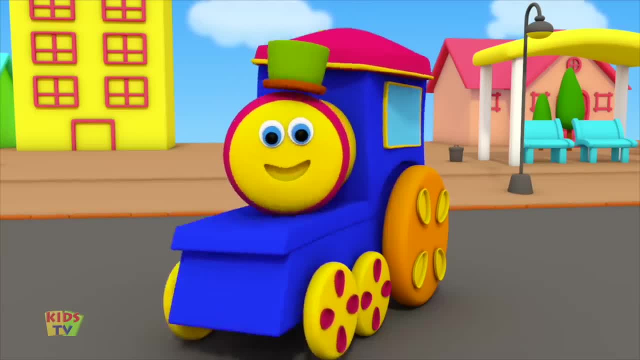 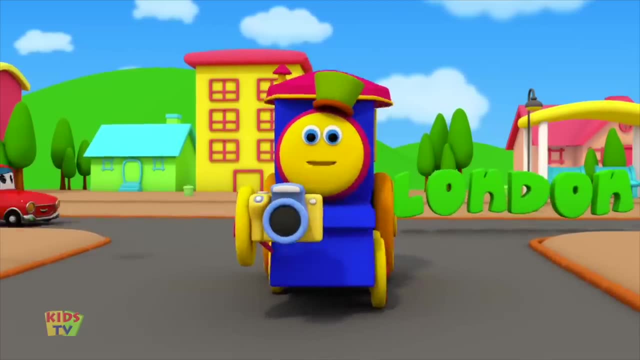 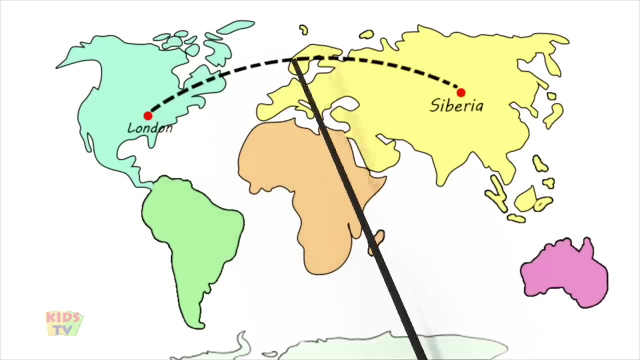 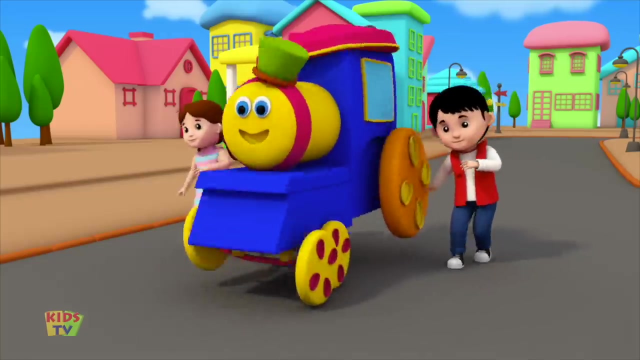 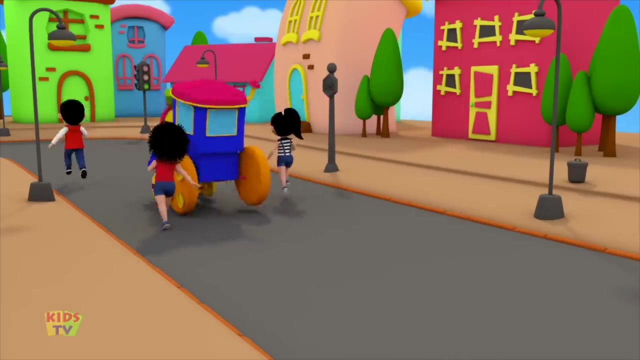 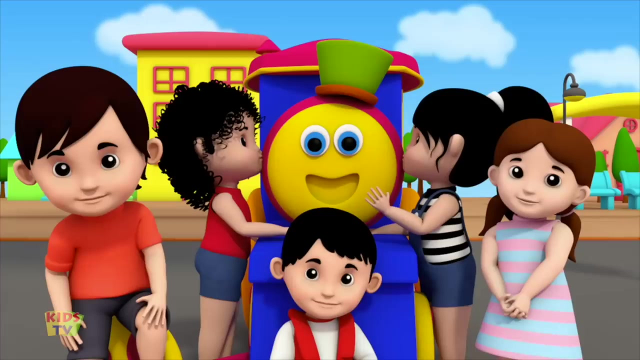 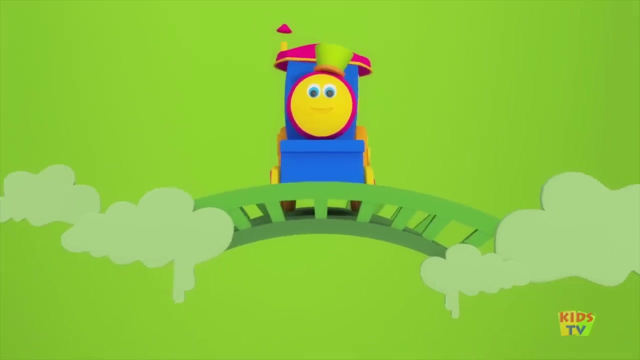 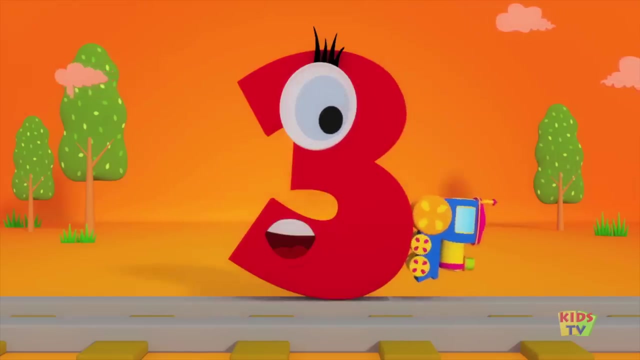 pumpkin. let's click some colors with our camera from London to Siberia. let's click some colors with our camera from London to Siberia. hi, I'm Bob the Train. oh, look at all those numbers. come, let's play with them. one, two, three and four. one, two, three and four. 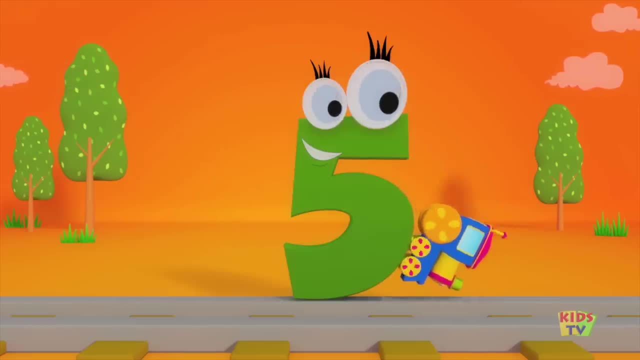 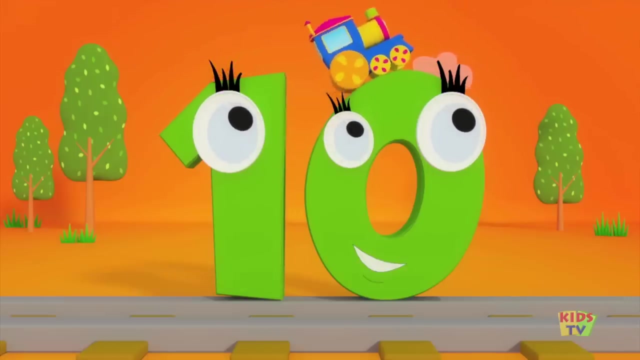 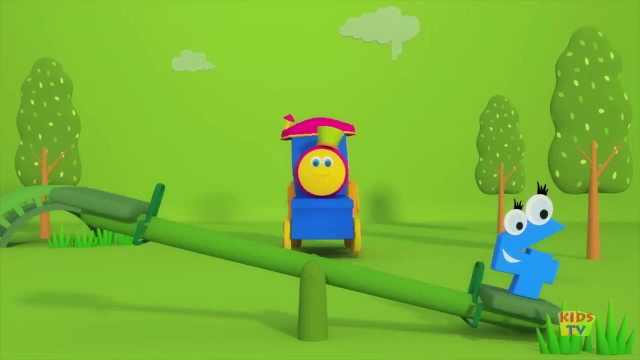 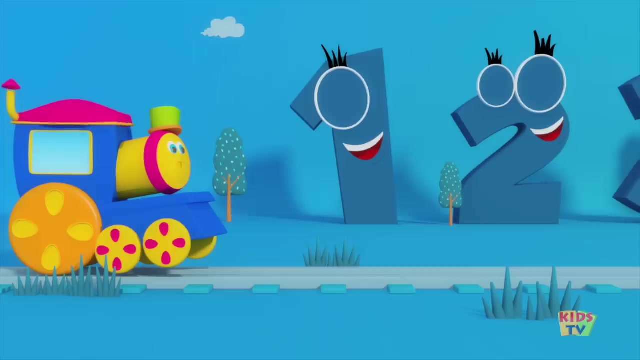 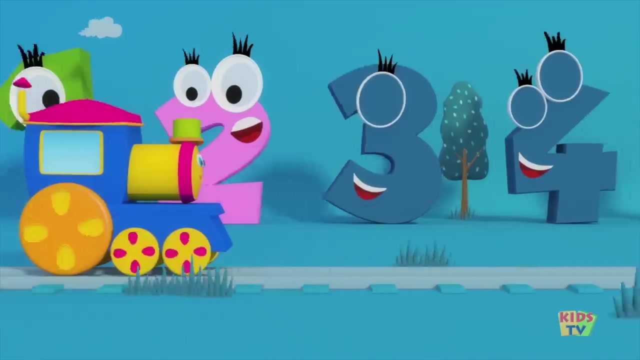 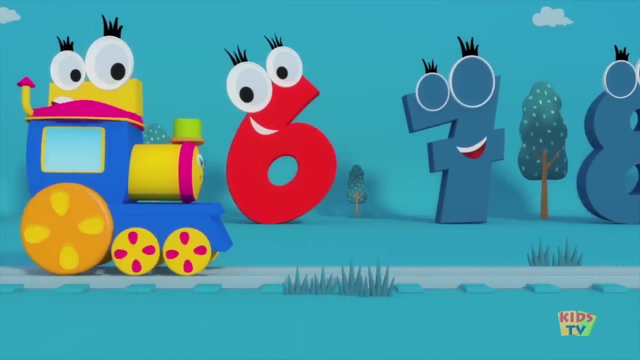 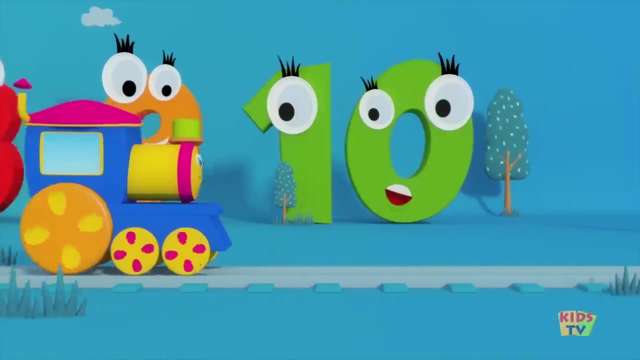 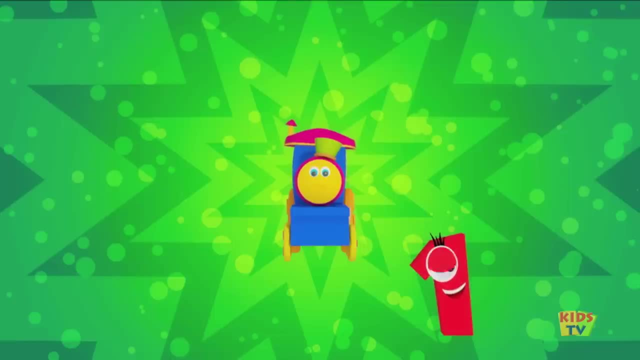 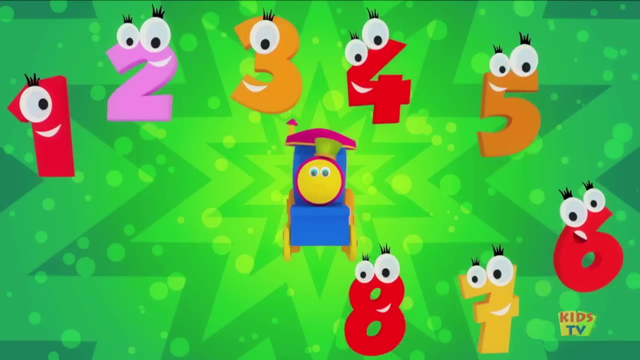 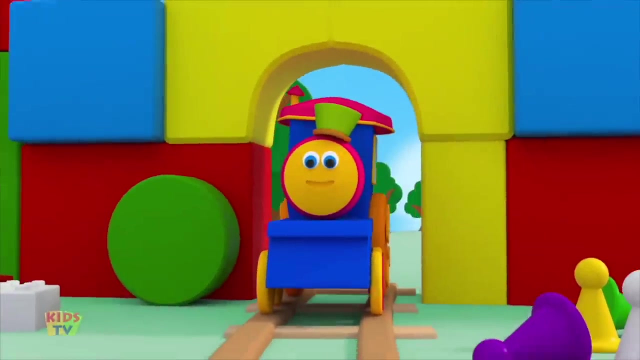 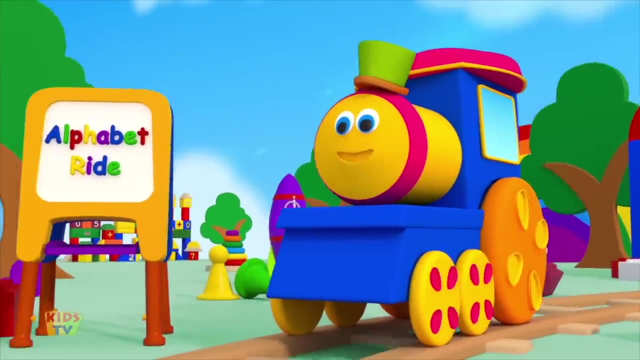 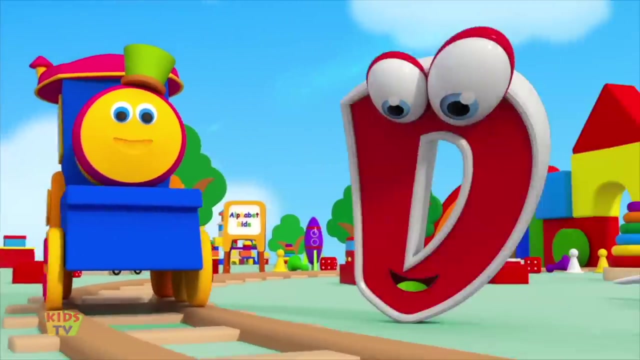 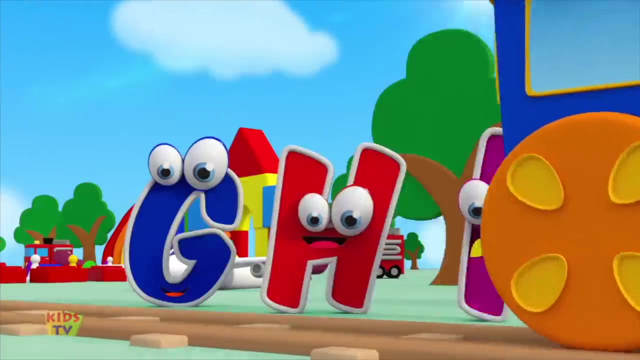 I love to play with numbers. Come with me, sing with me And dance to the number song. Did you enjoy that? Come back soon to play with Bob the Train. Wanna go on an alphabet ride with me: A, B, C and D, E, F, G, H, I. 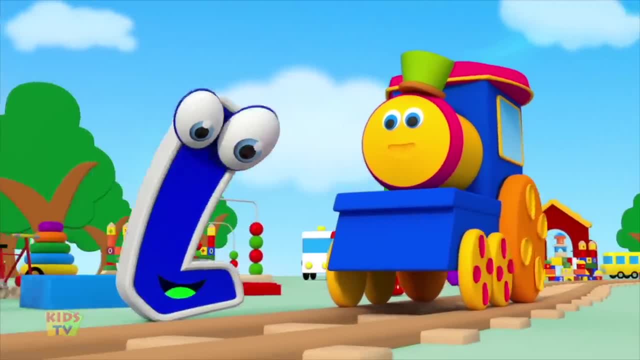 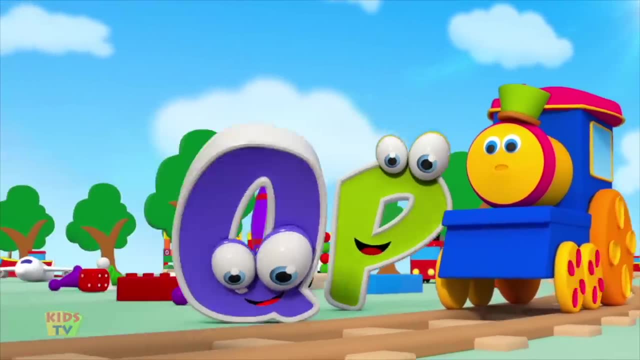 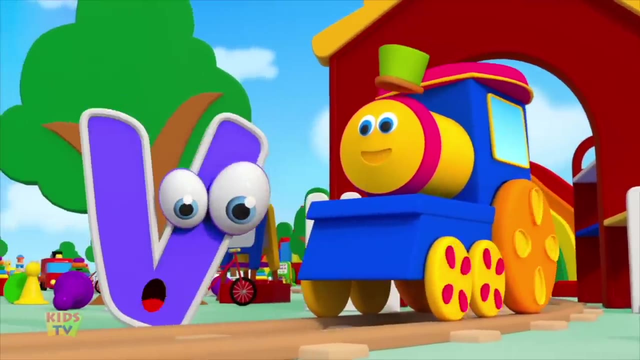 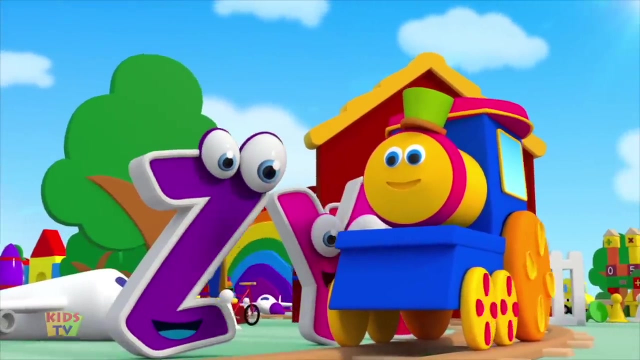 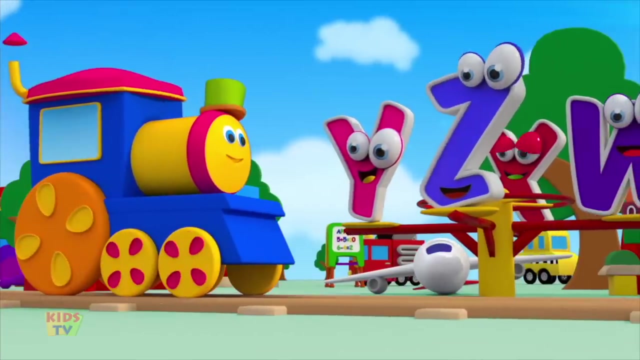 J K L and M N O V U R S T, Z, U and V, W, X and Y and Z. Wasn't that fun. Let's start from Z this time. Z and Y and X and W. 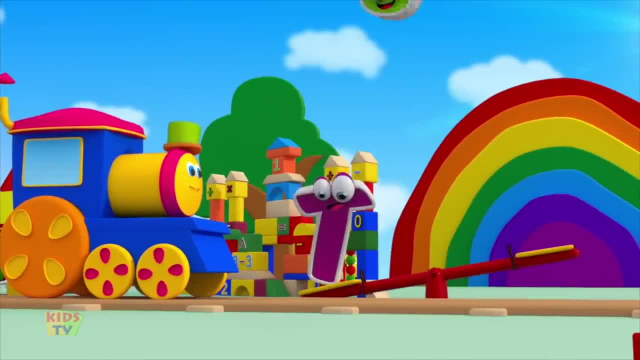 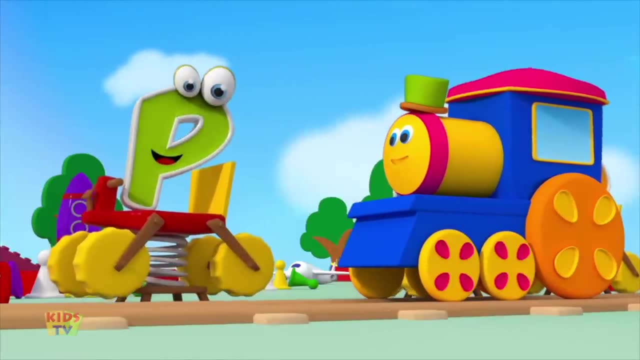 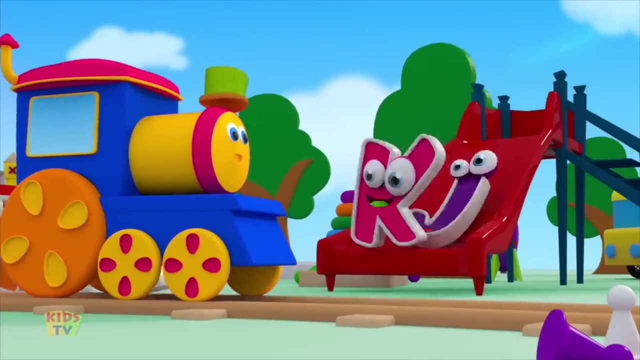 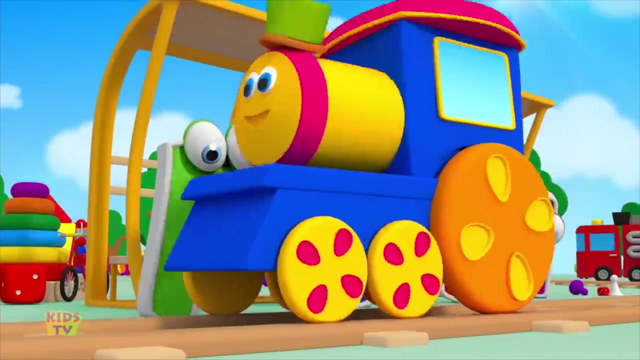 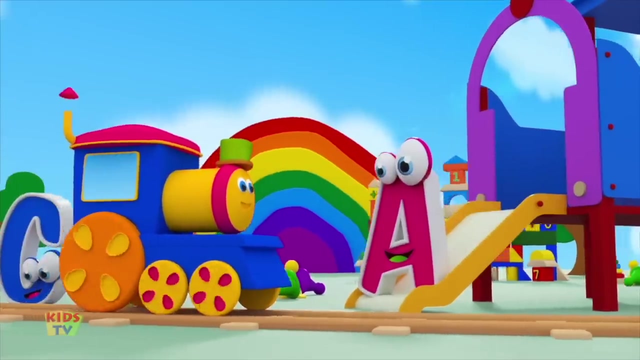 V and U and T and S, R, R and Q and P and O, N and M and L, K, J, I and H and G and F, E, D, C and B and A. One more time, starting from A. Let's all sing together. now. 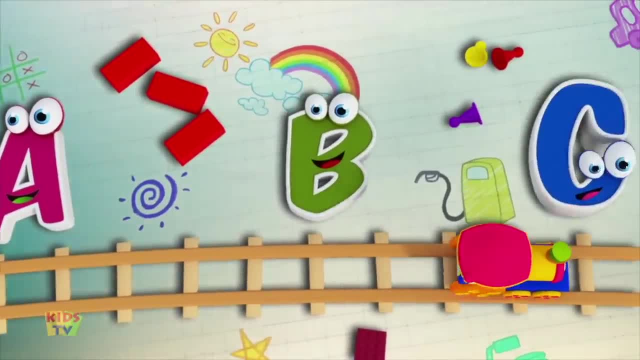 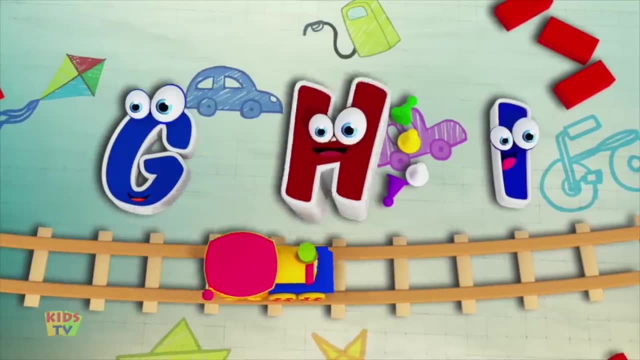 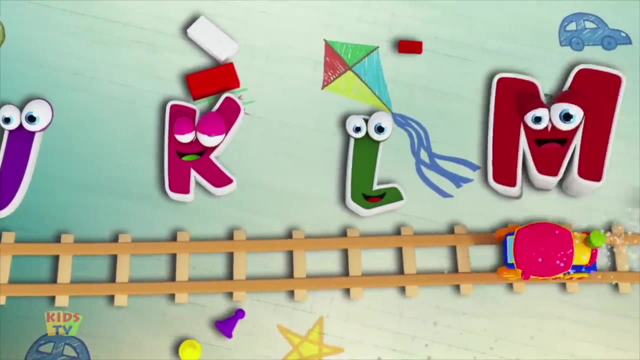 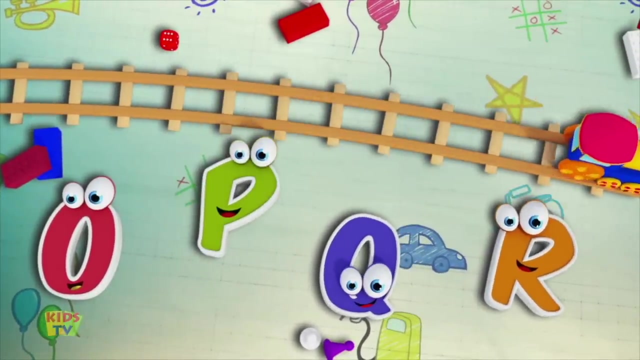 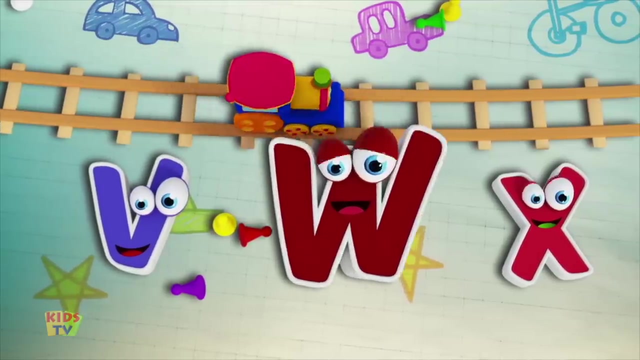 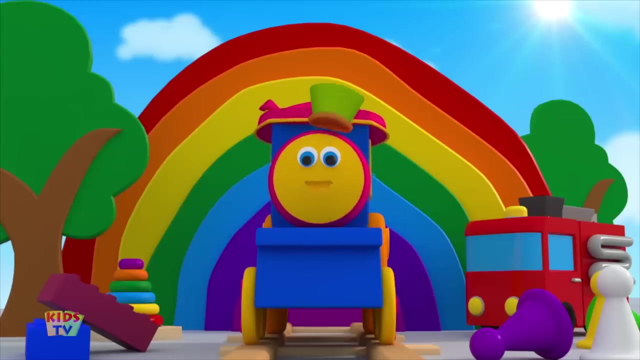 A and B and C and D, E and F and G, H, I, J and K and L and M, N and O and E, U, R, S and T and U and V, V, W, X and Y and Z. Did you enjoy the alphabet with Bob the train? 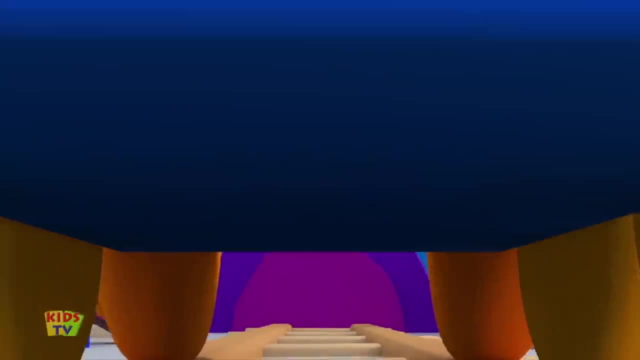 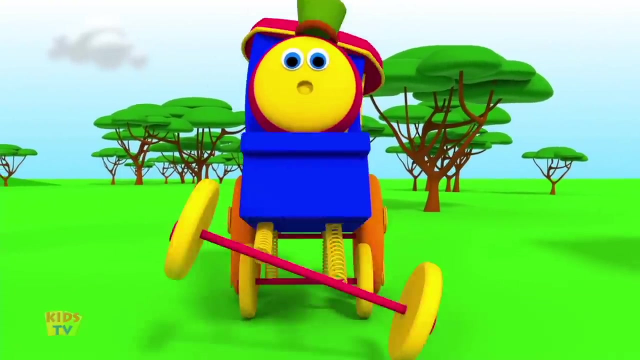 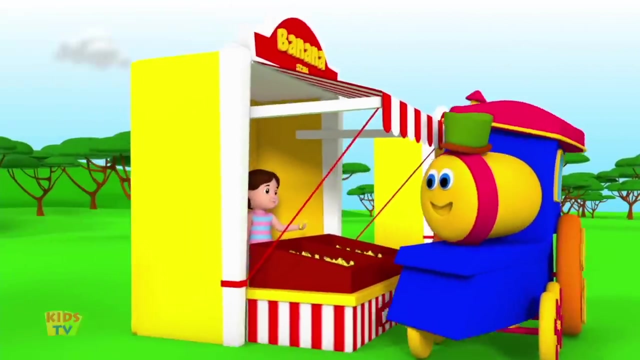 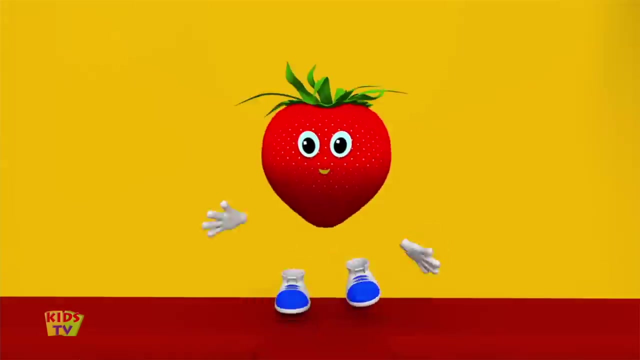 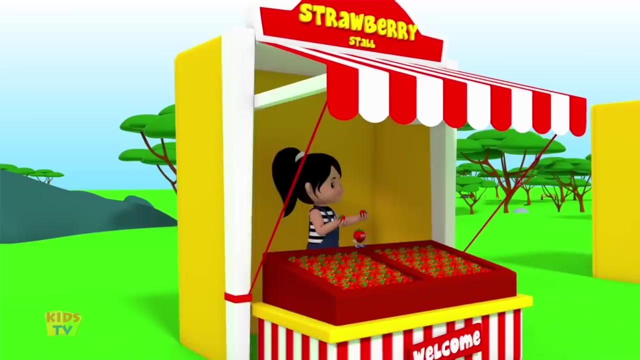 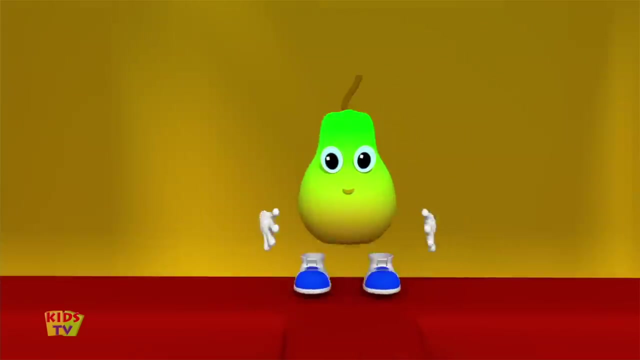 See you again next time. Hey kids, Welcome to Bob's learning street. Let's go meet the fruits today. Fruits, fruits, fruits. You just can't dispute Their positive attributes, Even in their birthday suits. Fruits, fruits, fruits, You just can't dispute. 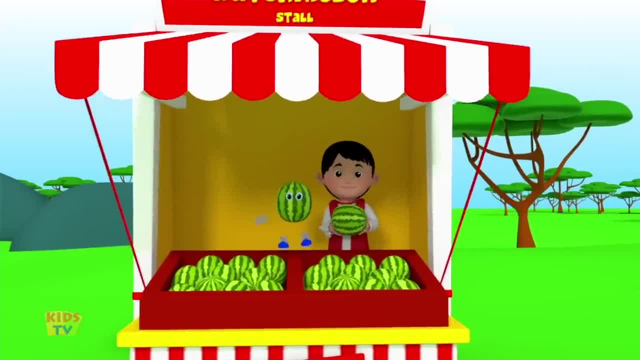 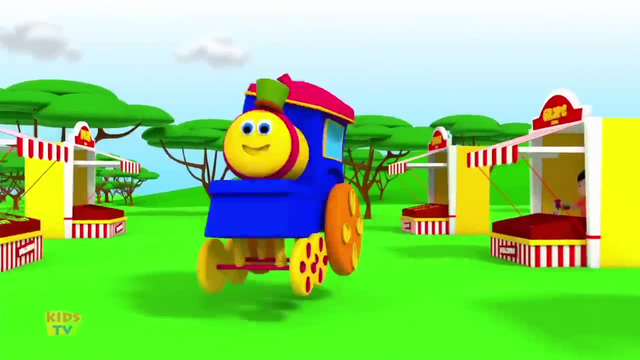 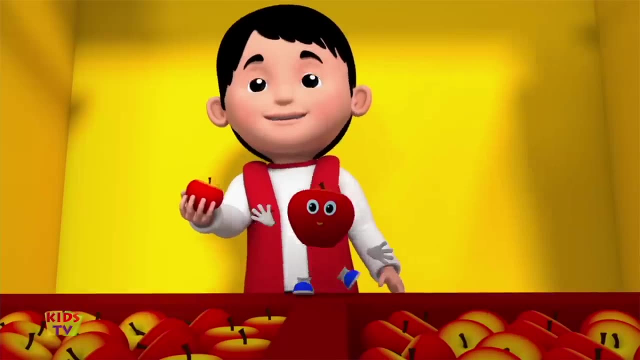 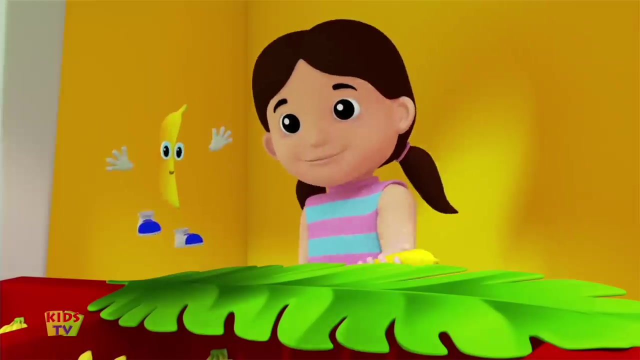 Their positive attributes Even in their birthday suits. You can have an apple Every single day. Cause: an apple a day Keeps the doctor away. The doctor away, Mr Yellow Banana. He loves to play piano. He can spell his name, we hope, But he never knows when to stop. 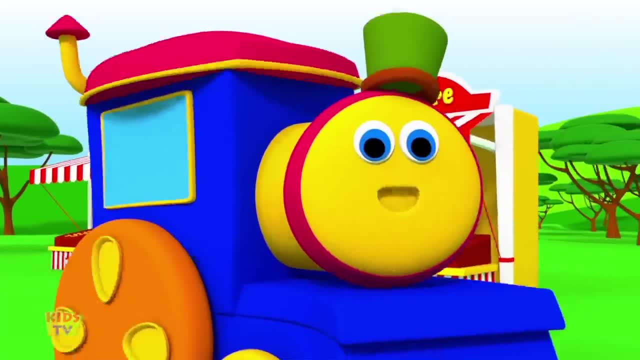 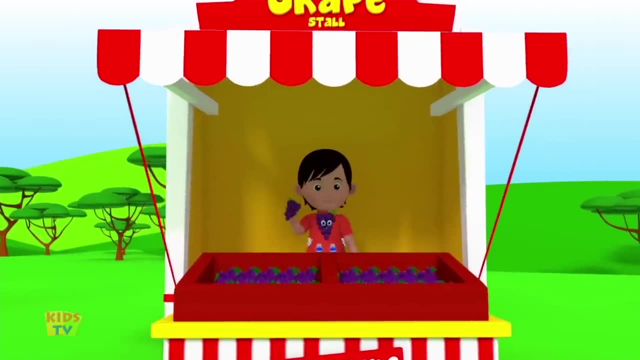 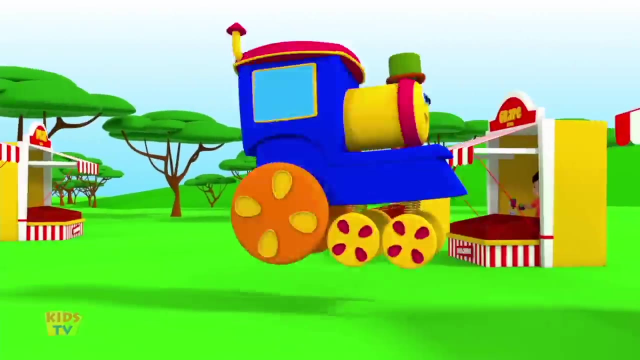 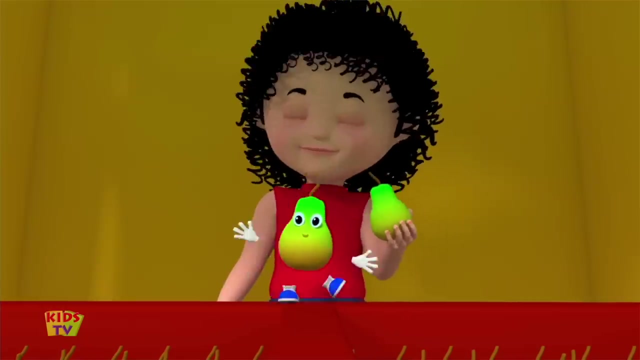 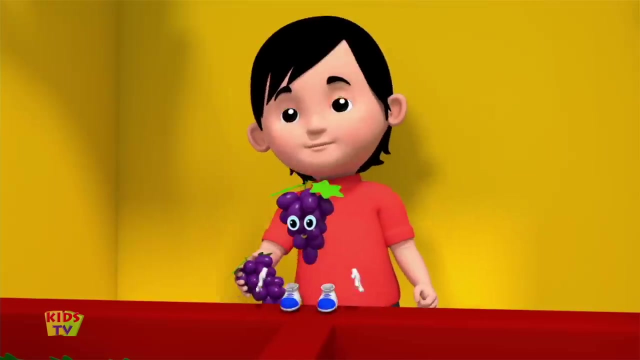 Fruits, fruits, fruits. You just can't dispute The positive attributes, Even in their birthday suits. Look at Mr Pear, He's beyond. compare Hanging in mid-air. If you eat him, please share, Please share These sweet little grapes. A bunch of oval shapes Brightening up landscapes. 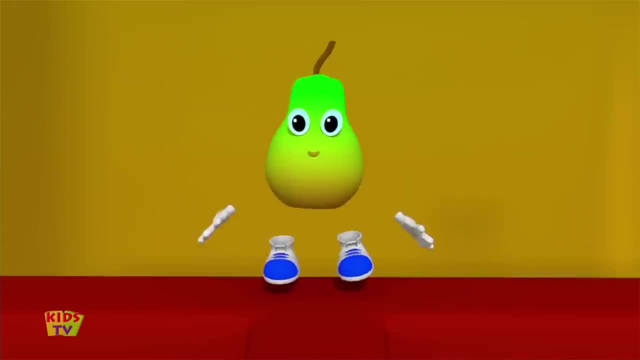 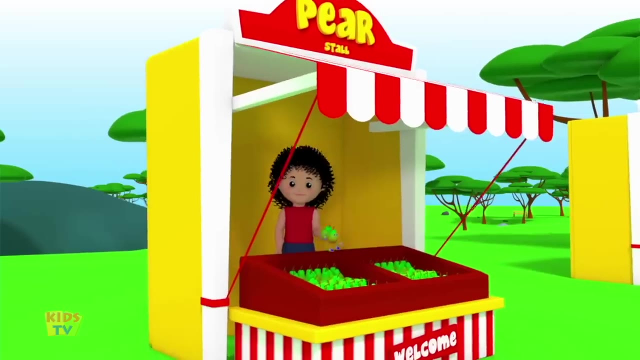 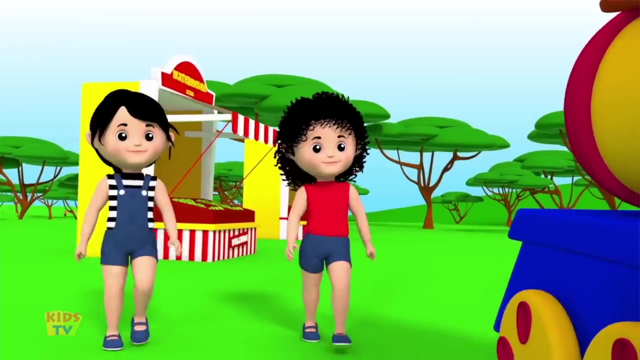 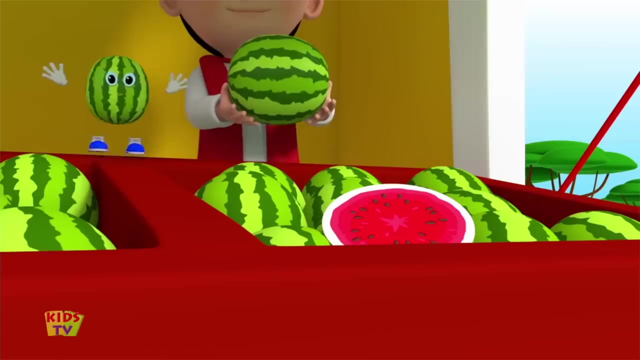 They're a juicy escape. Fruits, fruits, fruits. You just can't dispute Their positive attributes, Even in their birthday suits. Mr Watermelon, Don't confuse me with a lemon. You're green out, red Inside and striped Just like a felon. Just like a felon. 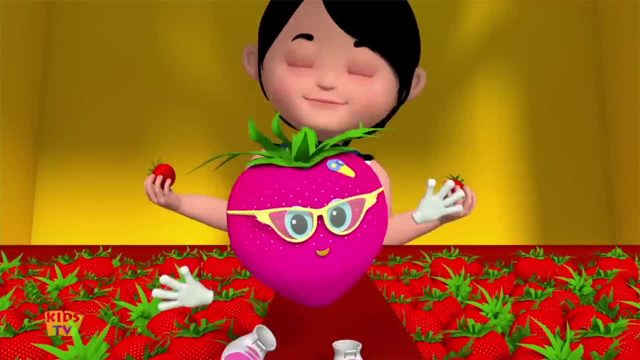 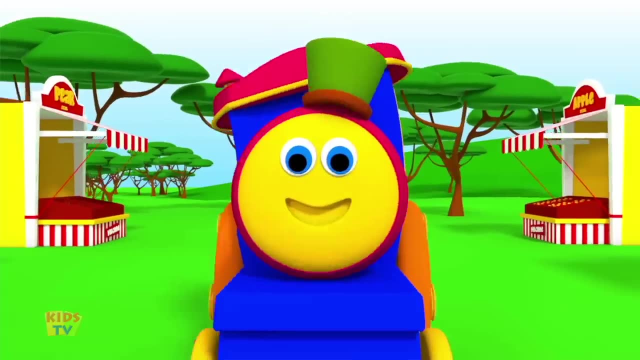 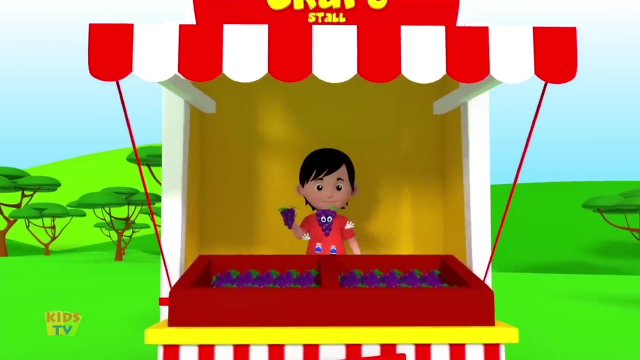 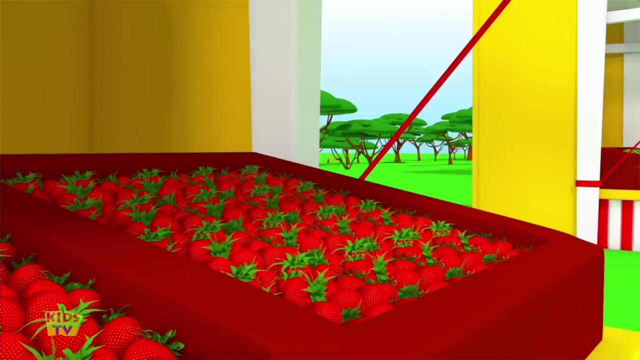 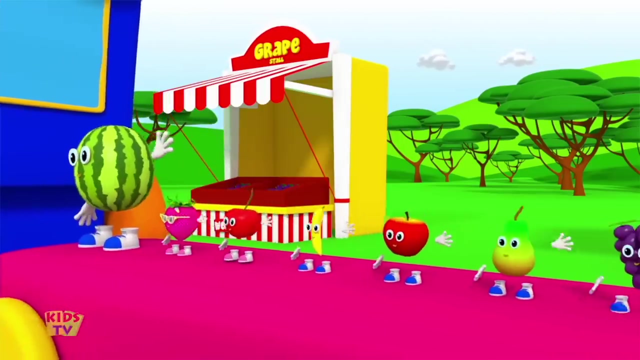 Pretty Miss Strawberry. You always look so merry With your friends, the little cherries. Why don't you both marry Fruits, fruits, fruits. You just can't dispute Their positive attributes, Even in their birthday suits. They'll always be Popular, popular and fun. I know a merry little song. 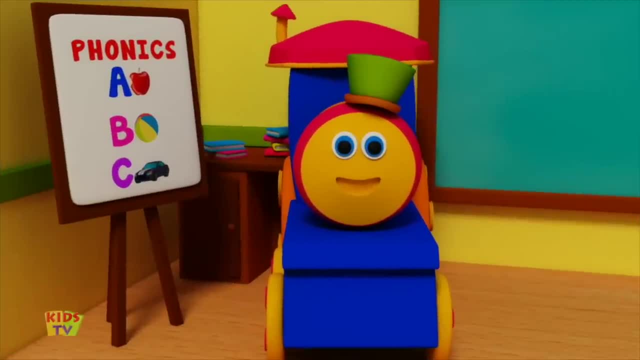 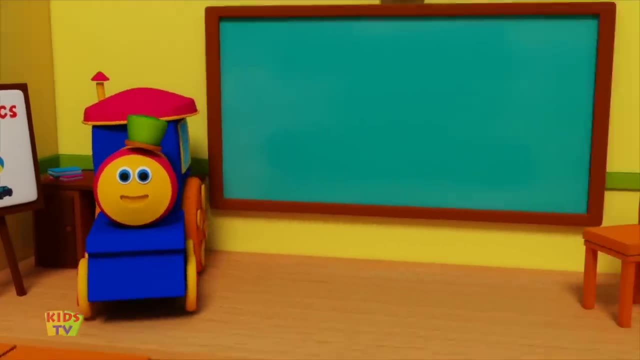 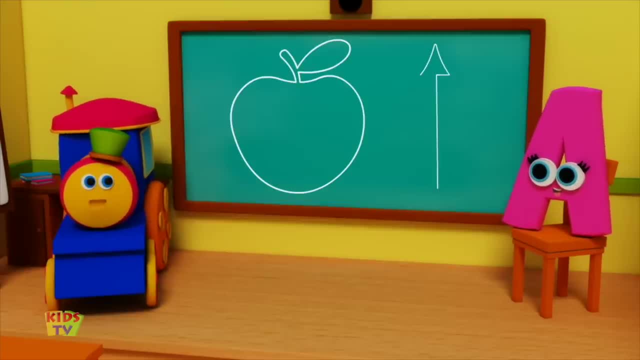 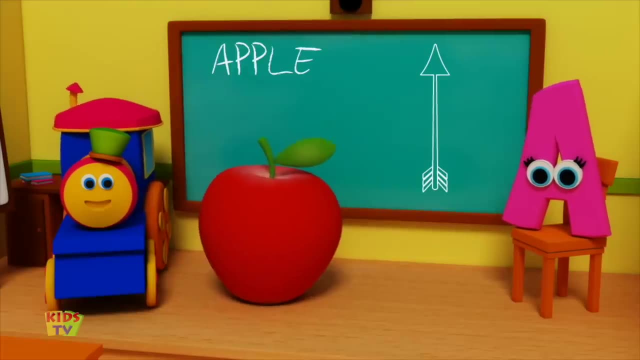 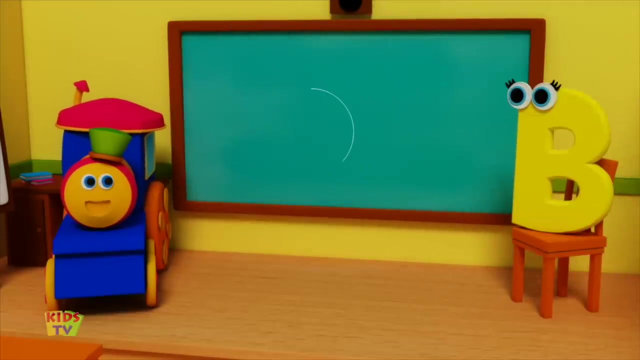 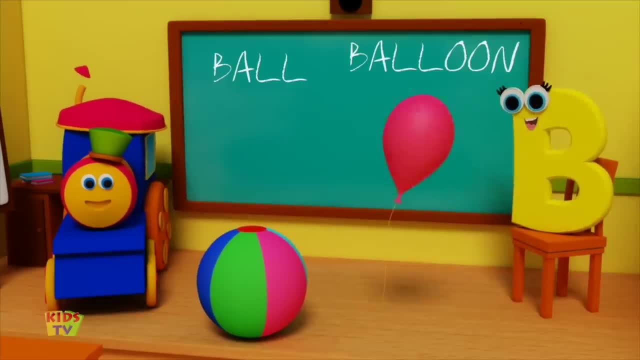 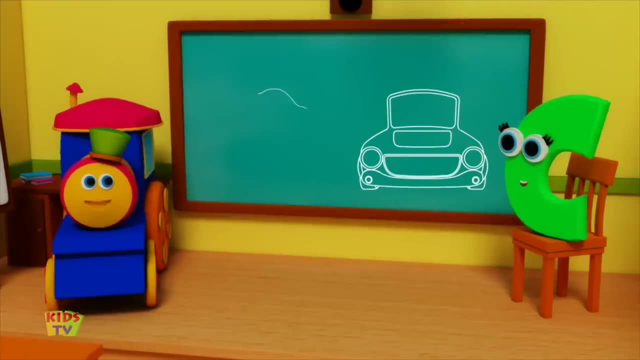 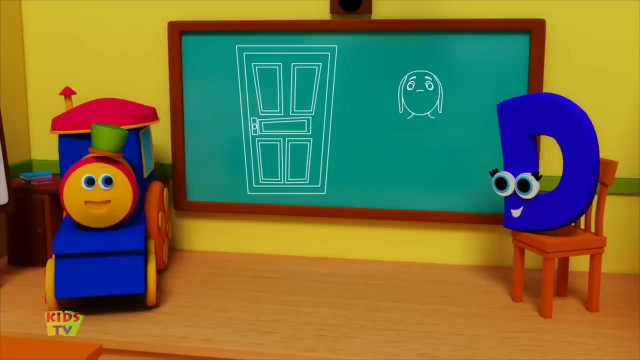 B is for b-b-b-balloon, C is for car c-c-car, C is for cloud c-c-cloud, C is for c-c-c-cloud, C is for c-c-c-car, D is for door d-d-door, D is for dog d-d-dog, D is for d-d-d-d-door. 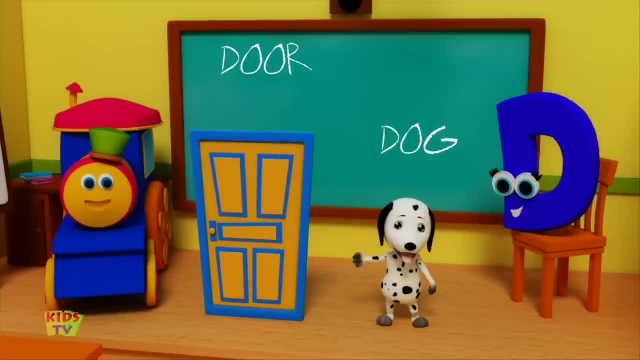 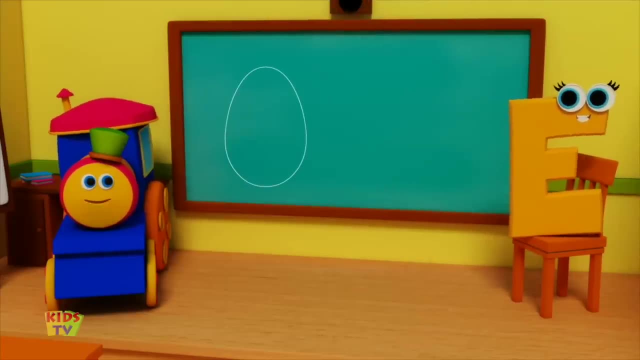 D is for d-d-d-d-dog, E is for eggs e-e-eggs. E is for earth e-e-earth, E is for a-a-a-a-eggs, E is for a-a-a-a-earth, F is for fan f-f-fan. 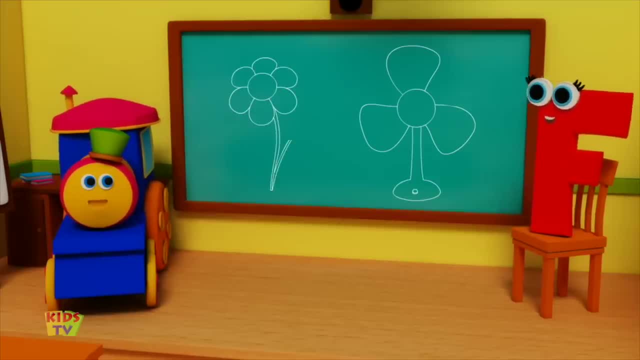 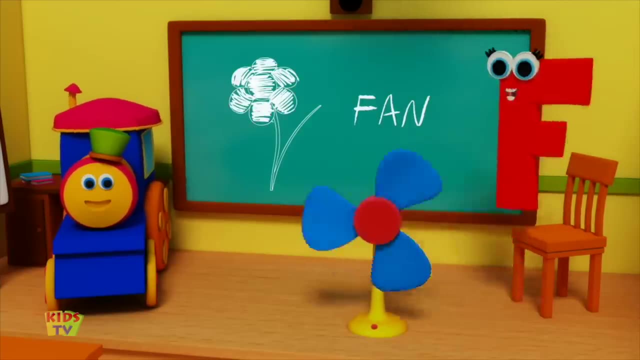 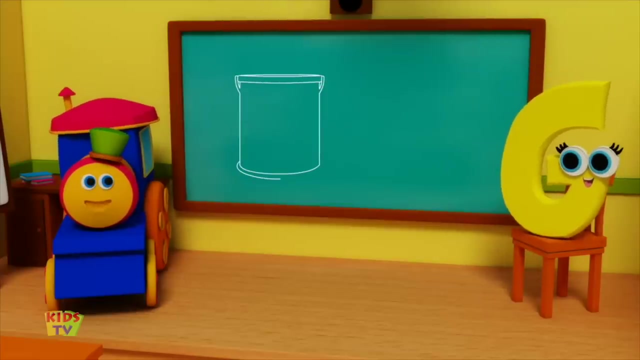 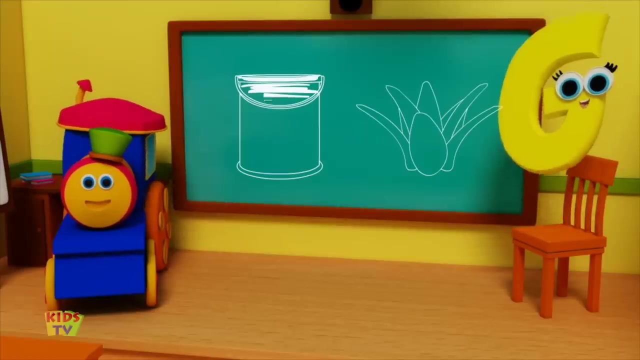 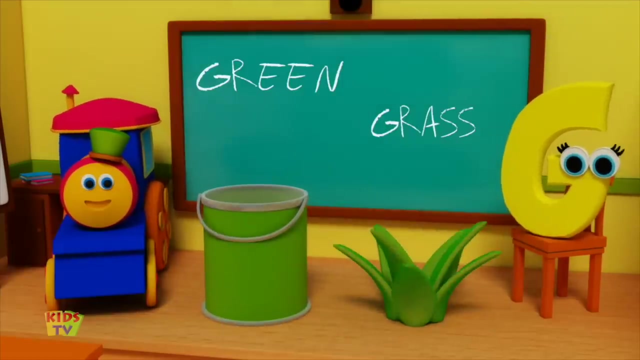 F is for flower, f-f-flower, F is for f-f-f-fan, F is for f-f-f-flower, G is for green: g-g-green. G is for grass: g-g-grass, G is for g-g-g-green, G is for g-g-g-grass, H is for heart: h-h-heart. 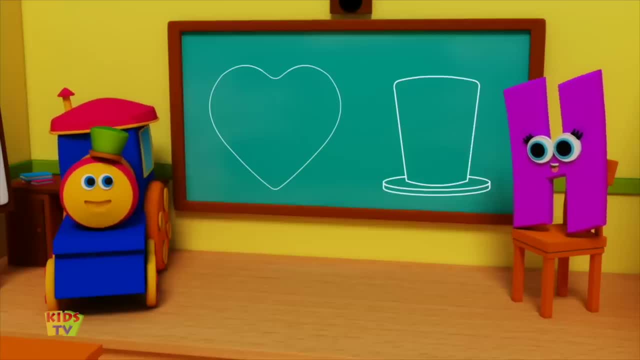 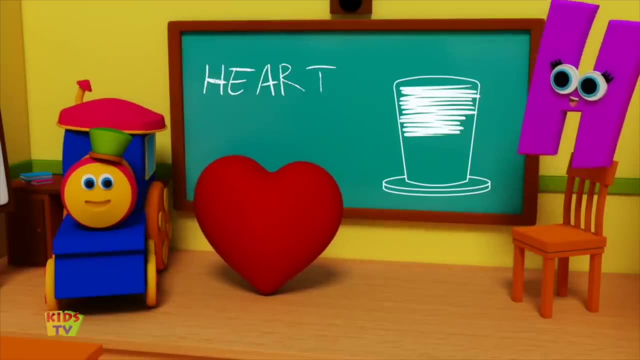 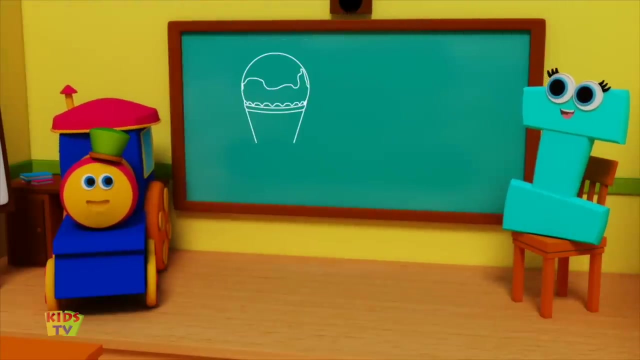 H is for hat h-h-hat, H is for h-h-h-heart, H is for h-h-h-hat. I is for ice cream, i-i-ice cream. I is for iron- i-i-iron. I is for i-i-i-ice cream. 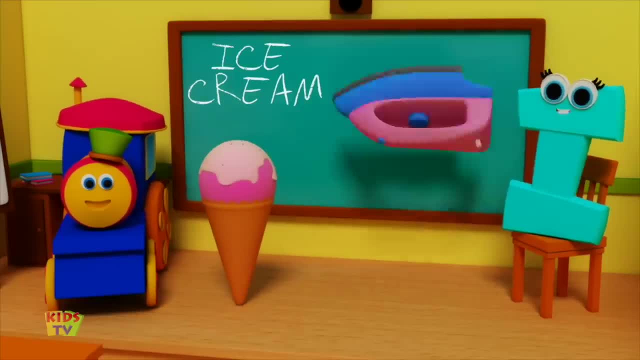 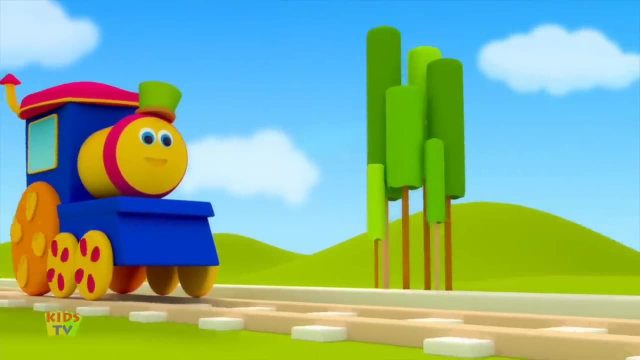 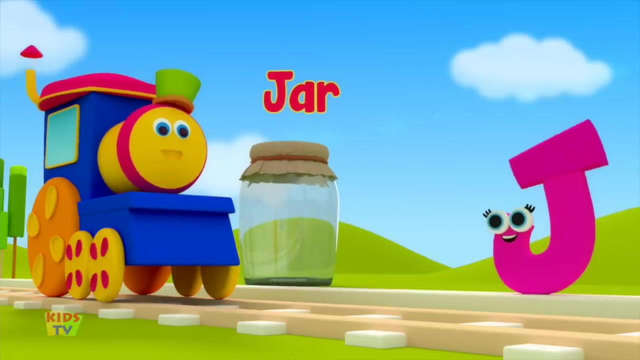 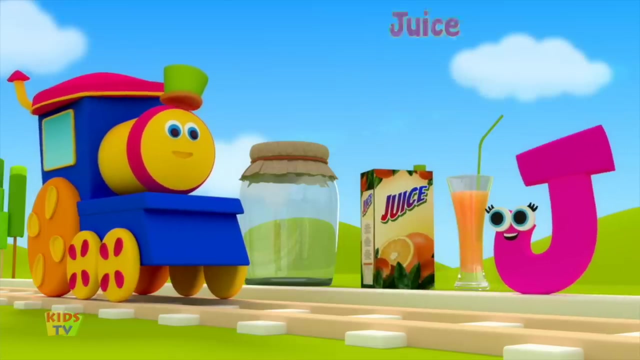 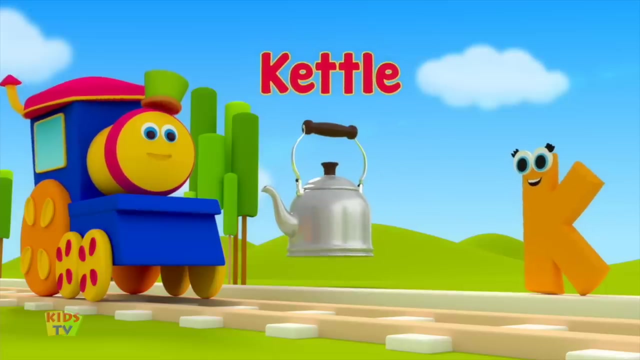 I is for i-i-i-iron. J is for jar- j-j-jar. J is for juice- j-j-juice. J is for j-j-j-jar, J is for j-j-juice, K is for kettle- k-k-kettle. K is for key- k-k-key. 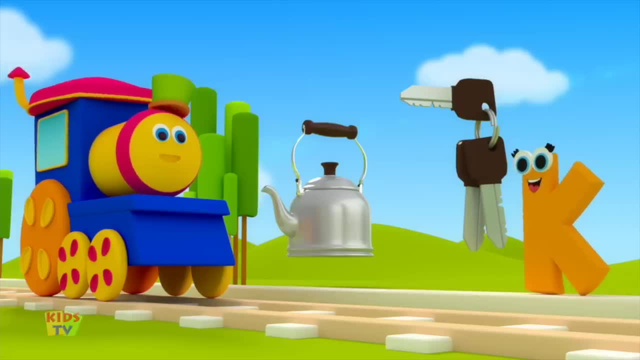 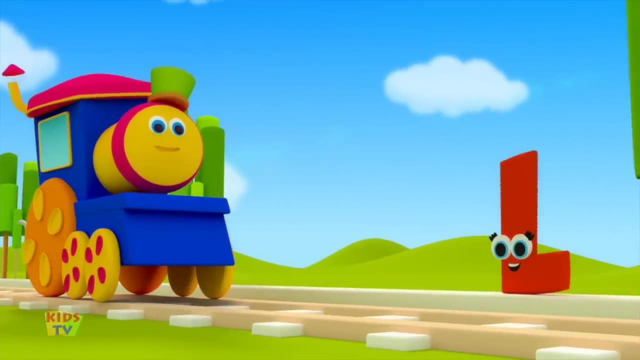 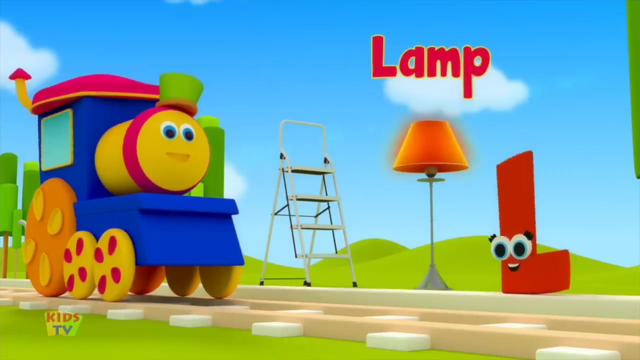 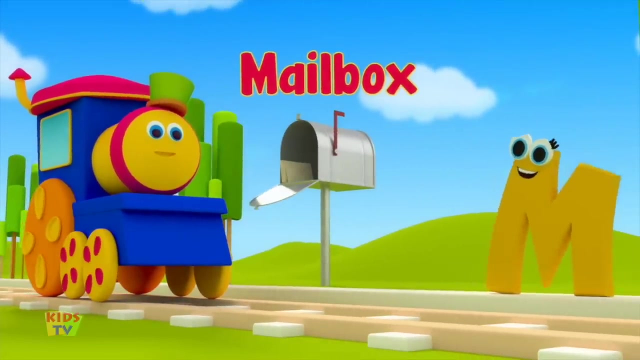 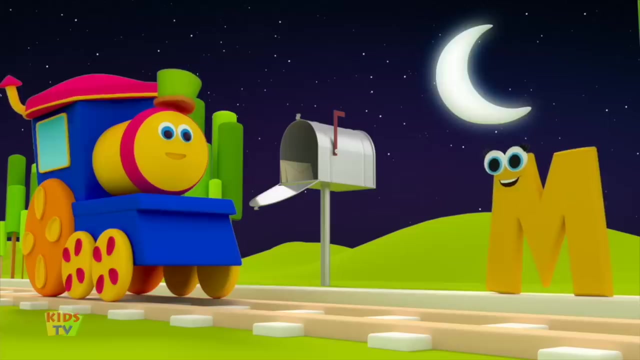 K is for k-k-k-kettle, K is for k-k-k-key, L is for ladder, l-l-ladder, L is for lamp- l-l-lamp, L is for l-l-l-ladder, L is for l-l-l-lamp, M is for mailbox: m-m-mailbox. M is for moon: m-m-moon. 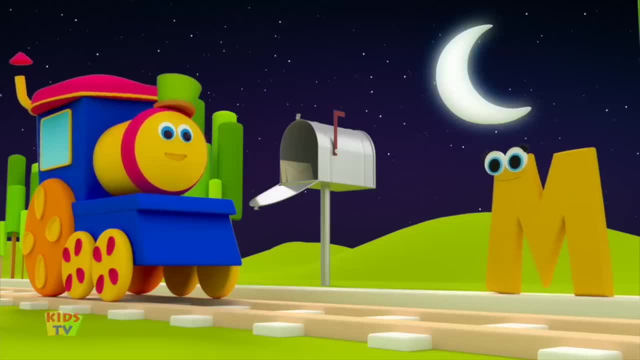 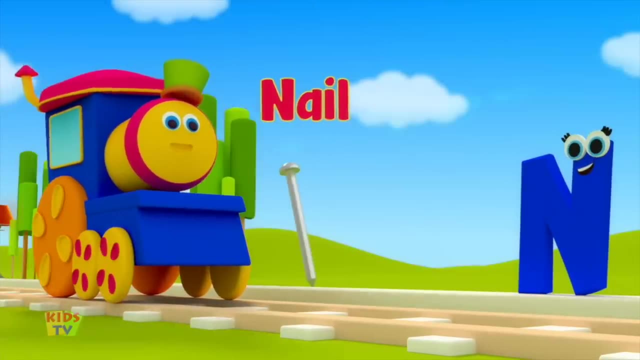 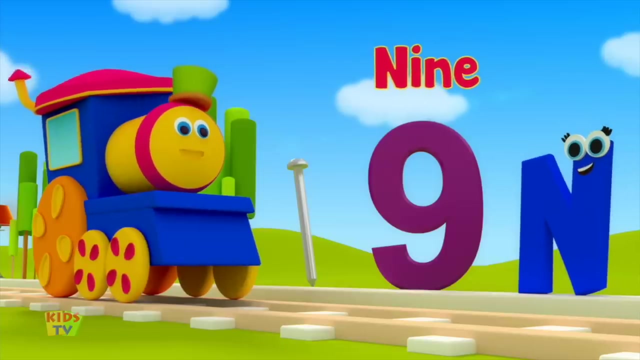 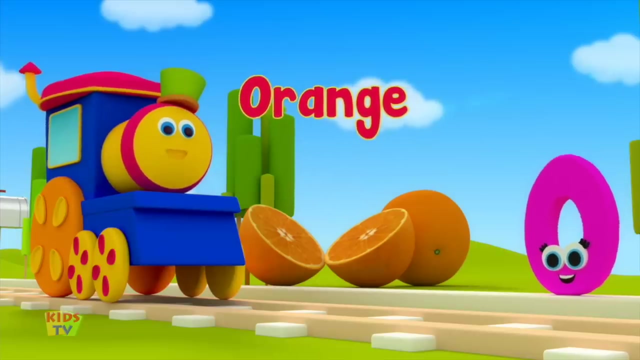 M is for m-m-m-mailbox, M is for m-m-m-moon, N is for nail n-n-nail. N is for nine- n-n-nine, N is for n-n-n-nail, N is for n-n-n-nine, O is for orange- o-o-orange, O is for oval- o-o-oval. 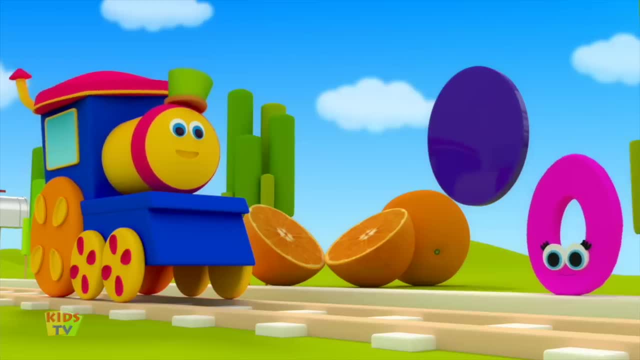 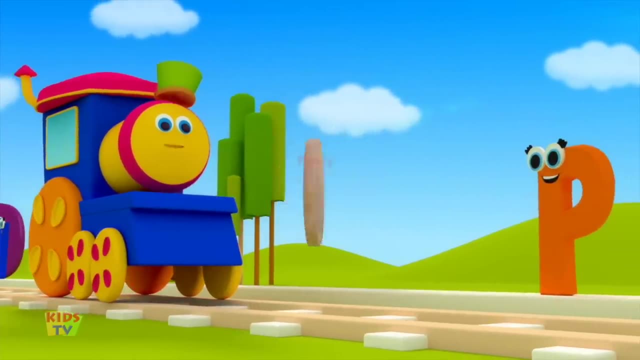 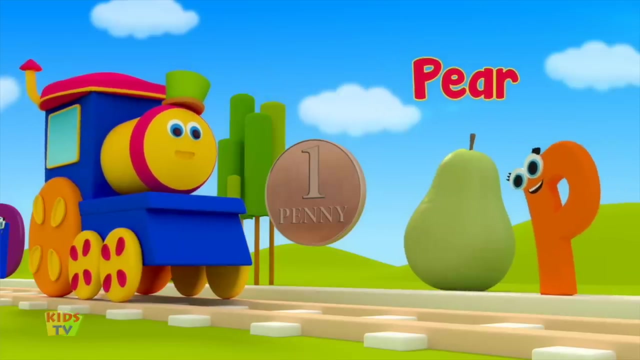 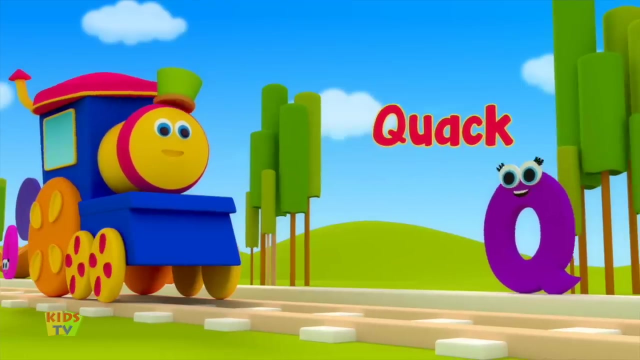 O is for o-o-o-orange, O is for o-o-o-oval, P is for penny p-p-penny, P is for pear p-p-pear, P is for p-p-p-penny, P is for p-p-p-pear, Q is for quack q-q-quack, Q is for question mark- q-q-question mark. 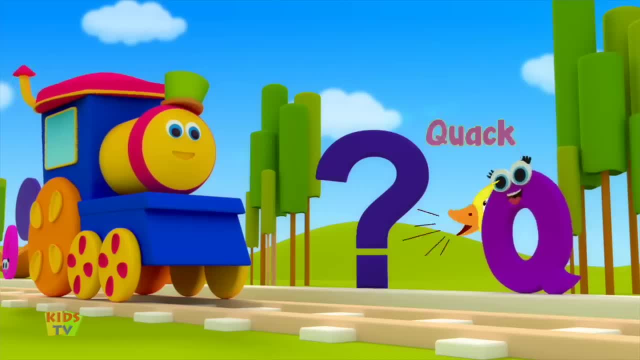 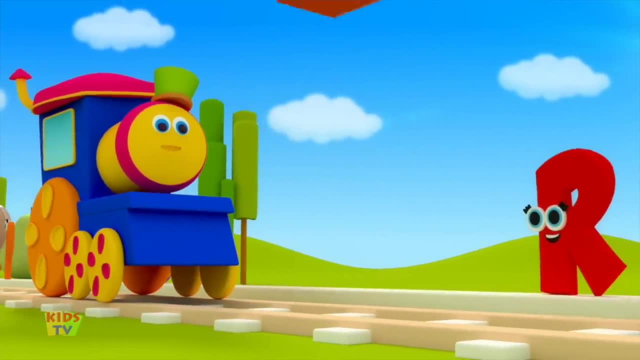 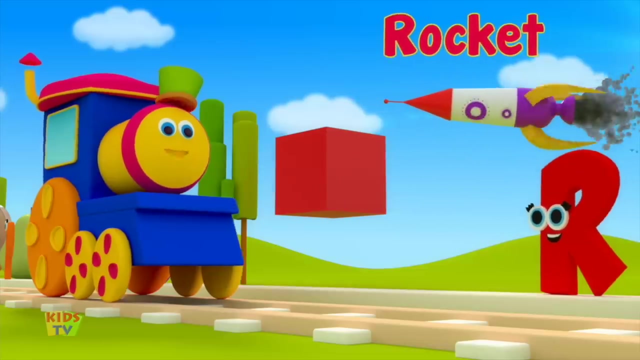 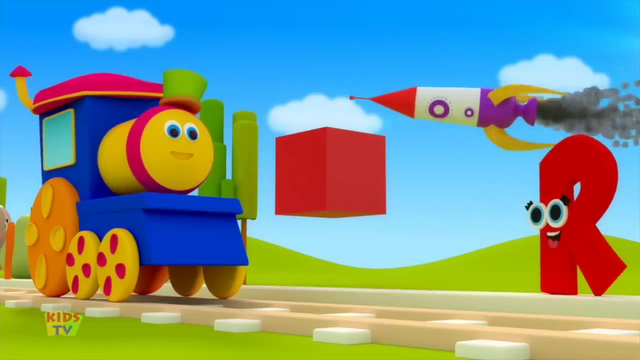 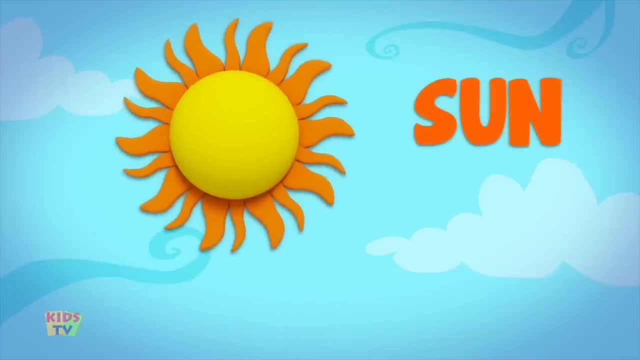 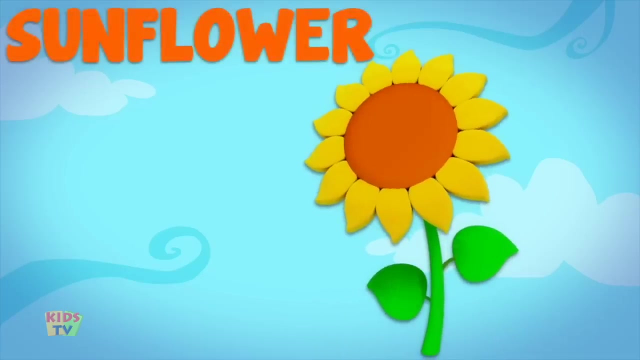 Q is for q-q-q-q-quack, Q is for q-q-q-q-question mark. R is for red r-r-red, R is for rocket r-r-rocket, R is for r-r-r-red, R is for r-r-r-rocket, S is for sun s-s-sun, S is for sunflower s-s-sunflower. 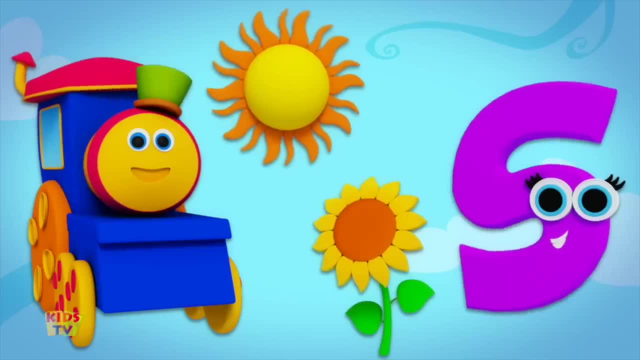 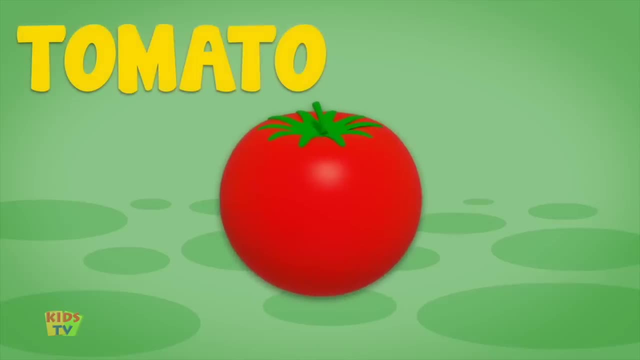 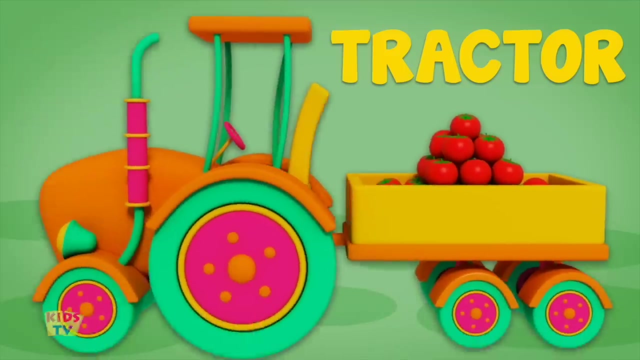 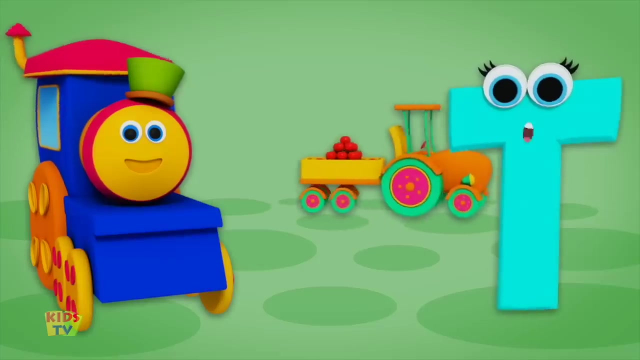 S is for s-s-s-sun, S is for s-s-s-sunflower, T is for tomato- t-t-tomato, T is for tractor t-t-tractor, T is for t-t-t-t-tomato, T is for t-t-t-t-tractor. 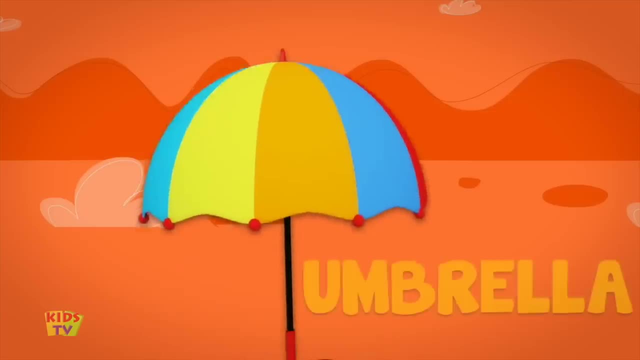 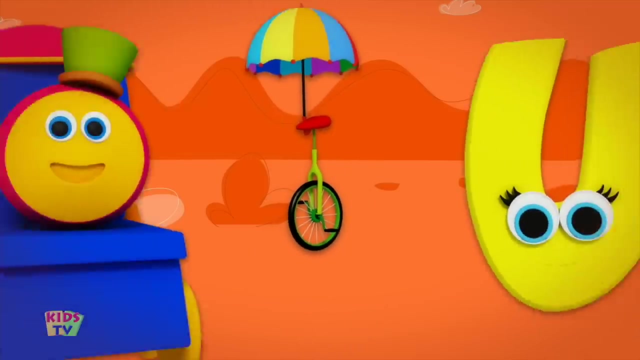 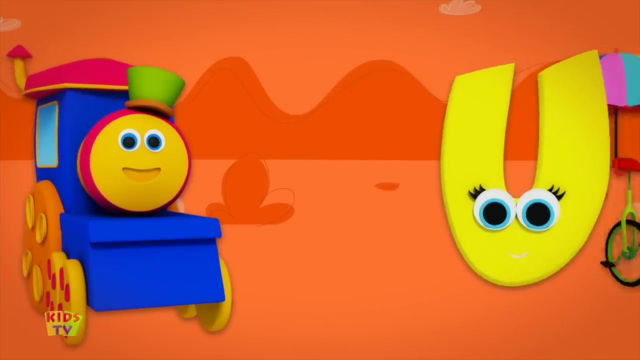 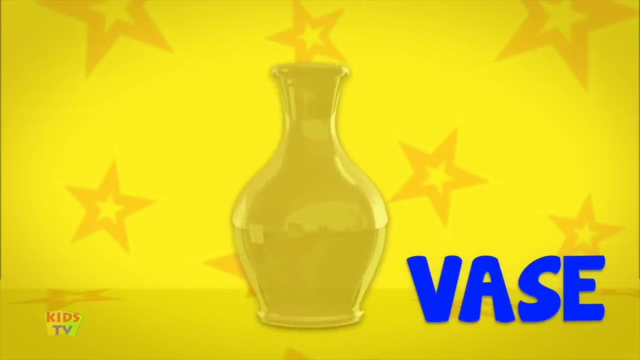 U is for umbrella, u-u-umbrella, U is for unicycle u-u-unicycle. U is for U? U U U U. Umbrella U is for U U U U, Unicycle. V is for Vaz V V. Vaz. V is for Violet, V V, Violet. 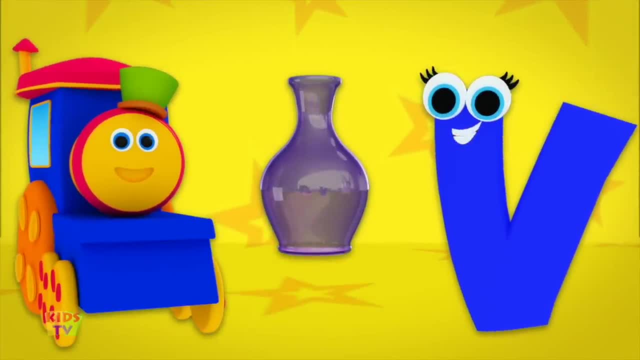 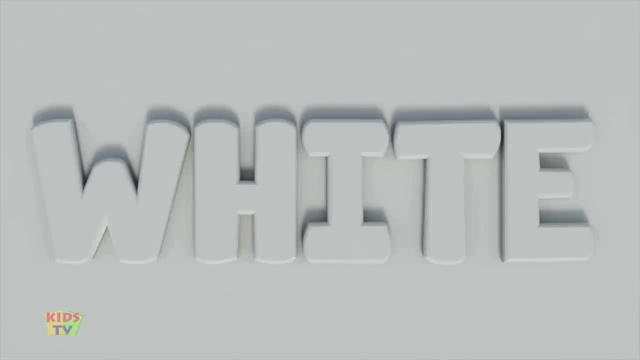 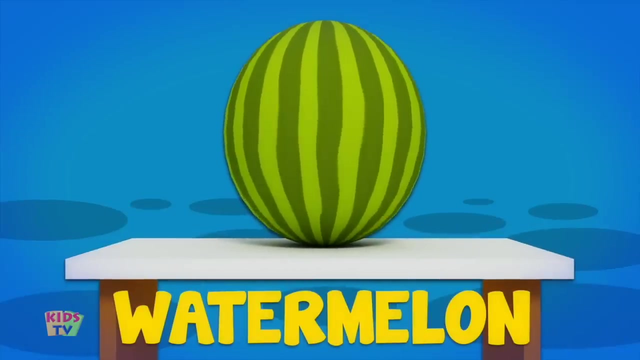 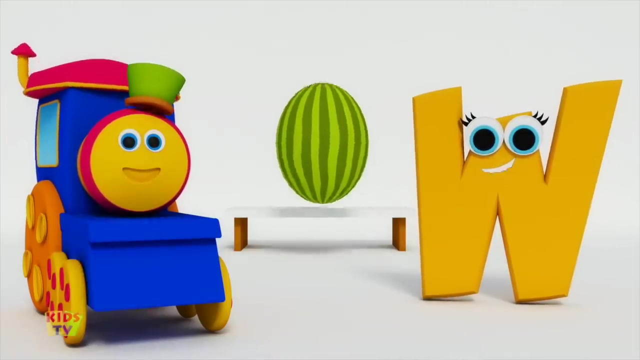 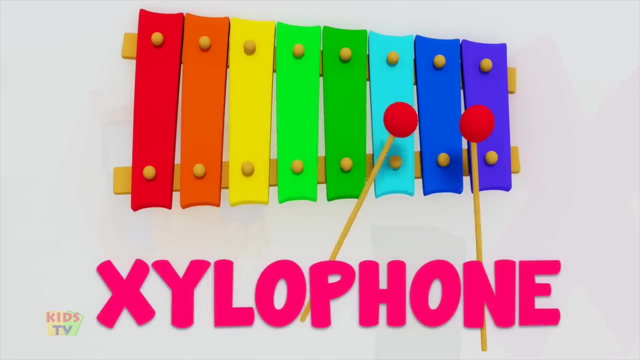 V is for V V V V. Vaz. V is for V V V V. Violet W is for white w-w-white. W is for watermelon w-w-watermelon. W is for w-w-w-white, W is for w-w-w-watermelon. X is for xylophone- z-z-xylophone. X is for x-box- x-x-x-box. 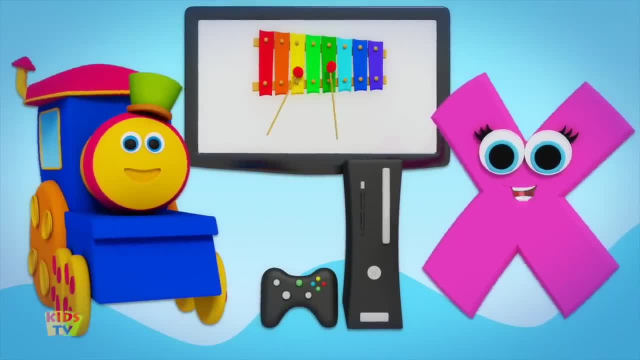 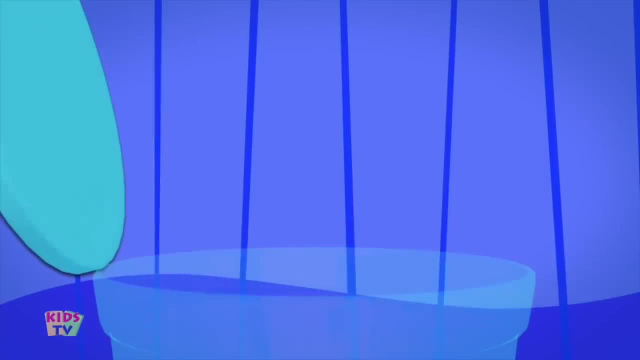 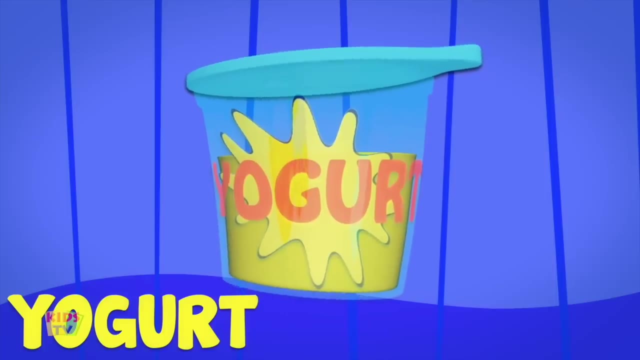 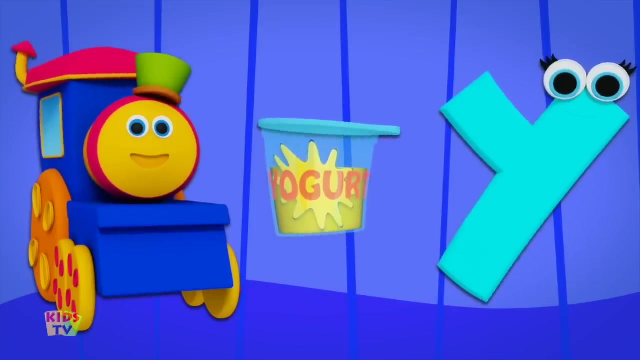 X is for z-z-z-xylophone, X is for x-x-x-x-box, Y is for yellow- y-y-yellow, Y is for yogurt- y-y-yogurt, Y is for y-y-y-yellow, Y is for y-y-y-yogurt. 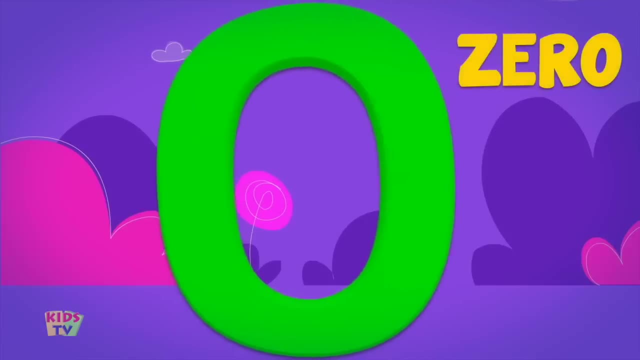 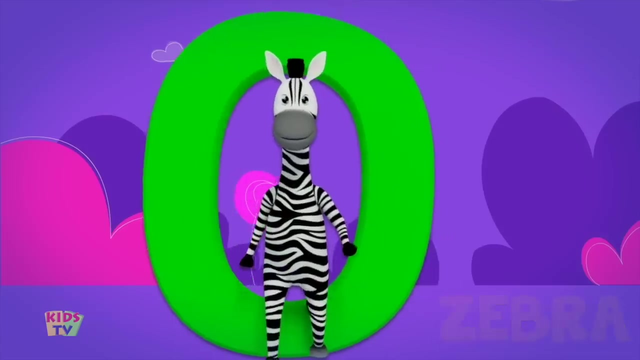 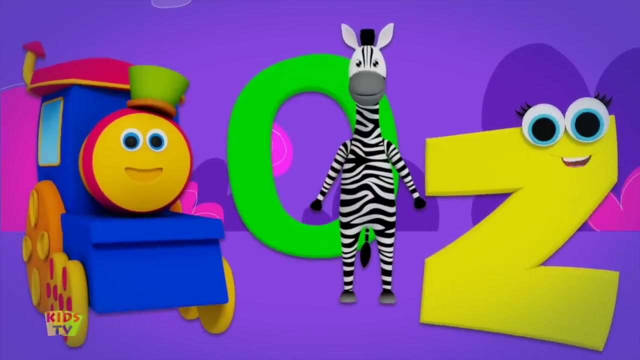 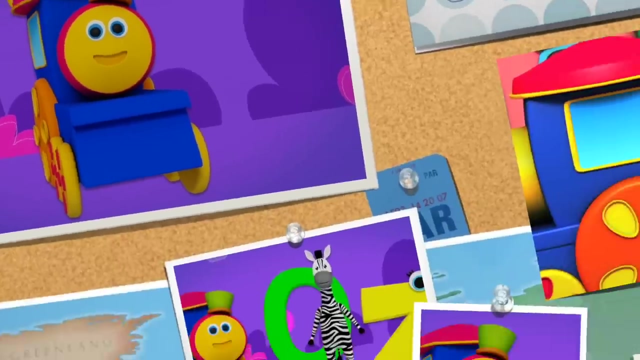 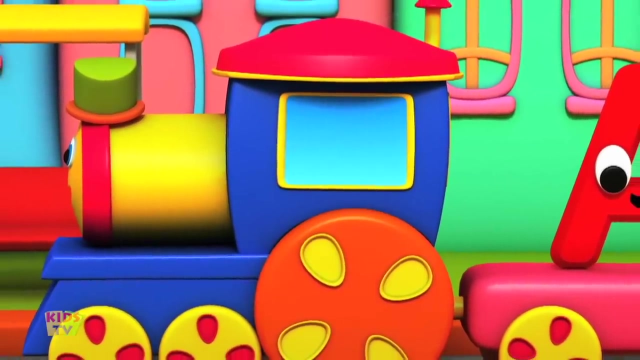 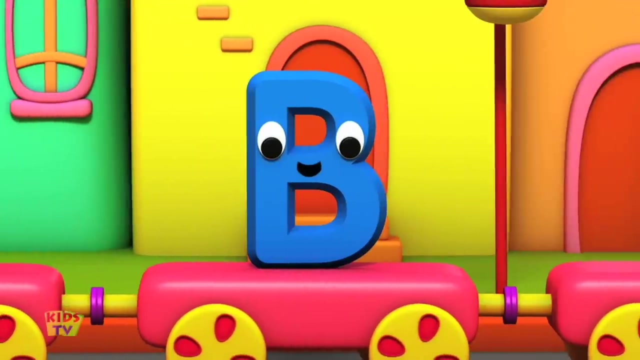 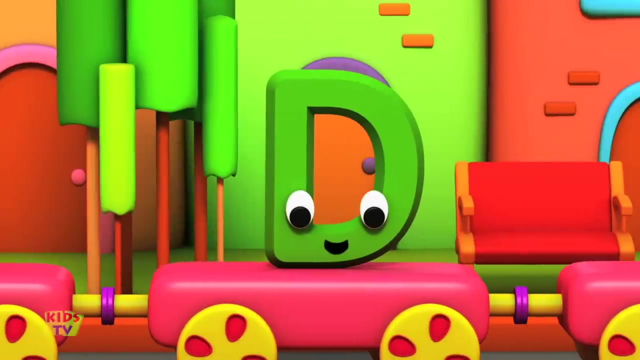 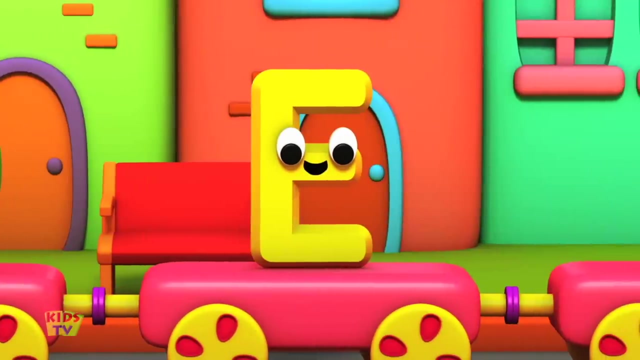 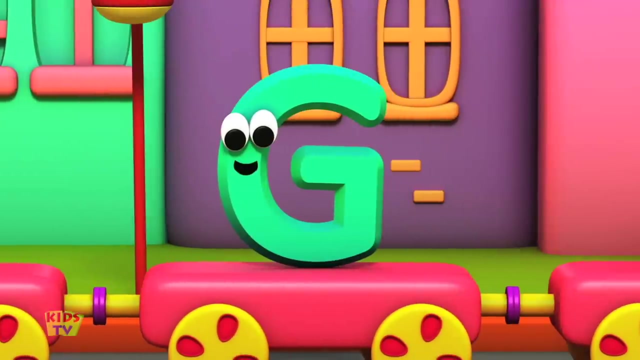 Z is for zero, Z-z-zero Z is for zebra, Z-z-zebra Z is for z-z-z-zero, Z is for z-z-z-zebra. Wasn't it fun learning the phonics? A, B, C, D, E, F, G, I. 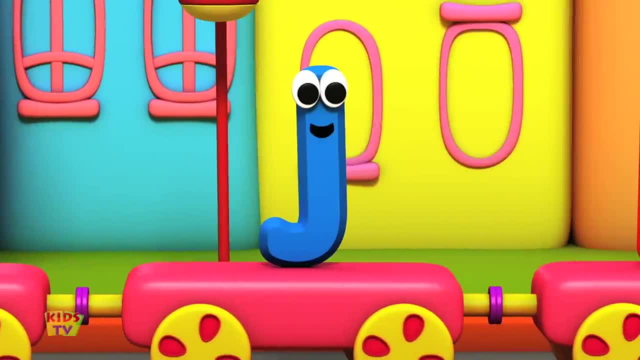 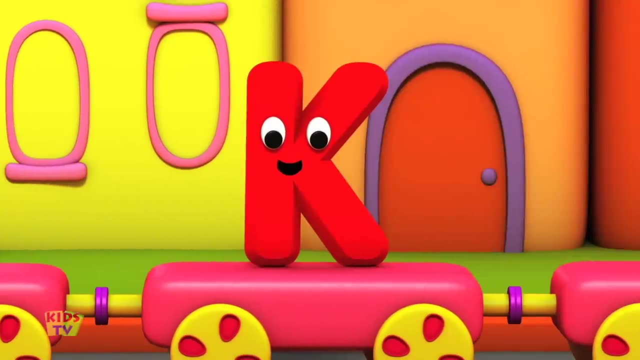 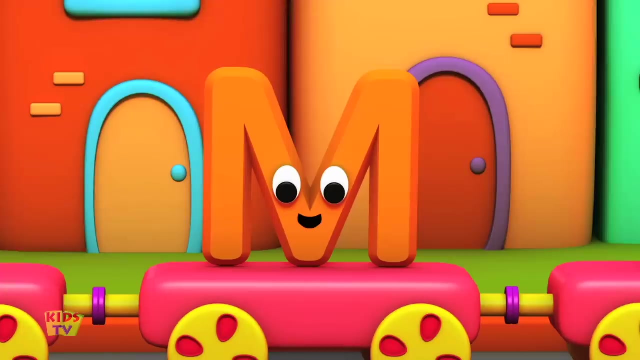 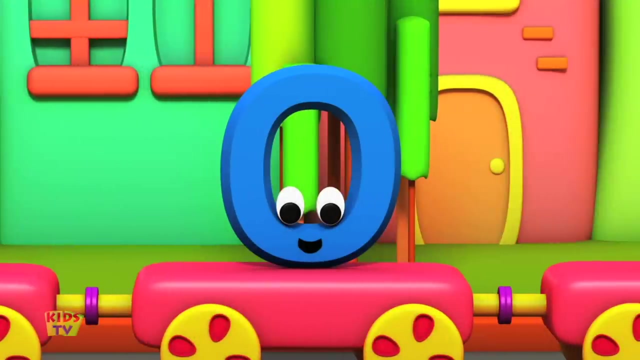 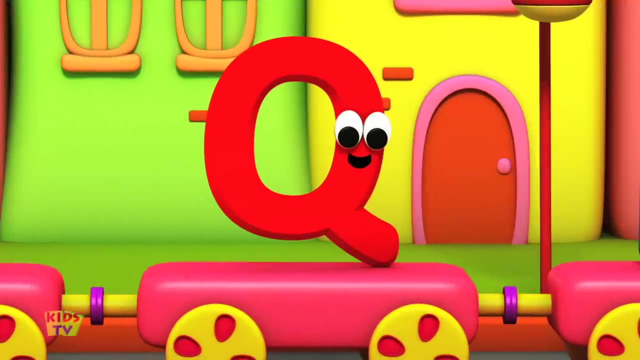 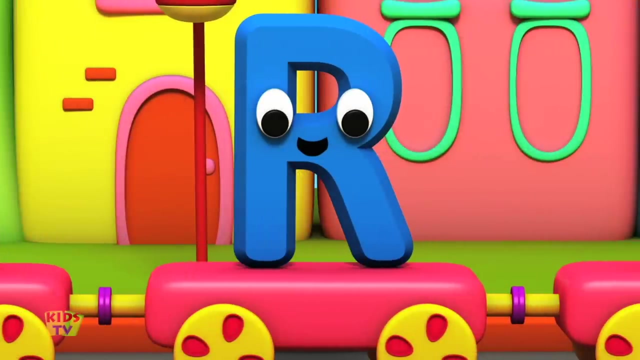 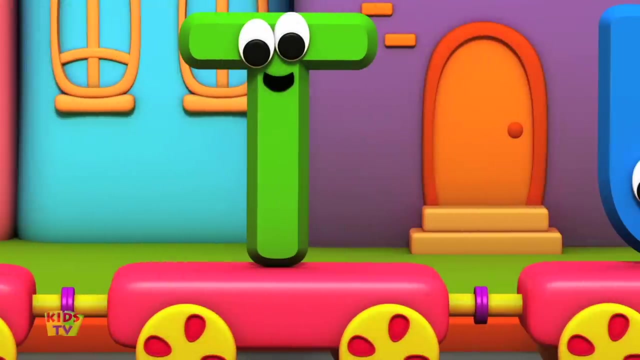 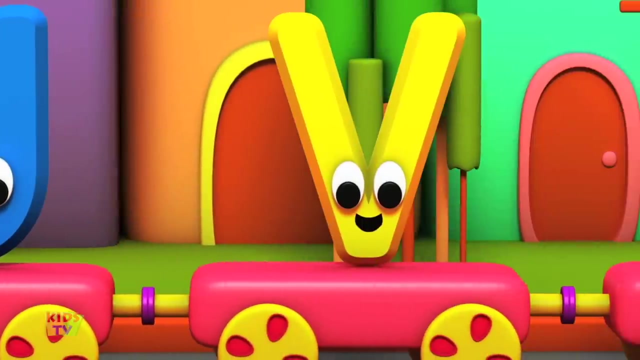 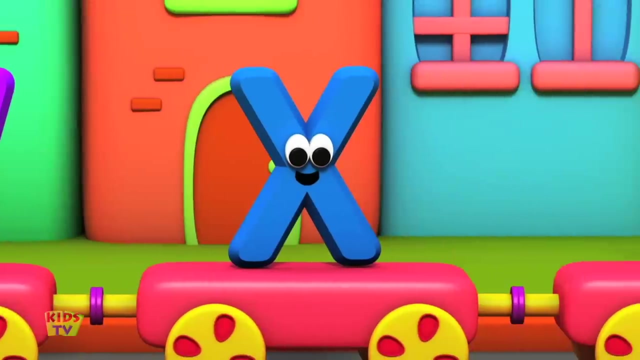 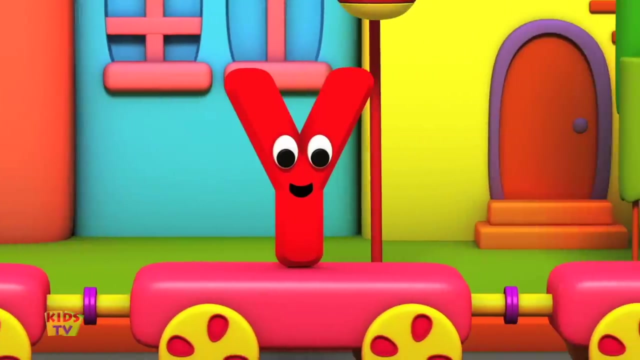 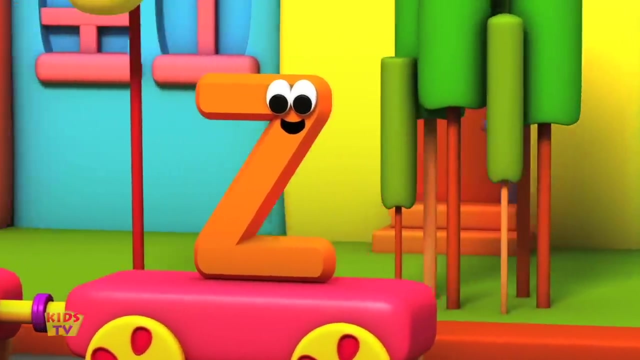 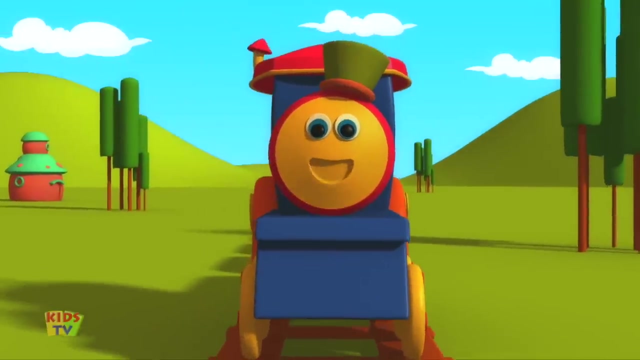 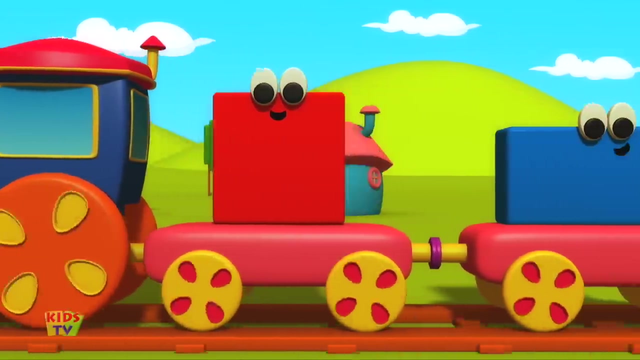 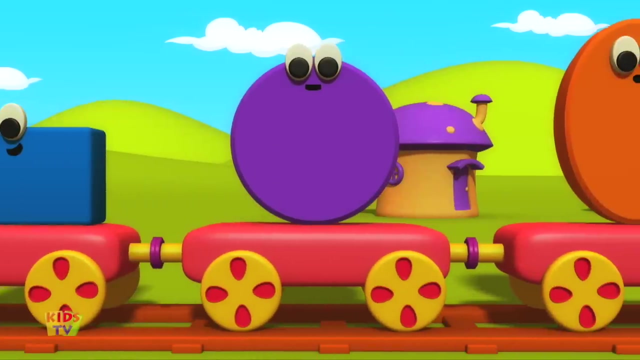 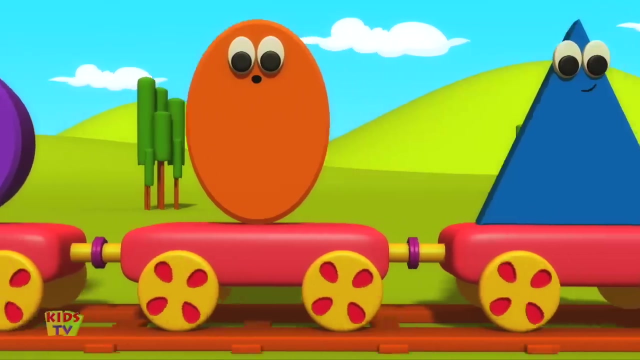 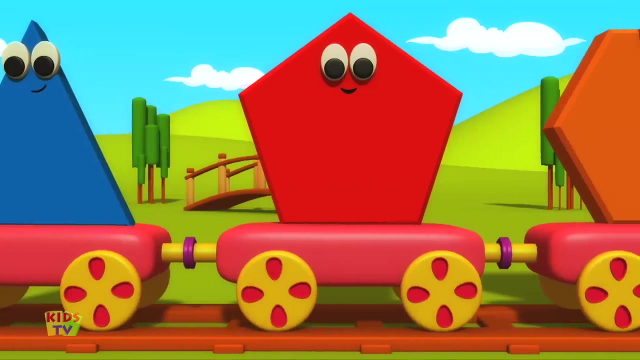 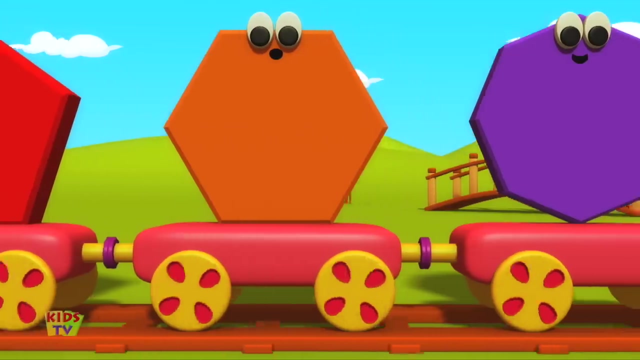 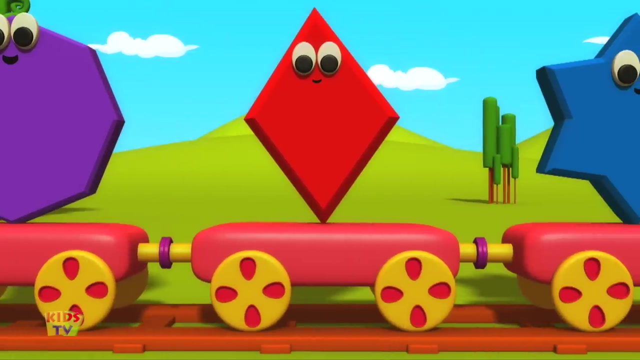 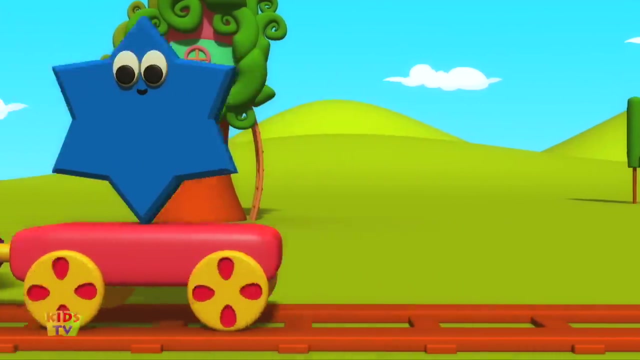 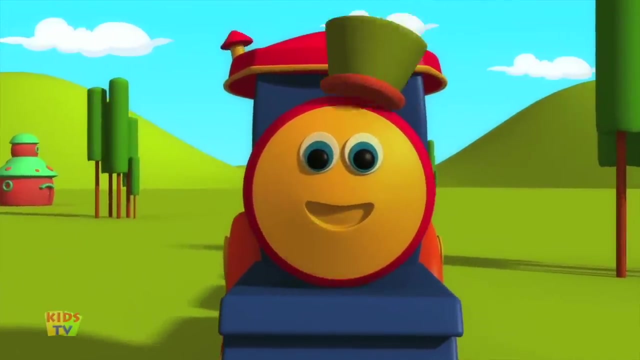 J, K, L, M, N, O, P, Q, R, S, T, U, V, W, X, Y Z. Let's learn about shapes, Squares, Rectangles, Circles, Ovals, Triangles, Pentagons, Hexagons, Octagons, Diamonds, Stars. Let's learn the colors Red. 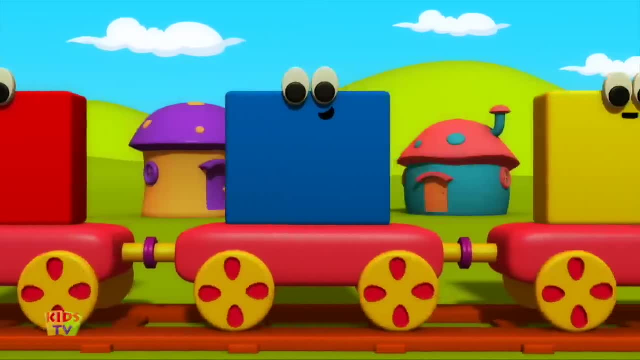 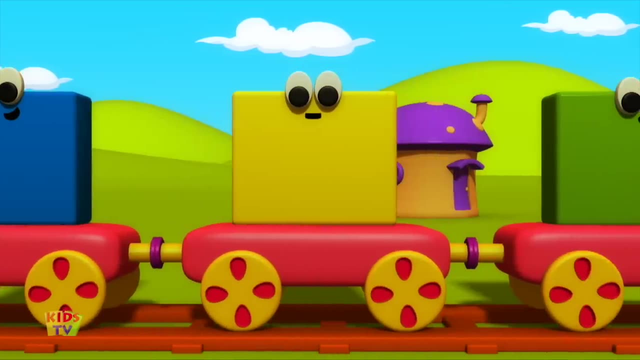 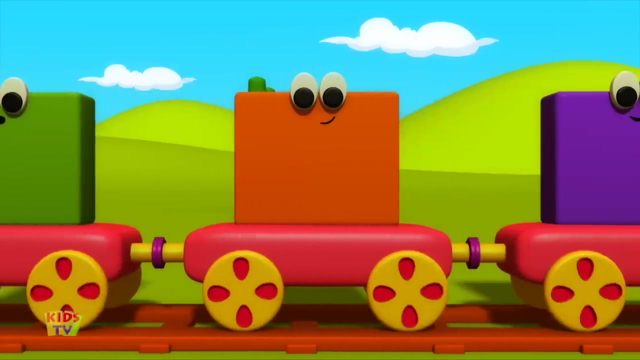 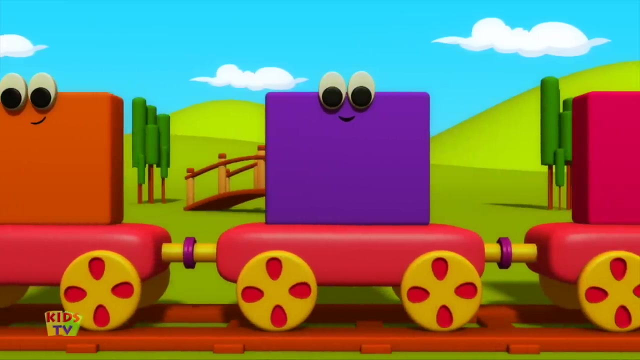 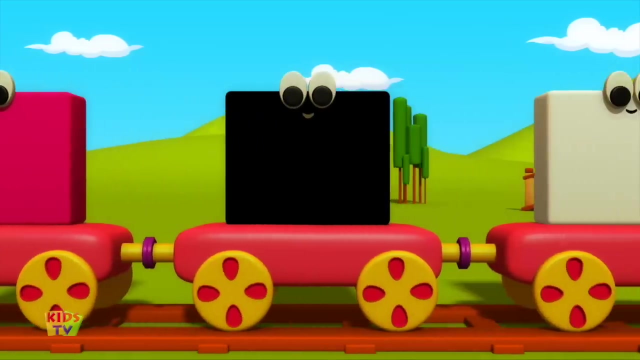 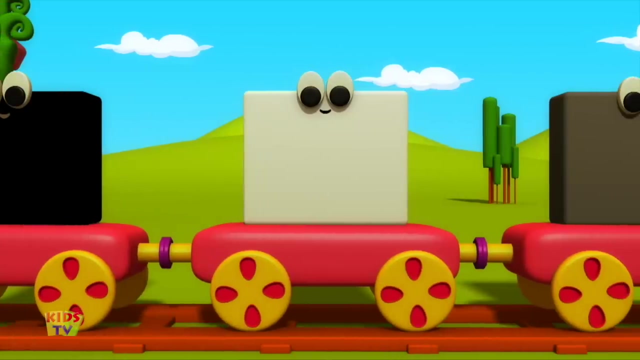 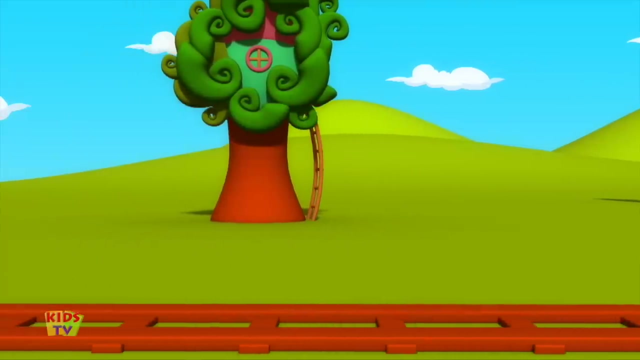 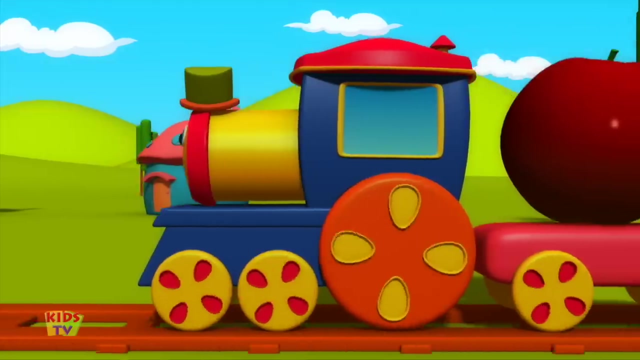 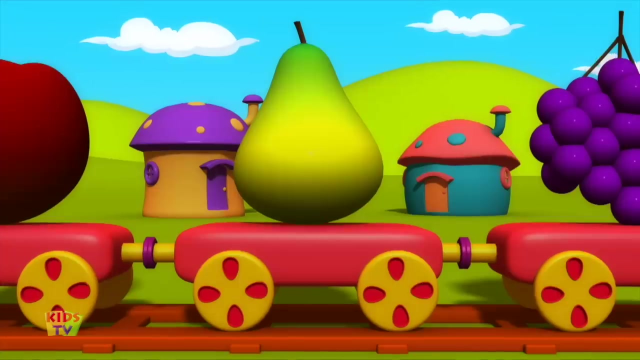 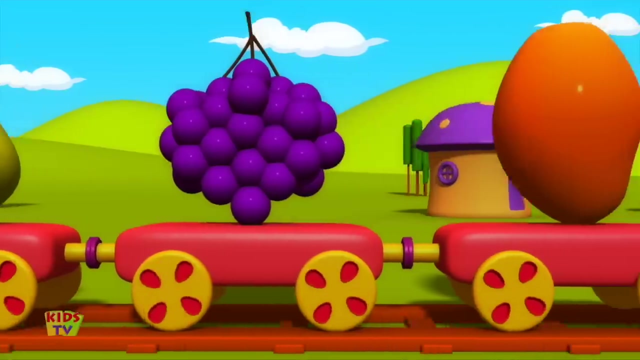 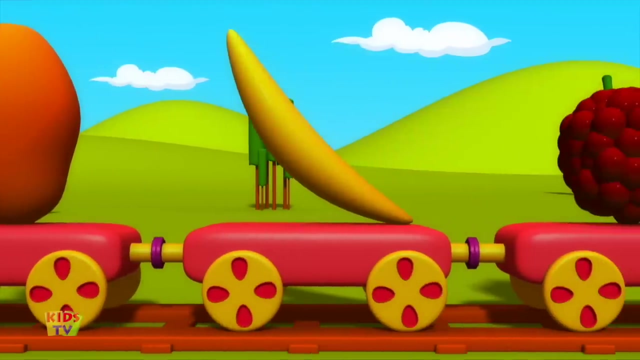 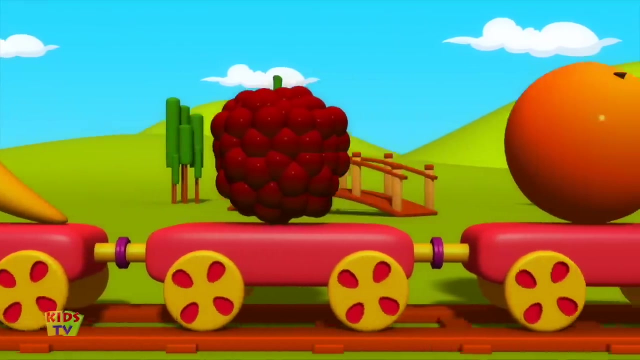 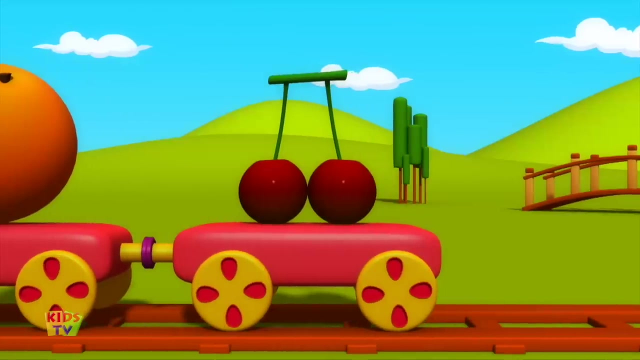 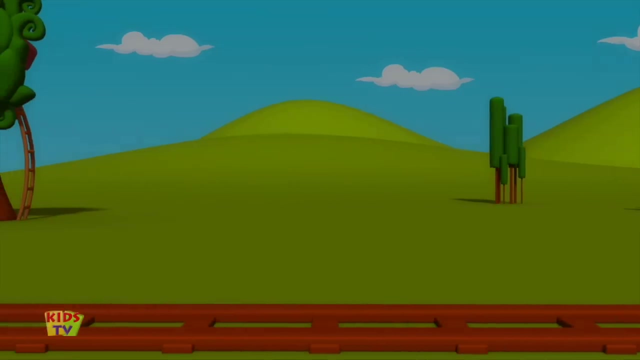 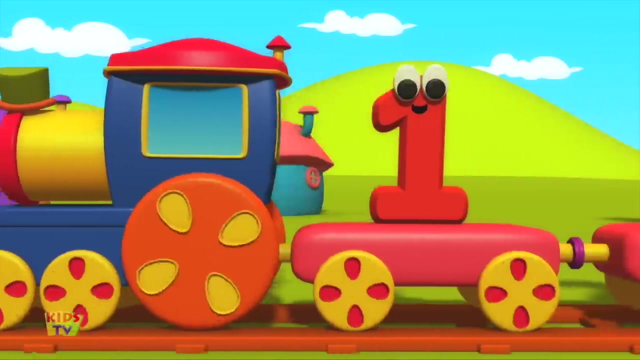 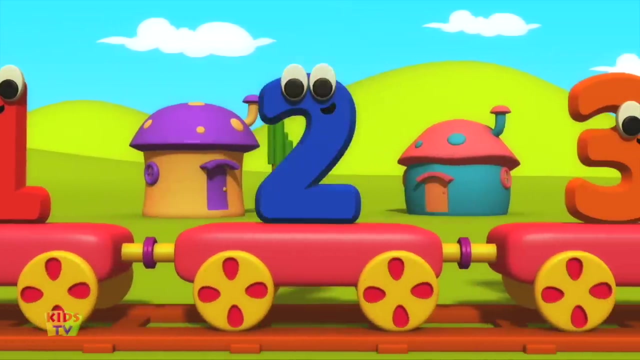 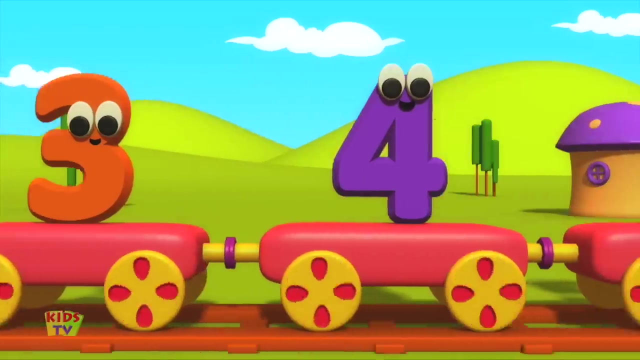 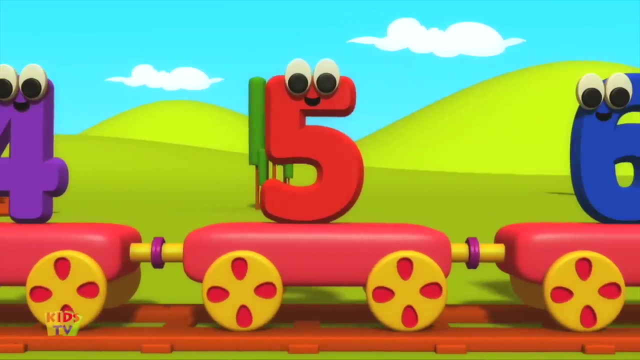 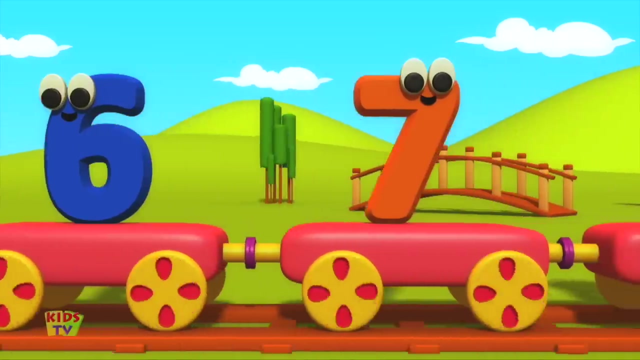 Yellow, Blue, Yellow, Green, Orange, Purple, Pink, Black, Blue, White, White, White, White, White, Gray. Let's learn about fruits: Apple, Apple, Hair, Hair, Hair, Grapes, Mango, Banana, Custard, Apple, Orange, Cherries. Let's learn the numbers One, Two, Three, Four, Five, Six, Seven, Eight, Nine, Ten. 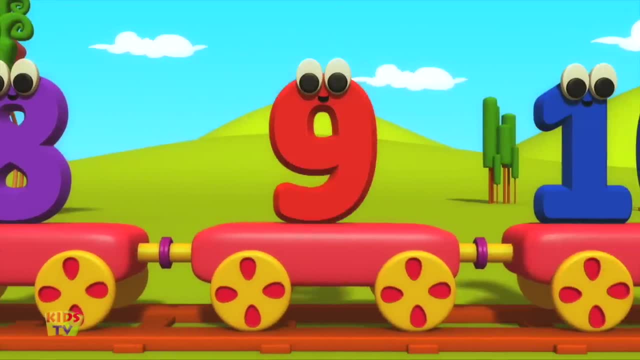 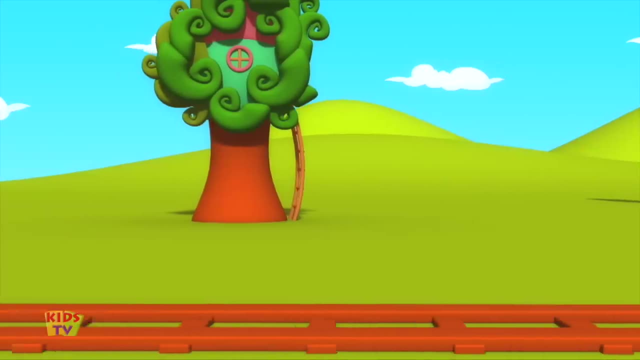 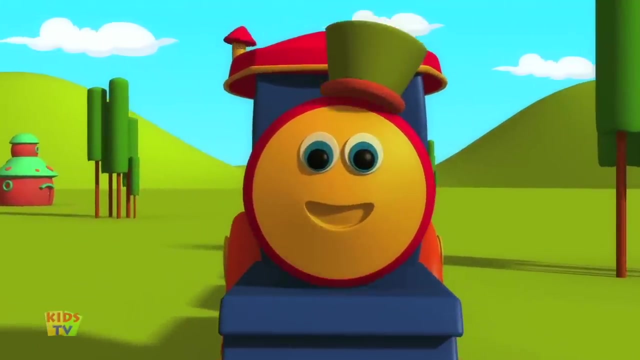 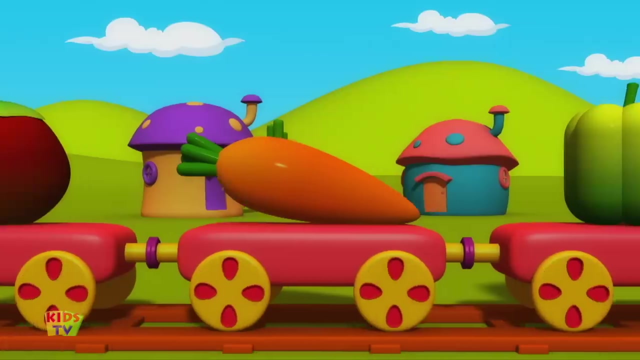 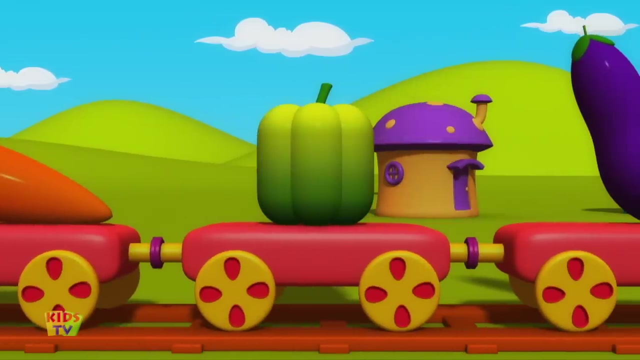 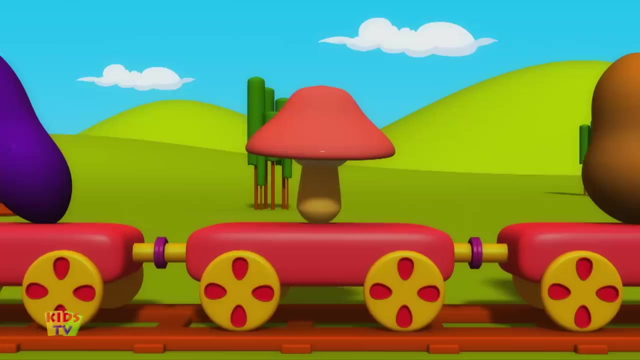 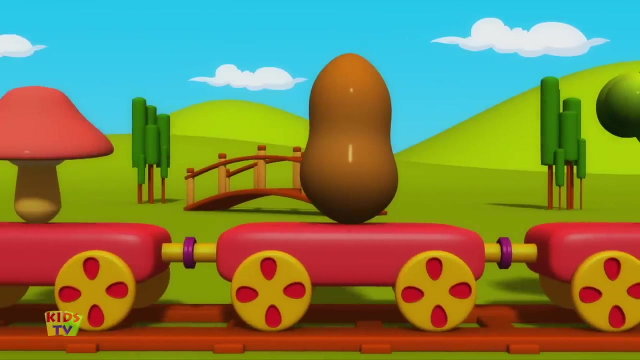 Let's learn about the numbers One, Two, Three, Four, Five, Six, Seven, Eight, Nine, Ten, Eleven, Twelve, Thirteen, Thirteen, Four, Four, Three, Two, One, Two, One, Two, Three, Two, One, Two, Three, Two, One, Two, Three, Two, One, Two, Two, Three, Three, Four, Four, Three, Two, One, Two. 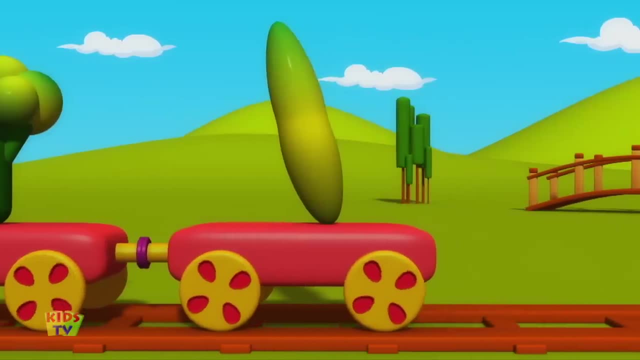 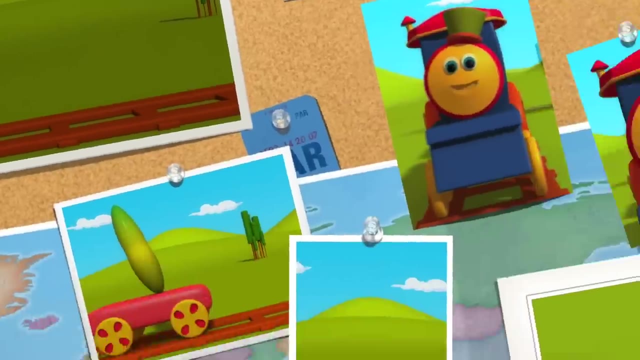 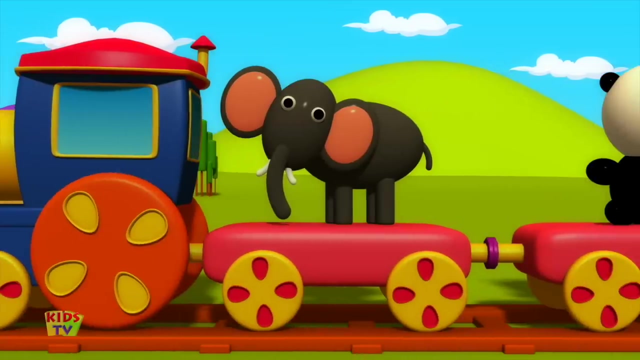 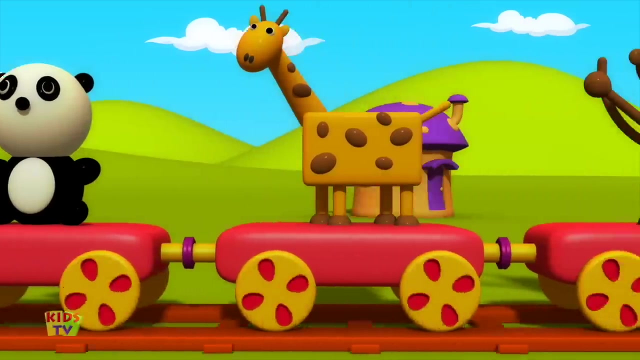 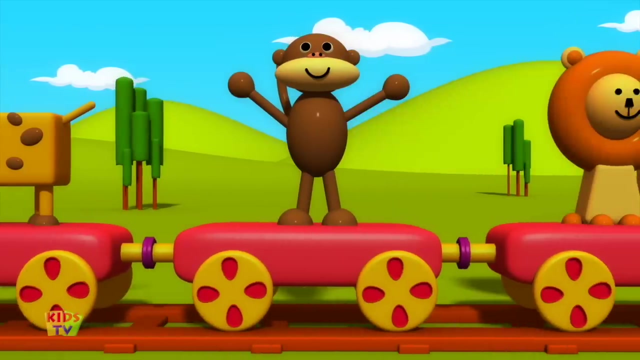 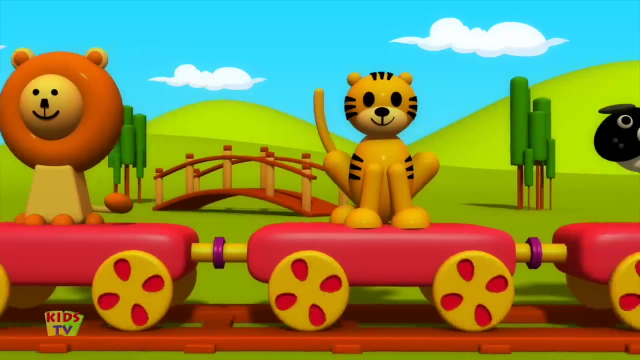 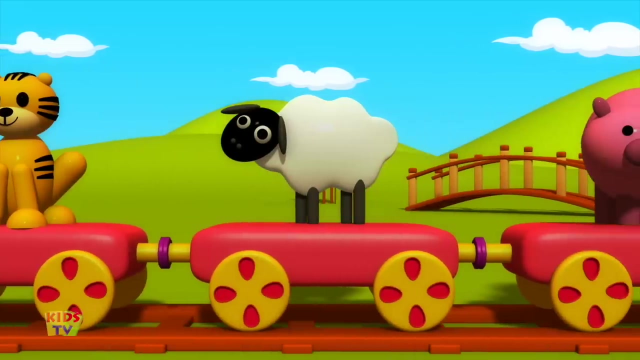 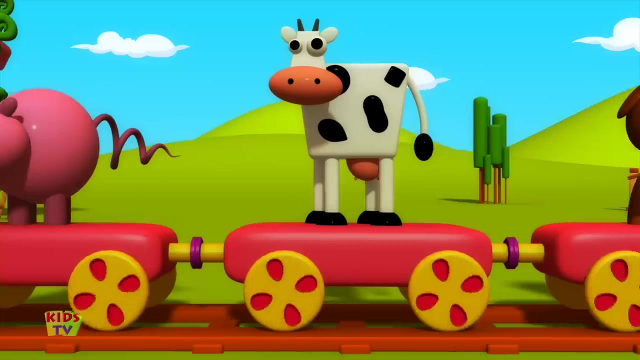 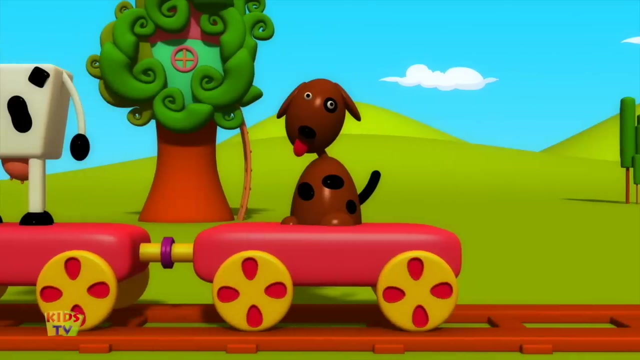 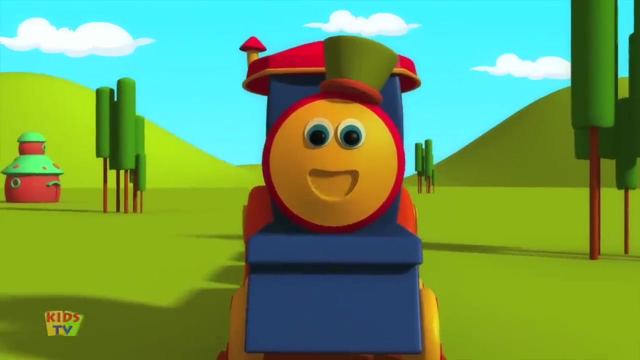 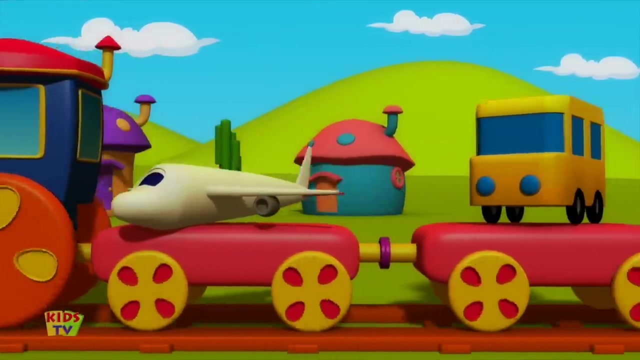 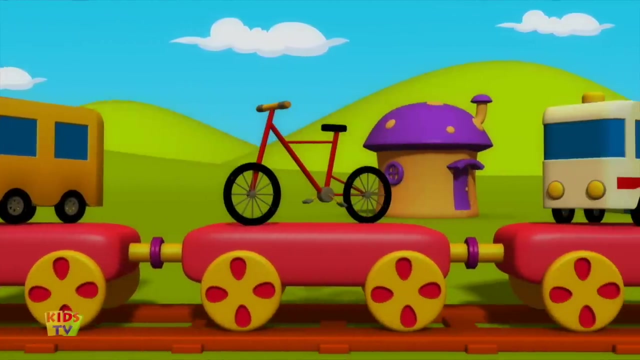 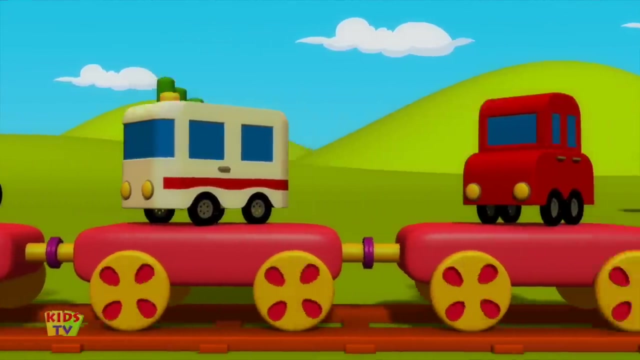 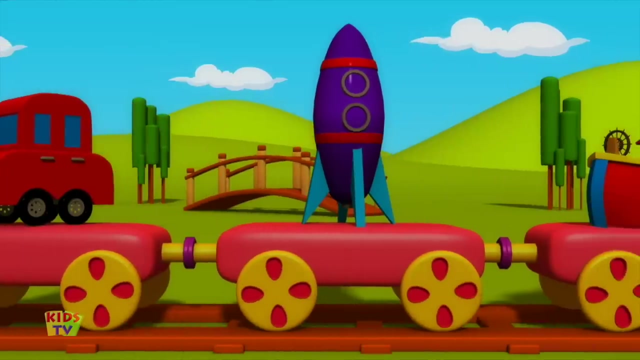 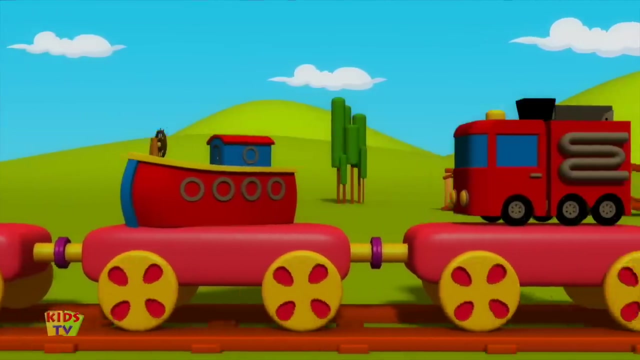 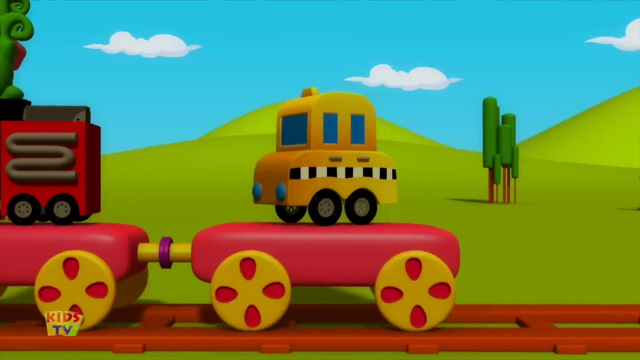 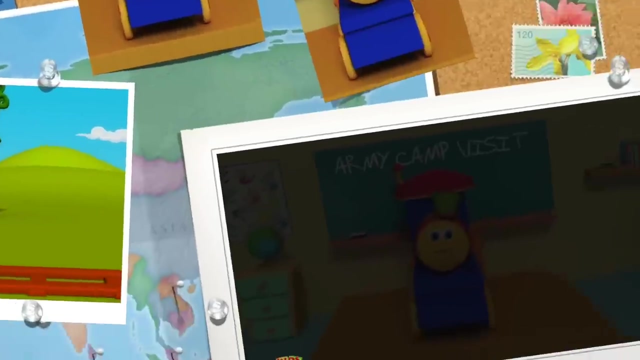 Two, One, Two, Three, Four, Four, Five, Four, Five, Six, Seven, Ten One, Two, Three, Three, Four. Two One, Two, Three, Two Giraffe, Monkey, Lion, Tiger, Sheep, Pig, Cow, Dog. Let's learn about Transport: Aeroplane, Bus, Cycle, Ambulance, Car, Rocket, Ship, Fire engine, Taxi helfen. 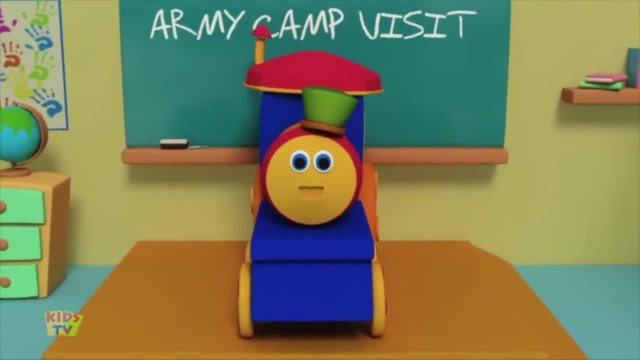 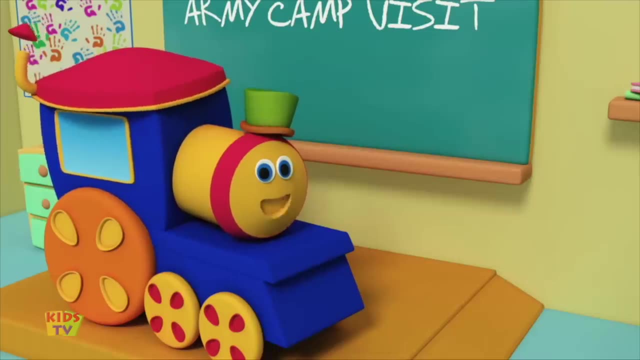 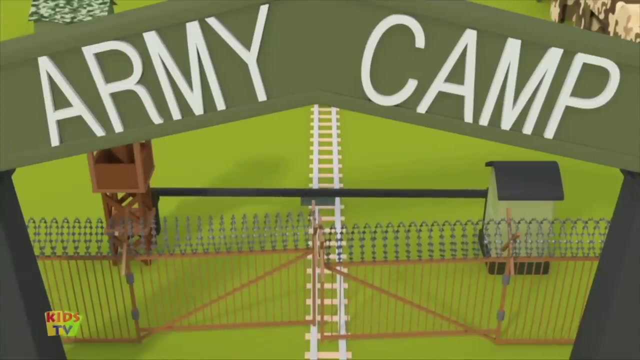 Hello kids, do you want to see something cool today? Yes, we do, We do, Yay, Ok, off to the army camp. we go, Hurry up now, don't be slow. What do you see, kids? We see a tank. 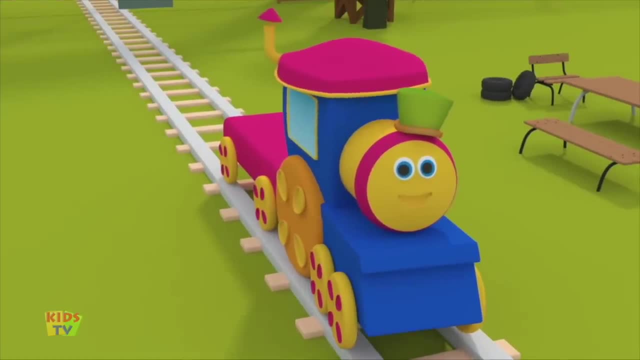 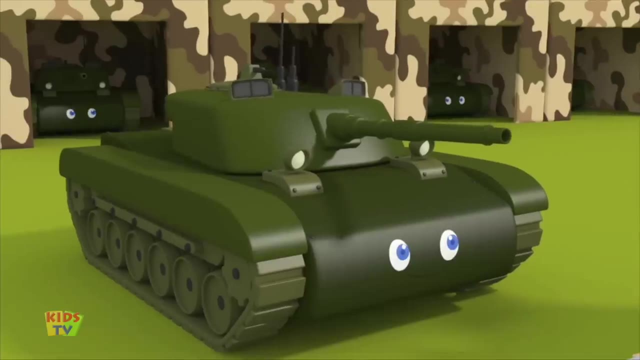 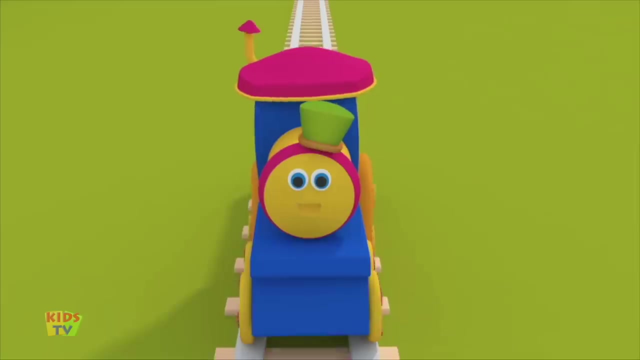 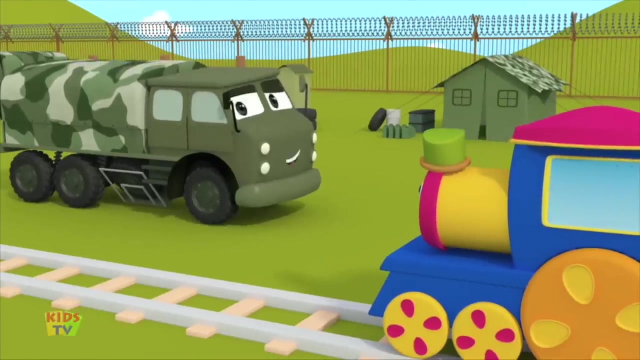 Yes, indeed, in the army camp He is top-ranked. Hello Mr Tank, What do you do? I Protect the country and our border too. Look, there's the army truck. Hello army truck. How are you doing? Hello Bob, I have to deliver goods to the soldiers, So I must get going. 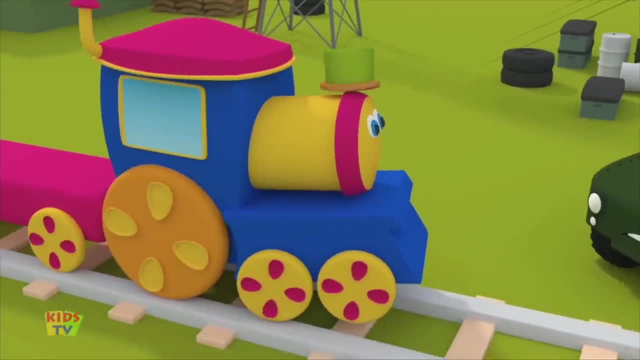 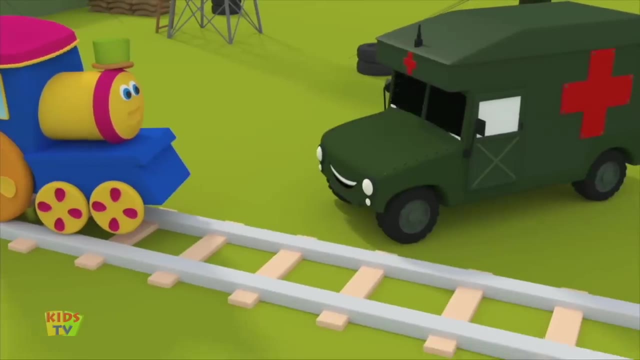 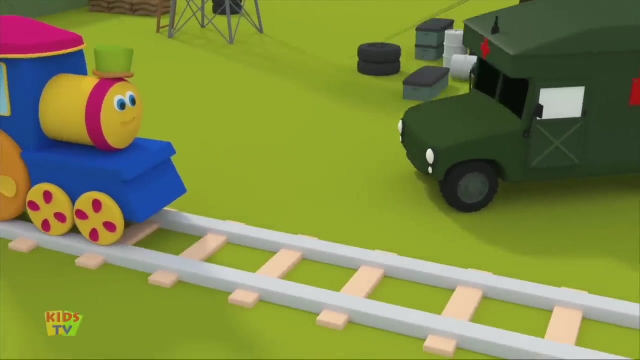 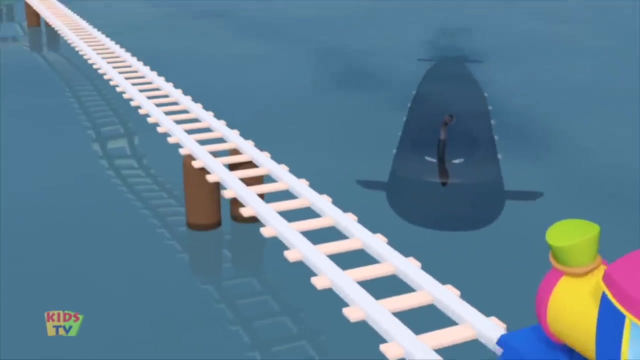 Hi Ambulance. you do look tired, Hey Bob. That's because I'm always required. What do you do all through the day? I help carry the wounded soldiers away. such a great job. What's that coming out of the water? a minute ago it could hardly be seen. 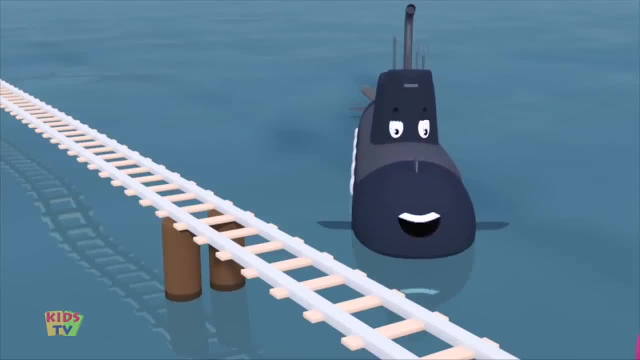 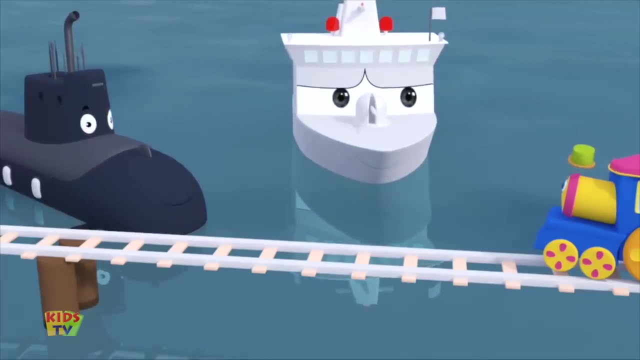 Hi there, Bob. I am mr Sully Submarine. my name means under the sea, both inside and outside the water, I can be Hello submarine, Hello Bob, How do you do? Greetings, mr Navy, Have you been sailing the water blue? 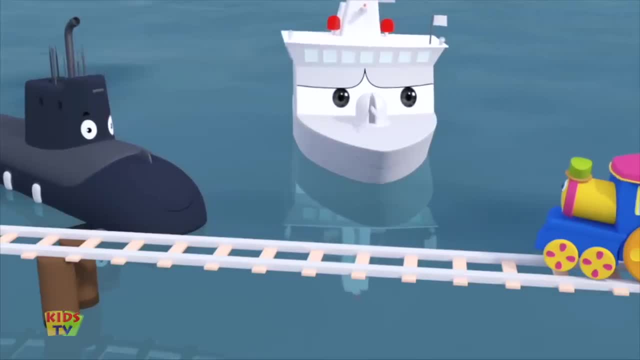 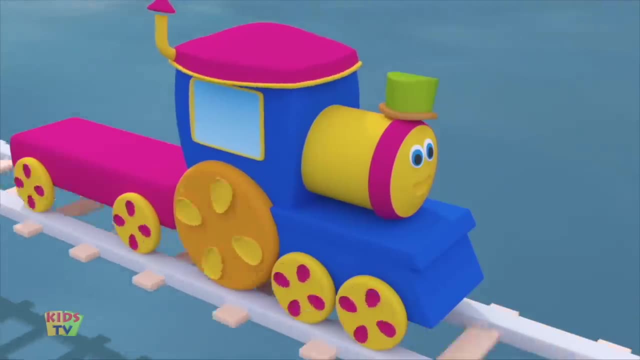 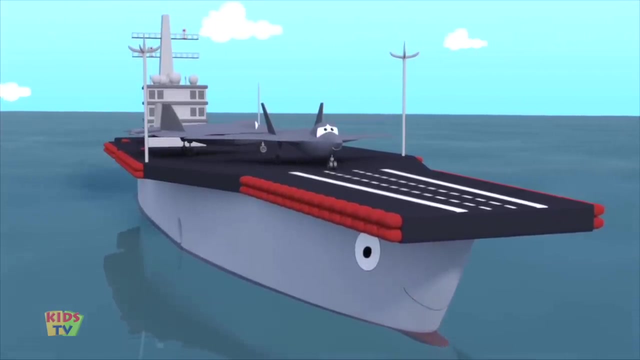 Yes, we sail on the sea and keep safe the coast, and that's certainly something of which you can boast. Look out there, That's an aircraft carrier. Oh, yes, that I am. Hello, my dear, I am the military's base on the sea. all these aircrafts all alone I carry. 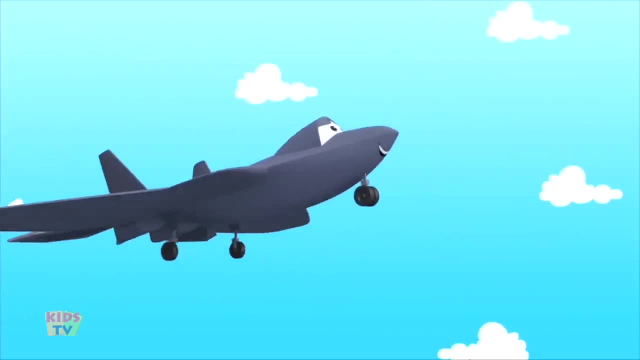 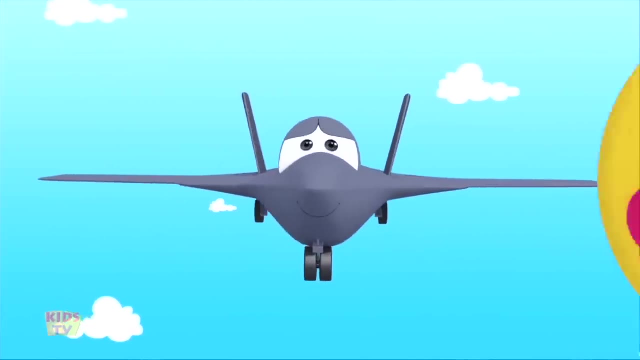 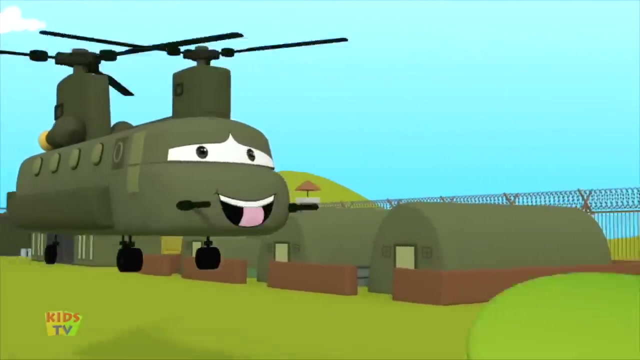 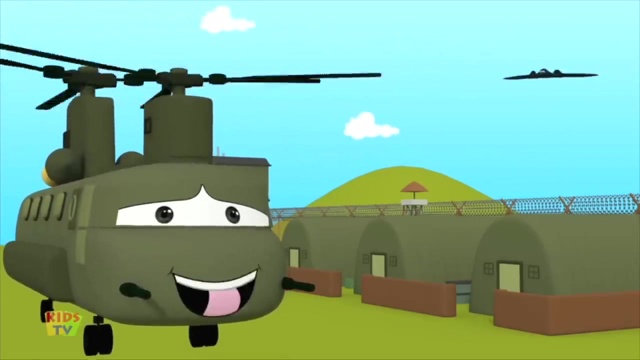 Here comes the fighter aircraft. Oh my, I Fly very high so I can protect the sky. Look up, that's a transport helicopter. What do you do, Hello Bob? How do you do I carry troops through the air and take them places far or near? 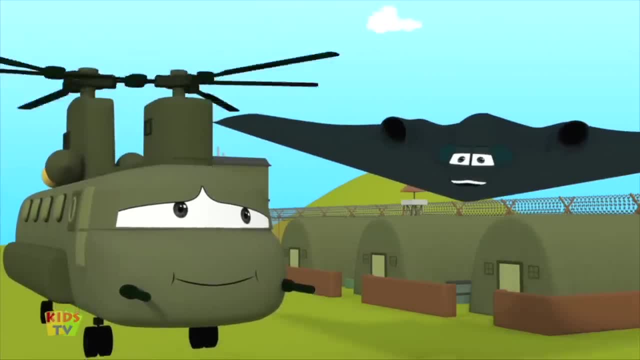 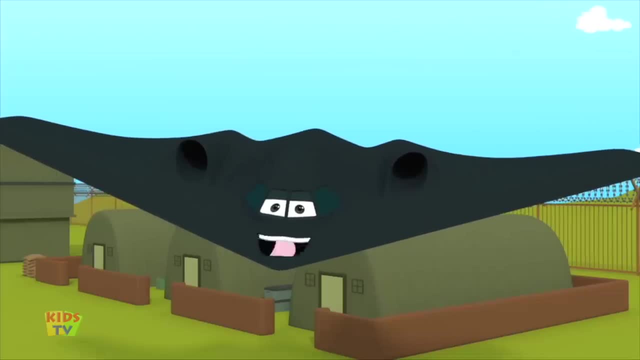 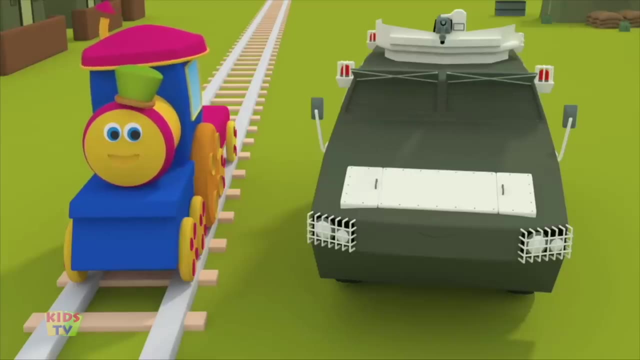 Here comes the bomber. watch out, Hello Bob. My name is bomber and my enemies fear me. My bombs can destroy all targets, on the land or in the sea. Hi, armored personnel carrier, What have you got concealed? Hello, I am carrying military forces to the battlefield. 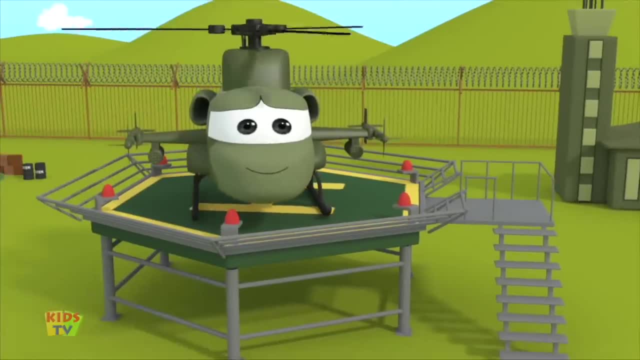 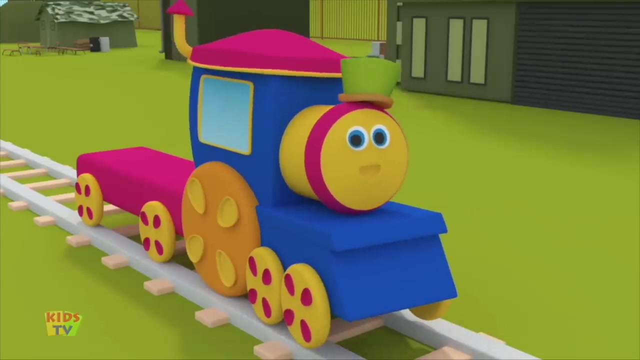 Hi Bob, how are you? Hello helicopter, What do you do? I am a lot like the army truck and I give everyone a helping hand. My job is to connect areas difficult to reach by land. Kids, look there. which Army Transport is that? Can you guess? 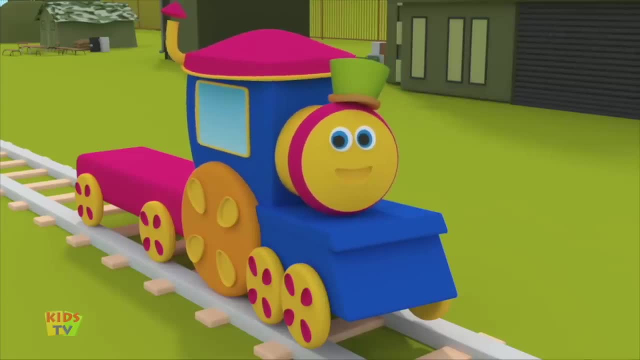 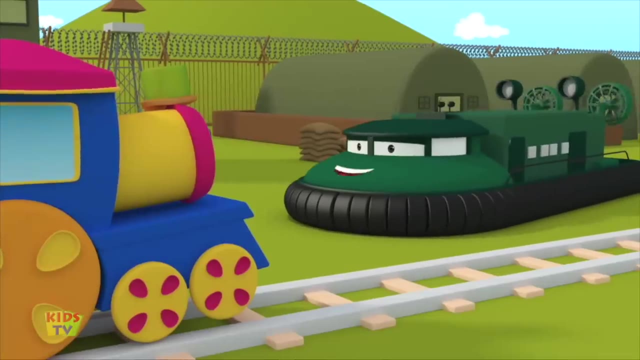 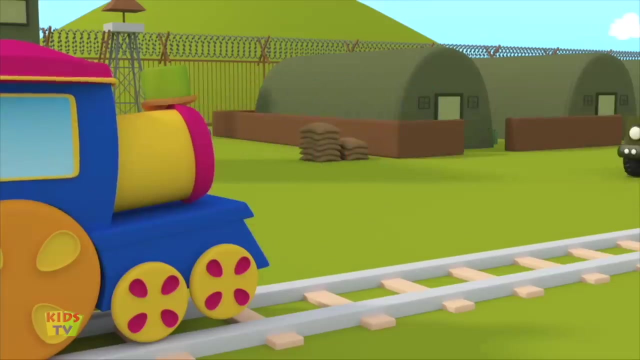 No, Oh, please No. that's a different one, That's an army hovercraft. Oh goodness me, here it comes. I can drive on any kind of surface and I go where there are big problems. Look over there, kids, here comes the army jeep. 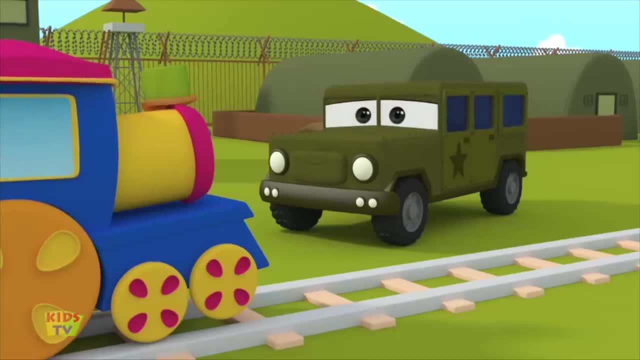 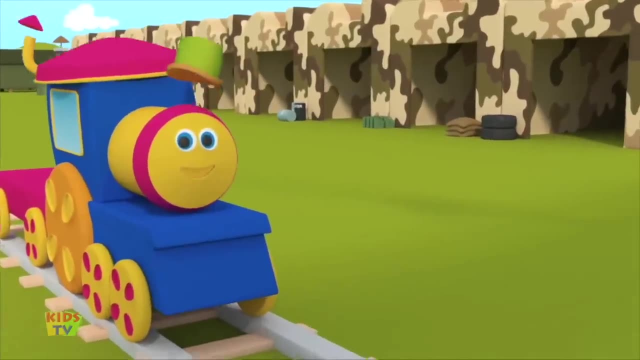 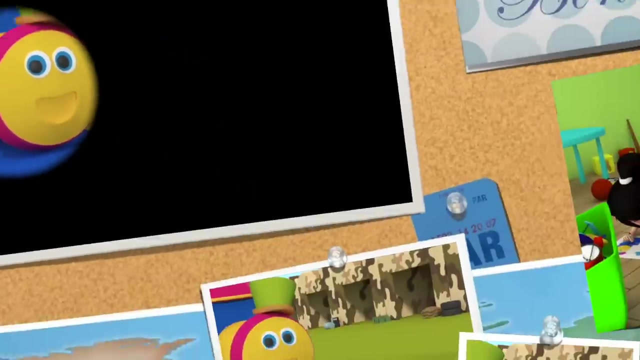 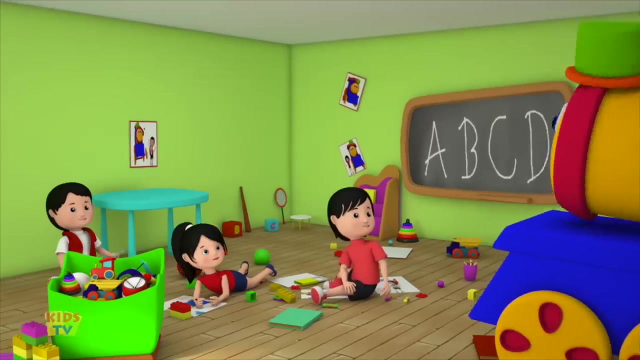 Hi Bob, I can easily drive over rough roads, no matter how high or deep. Kids, I hope at the army camp you had fun. Bye bye. now I have got to run. Bye bye Bob. Hey kids, let's play with the colourful crayons. 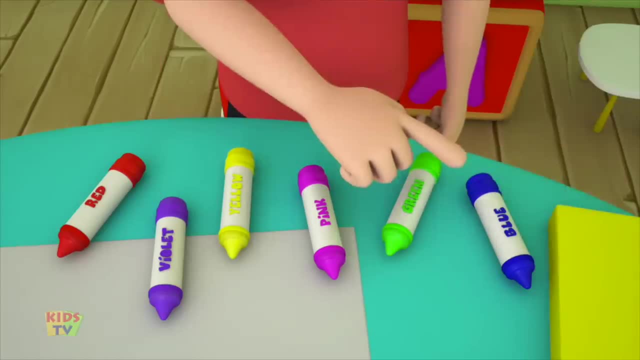 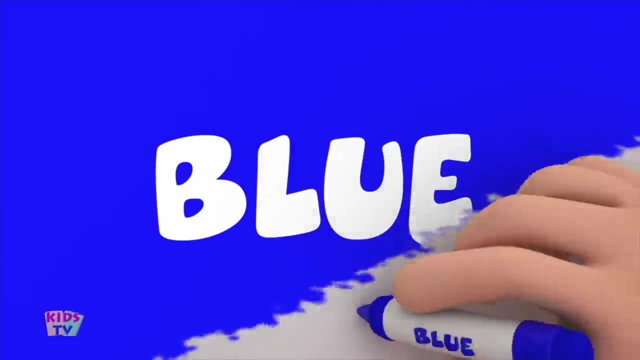 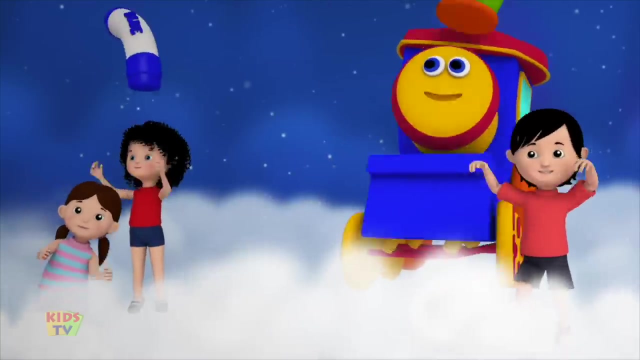 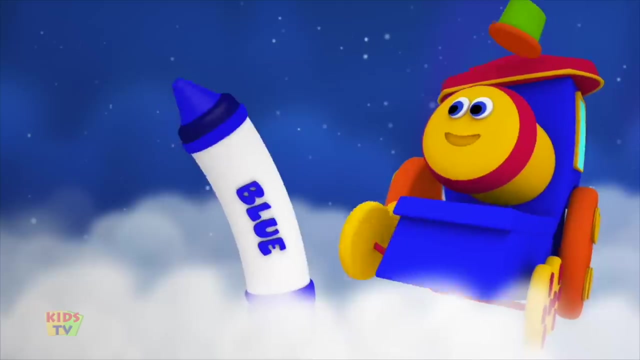 Come, let us pick a colour. look, we've got the colour blue. Put the crayon to face And paint a beautiful sky. It looks so pretty, don't you think? Don't you love the colour blue? It's just one of the colours in our crayons box. 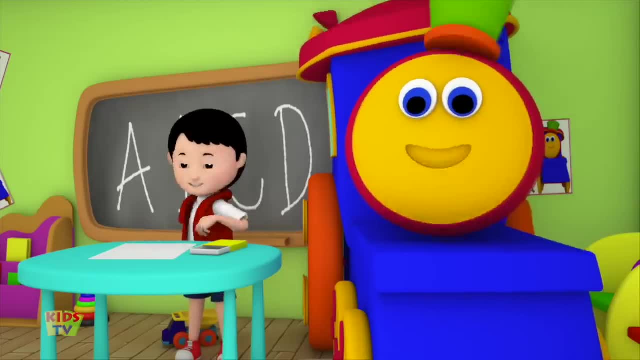 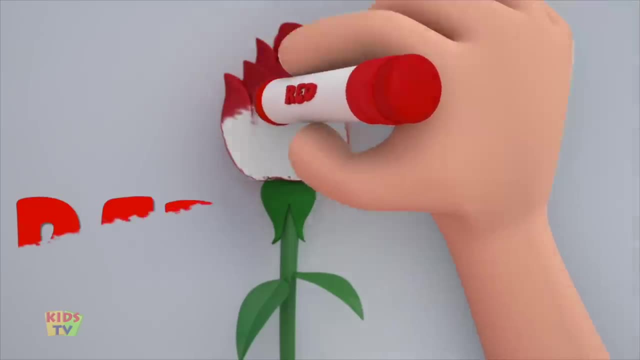 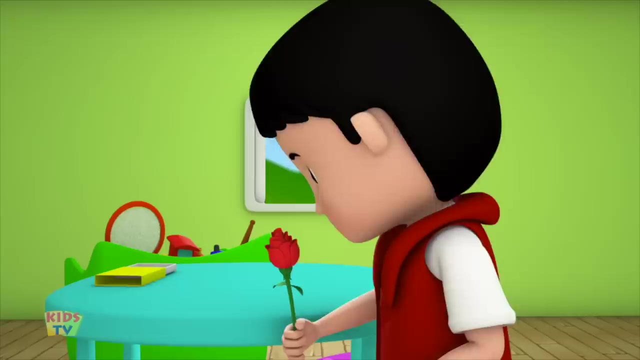 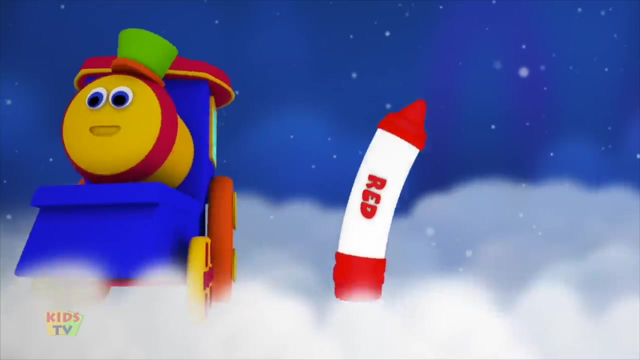 Come, let us pick a colour. look, we've got the colour red. Put the crayon to paper And paint a lovely rose. It looks so pretty, don't you think? Don't you love the colour red? It's just one of the colours in our crayons box. 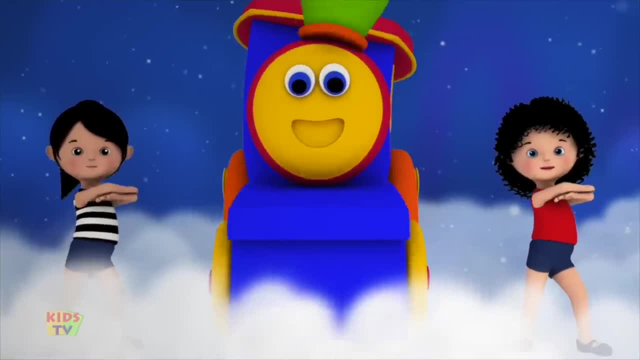 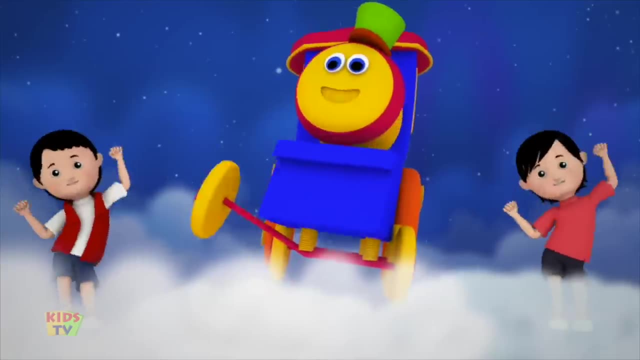 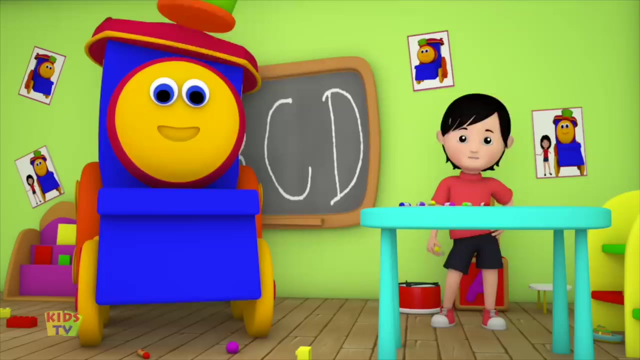 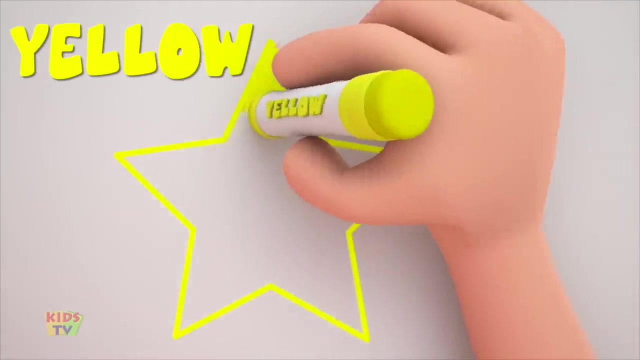 Come, let us pick a colour. look, we've got the colour yellow. Put the crayon to paper And paint a twinkling star. It looks so pretty, don't you think? Don't you love the colour yellow? It's just one of the colours in our crayon box. 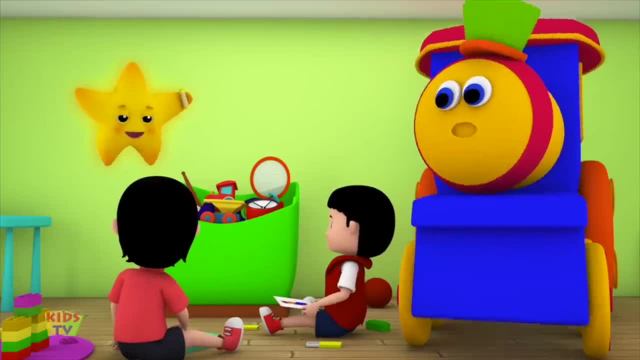 Put the crayon to paper And paint a twinkling star. It looks so pretty, don't you think? Don't you love the colour yellow? It's just one of the colours in our crayon box. Put the crayon to paper. 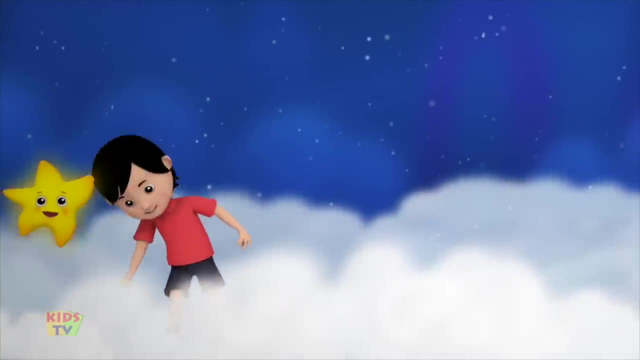 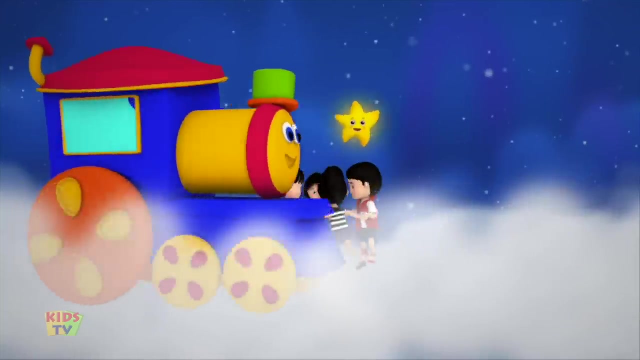 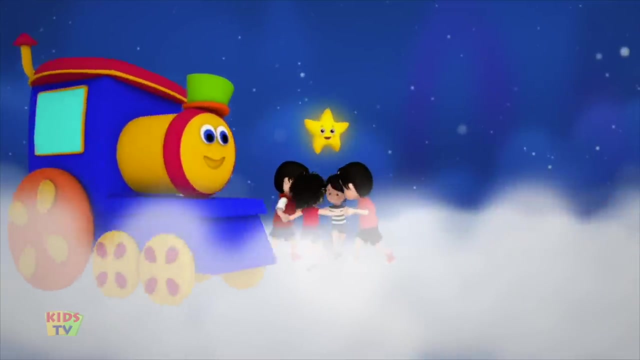 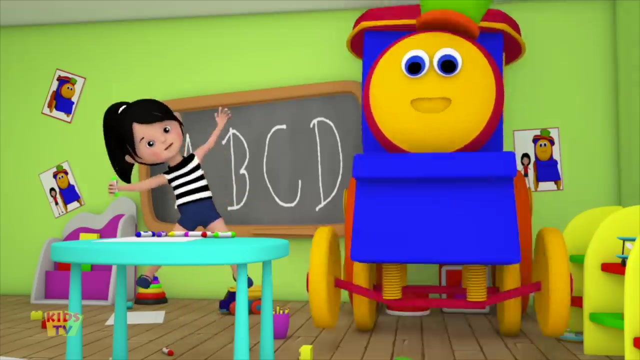 And paint a twinkling star. It looks so pretty, don't you think? Don't you love the colour yellow? It's just one of the colours in our crayon box. Come, let us pick a colour. look, we've got the colour blue. 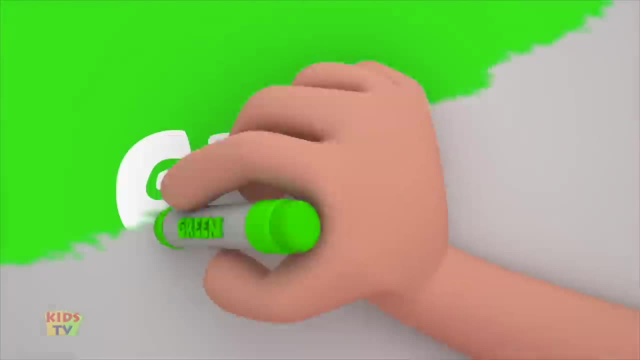 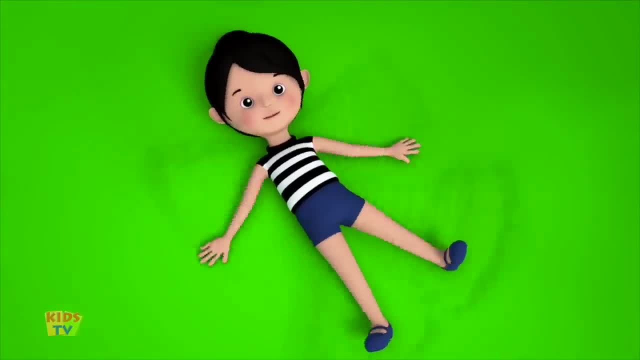 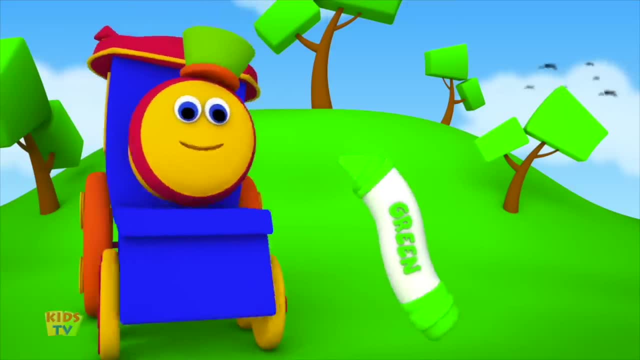 It's just one of the colours in our crayon box. Put the crayon to paper And paint a twinkling star. It's just one of the colours in our crayon box. Put the crayon to paper And paint a lovely field. 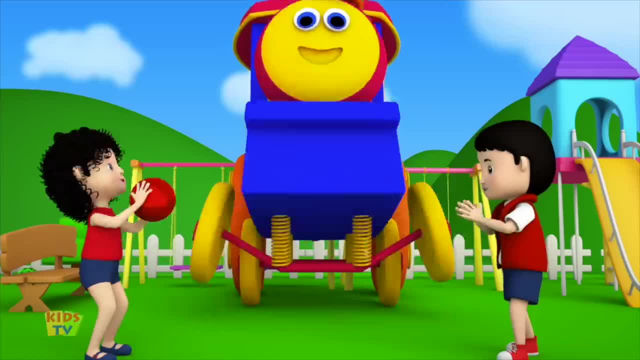 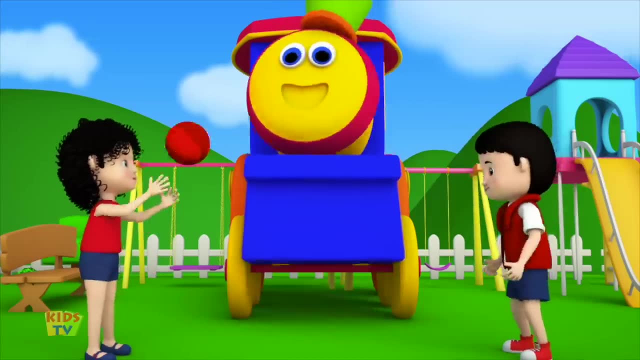 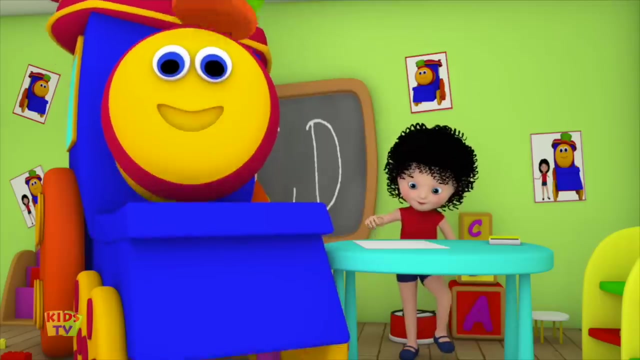 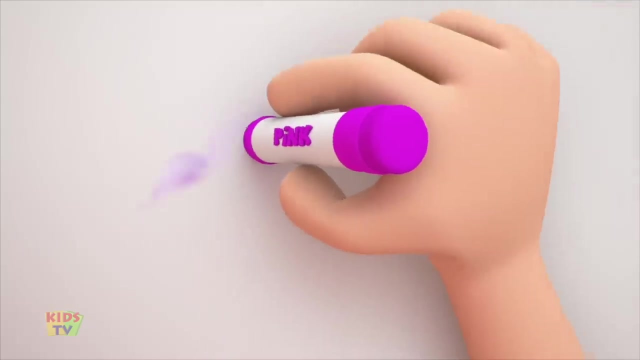 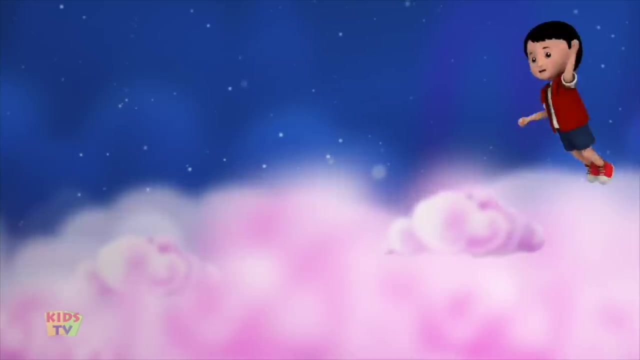 It looks so pretty, don't you think? Don't you love the colour green? Come, let us pick a color. Look, we've got the color pink. Put the crayon to paper And paint some cotton candy. It looks so pretty, don't you think? Don't you love the color pink? 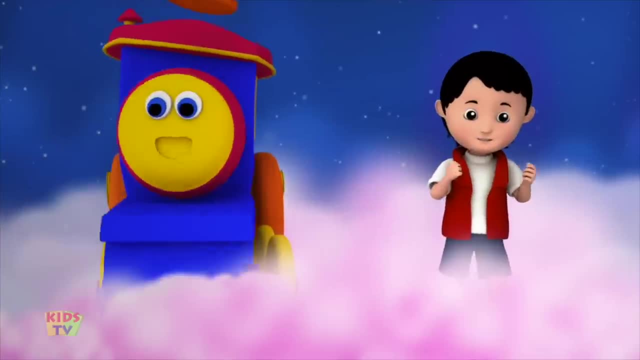 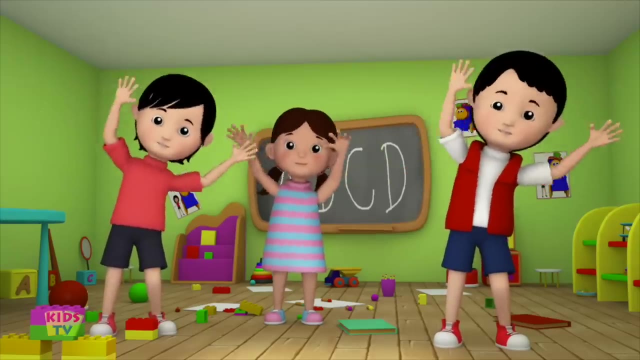 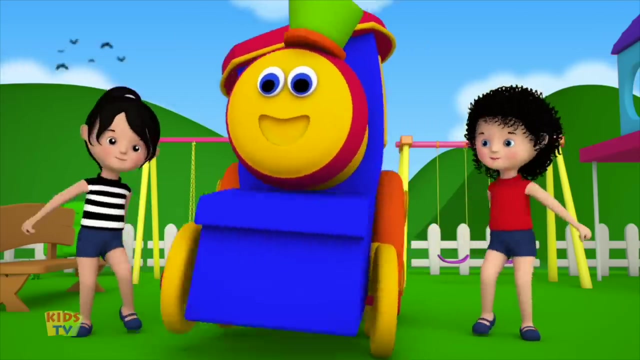 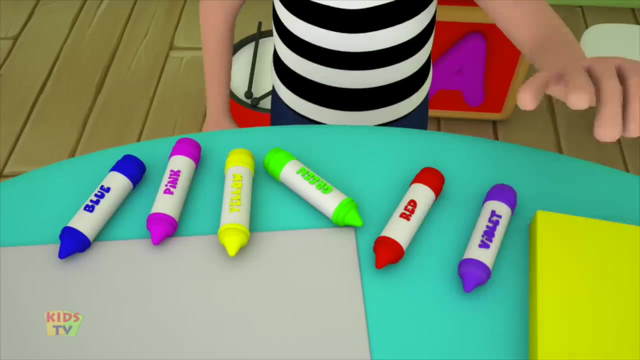 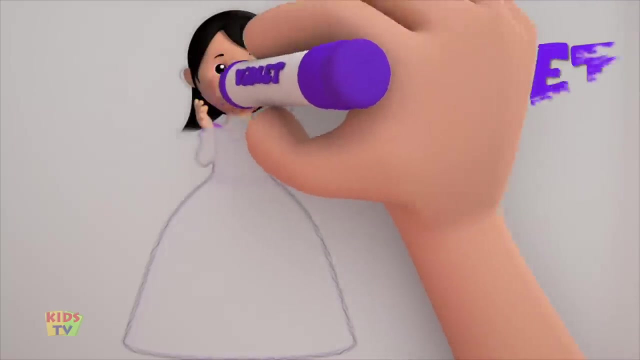 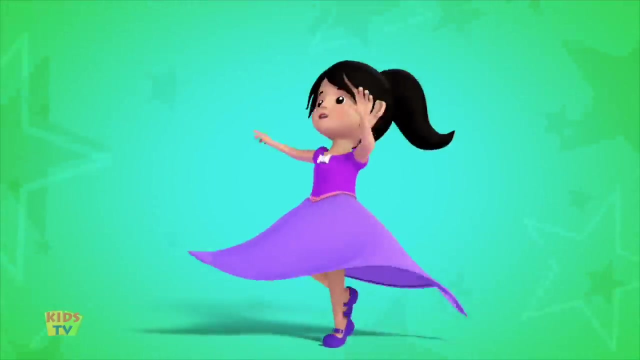 It's just one of the colors In our crayon's box. Come, let us pick a color. Look, we've got the color violet. Put the crayon to paper And paint a princess dress. It looks so pretty, don't you think? Don't you love the color violet? 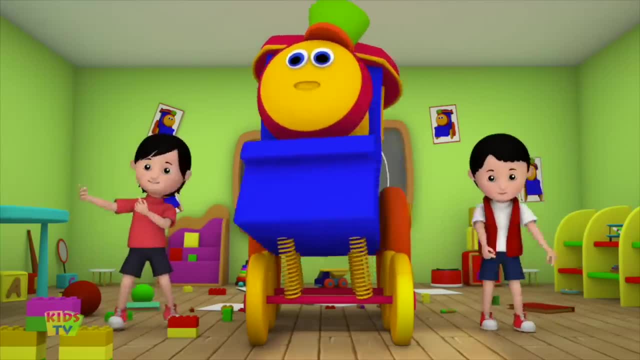 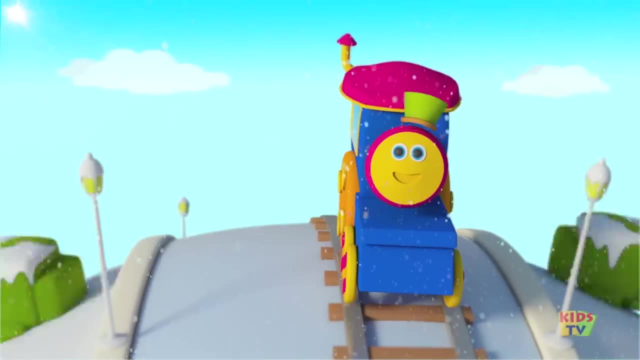 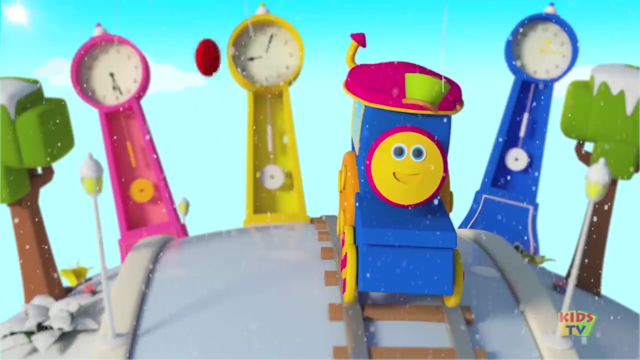 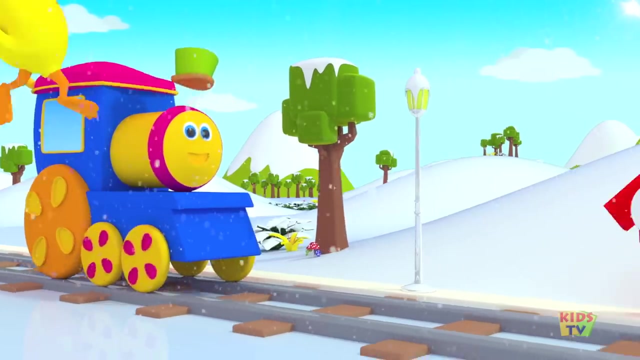 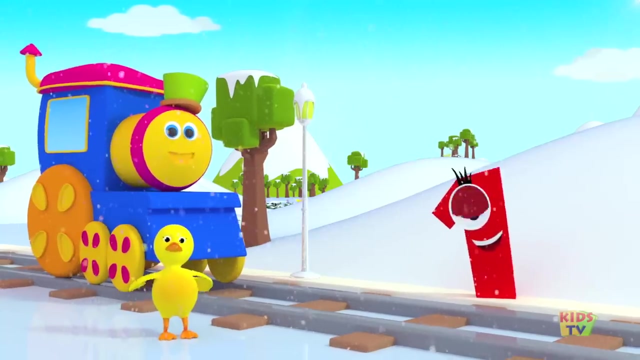 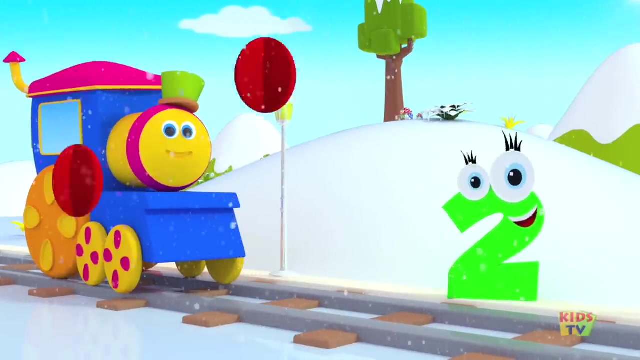 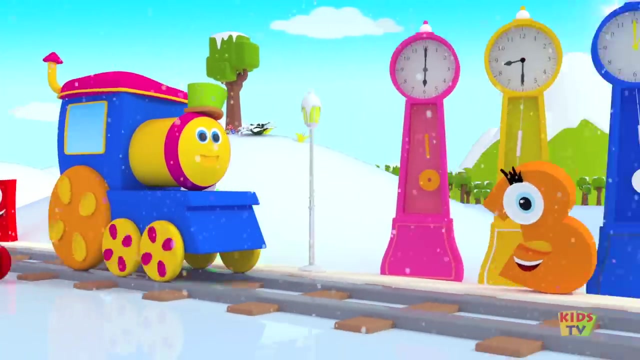 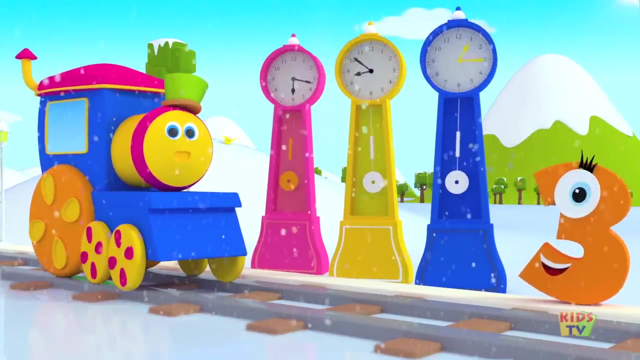 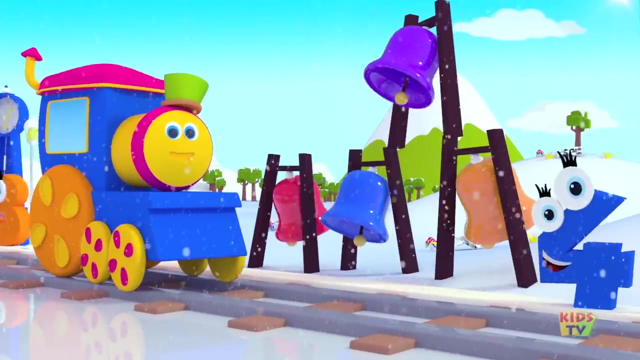 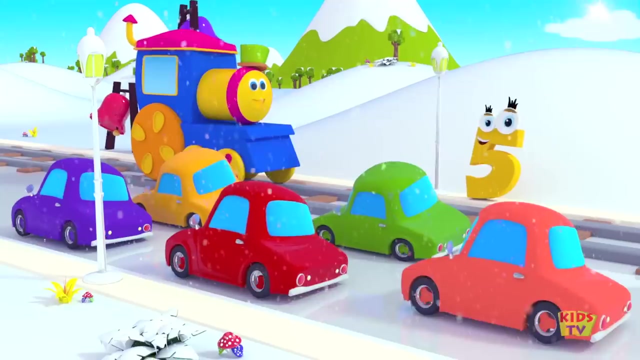 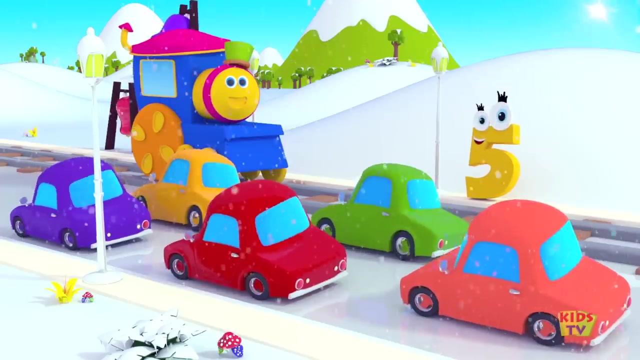 It's just one of the colors In our crayon's box. Shall we go on a numbers counting ride With Bob the train? Yes, Ok, hop on aboard. Thanks, Bob. It's just one of the colors In our Beep, beep, beep. Five new cars, Six. 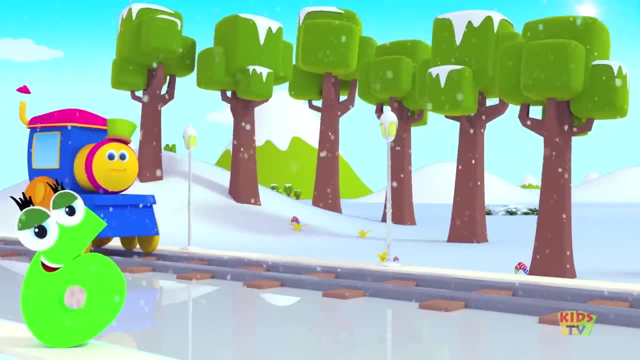 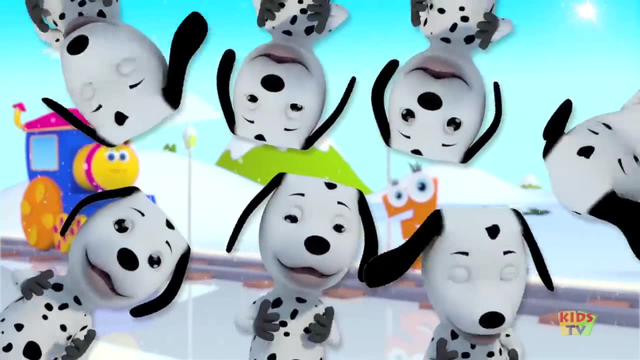 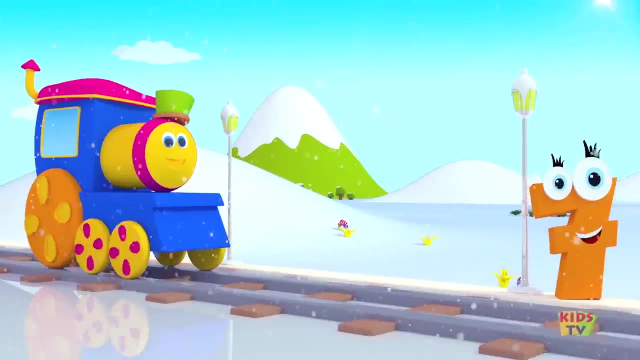 Six tall trees. Swish swish swish Swish swish swish. Six tall trees. Seven, Seven naughty dogs. Woof, woof, woof, Woof, woof, woof. Seven naughty dogs. Eight Eight noisy drums, Bang bang bang. 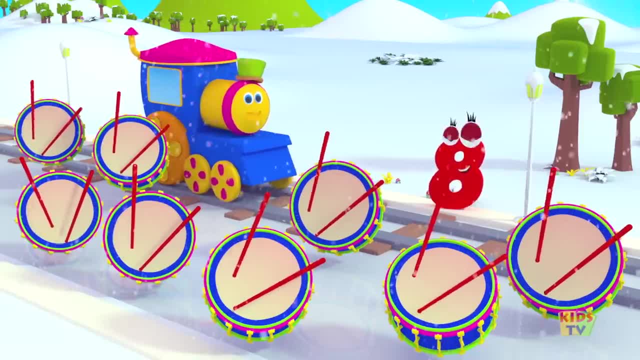 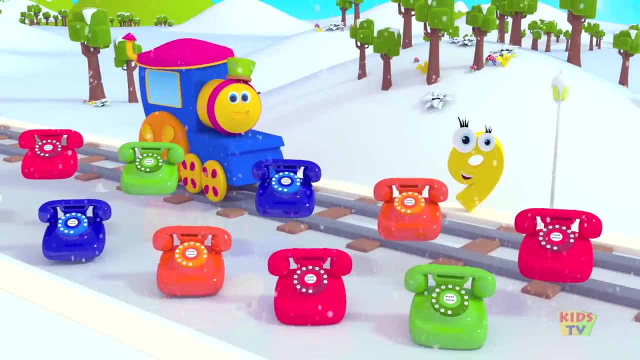 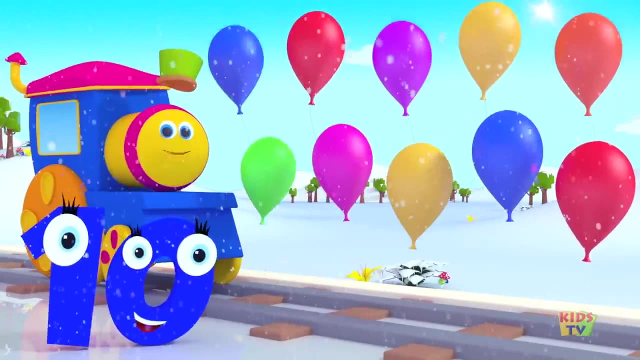 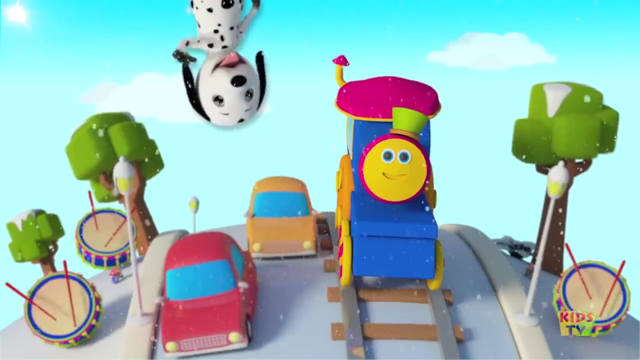 Bang, bang, bang. Eight noisy drums. Nine Nine ringing phones: Tring tring, tring, Tring, tring, tring. Nine ringing phones. Ten, Ten pretty balloons. Pop, pop, pop, Pop, pop, pop, Ten pretty balloons, Wasn't that fun. 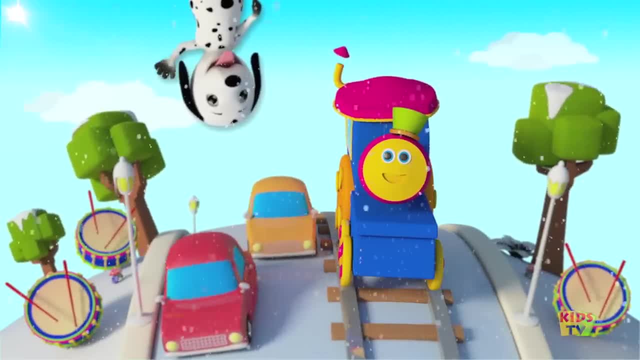 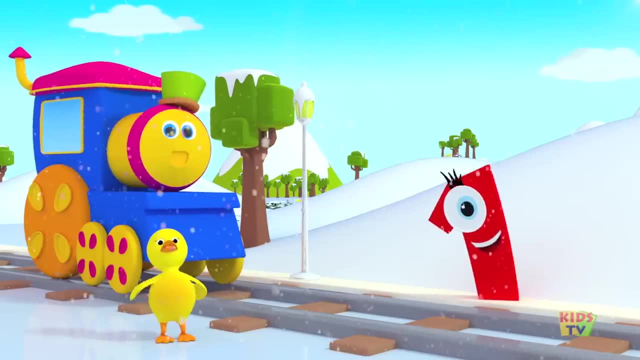 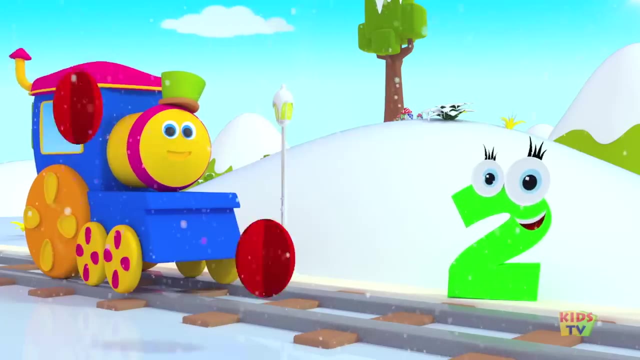 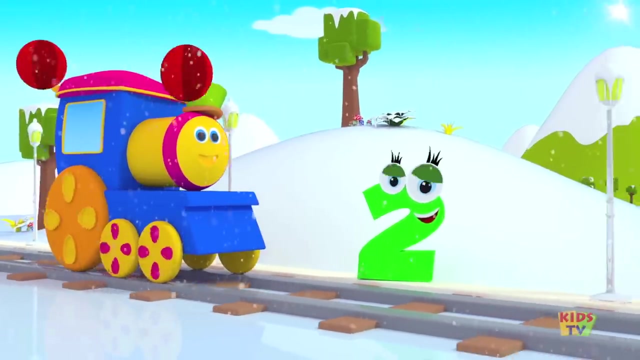 Let's do it one more time. One, One, One little duck, Quack, quack, quack, Quack, quack, quack. One little duck. Two. Two red balls: Bounce, bounce, bounce, Bounce, bounce, bounce. Two red balls, Three. 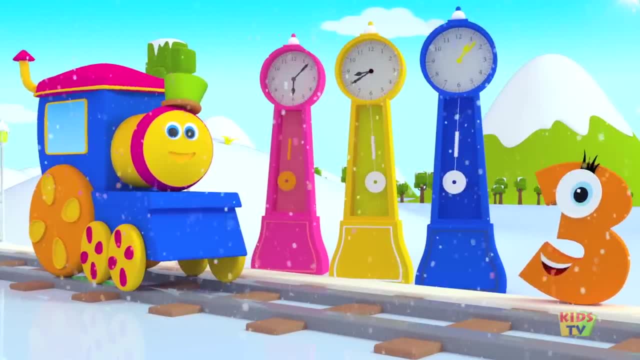 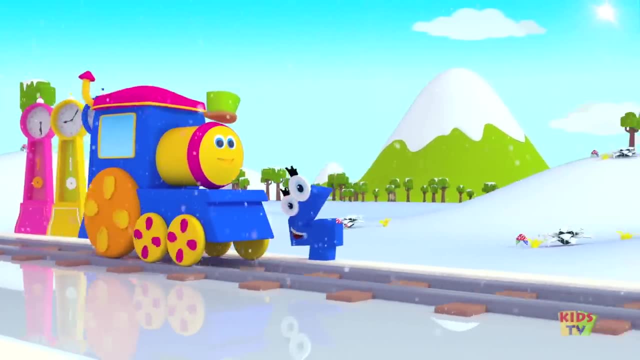 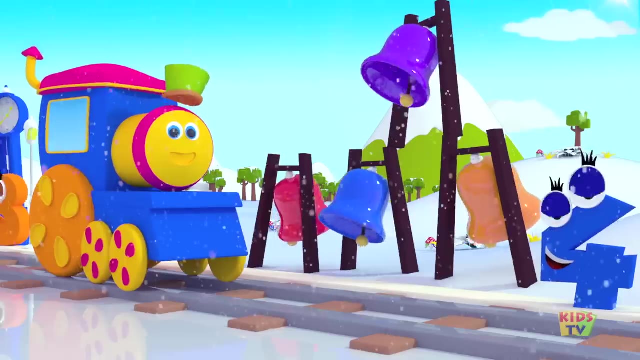 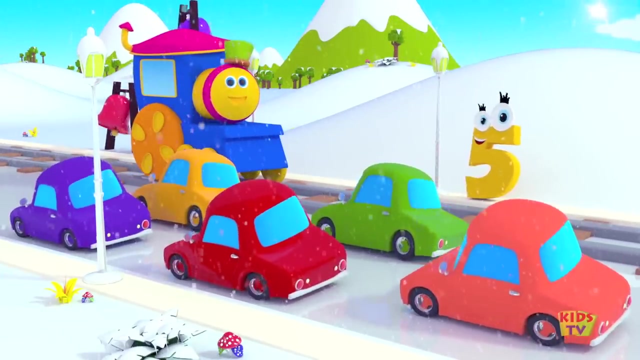 Three old clocks Tick, tock, tick, Tick, tock, tick. Three old clocks. Four, Four big bells, Ding dong ding, Ding, dong ding. Four big bells. Five, Five new cars: Beep, beep, beep, Beep, beep, beep. 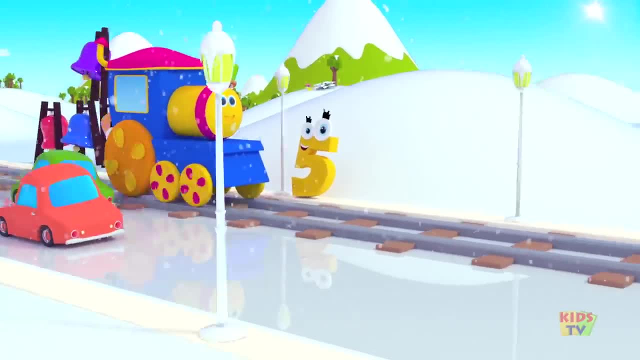 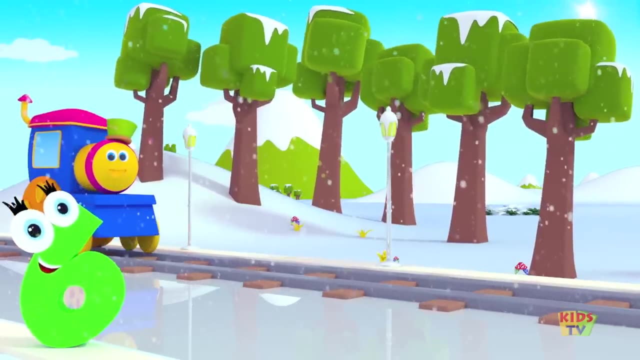 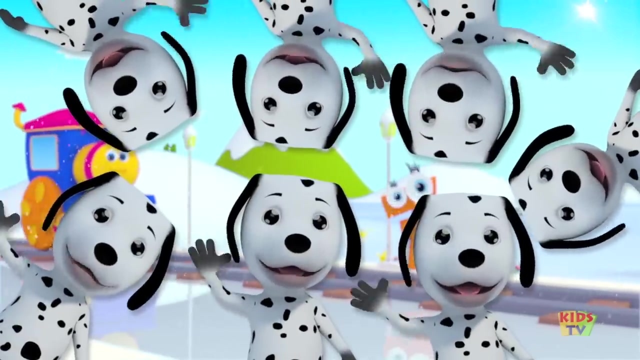 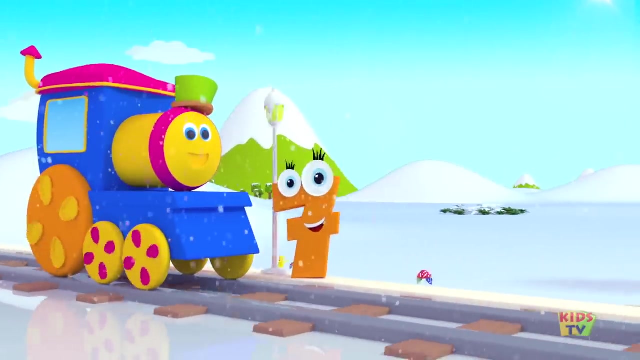 Five new cars. Six Six tall trees, Swish, swish, swish, Swish, swish, swish. Six tall trees. Seven, Seven naughty dogs. Woof, woof, woof, Woof, woof, woof. Seven naughty dogs. Eight Eight noisy drums. 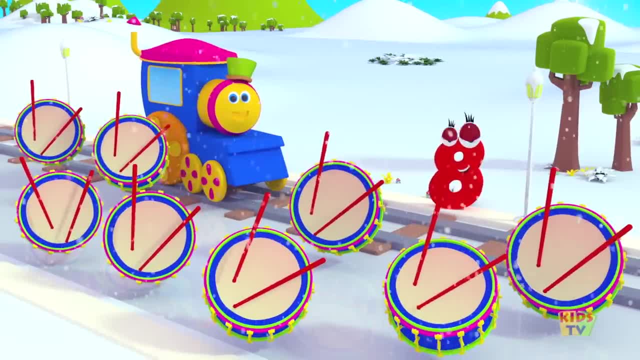 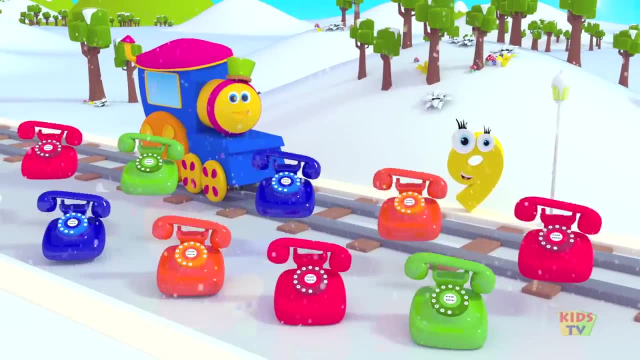 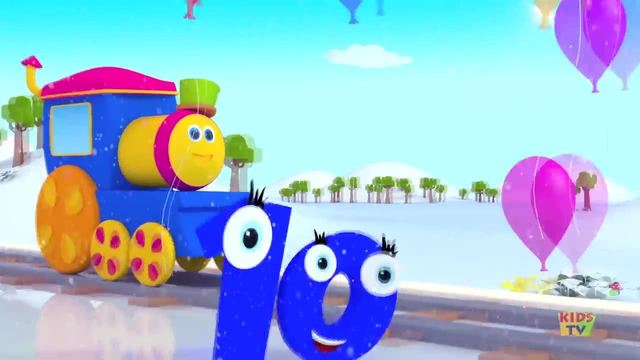 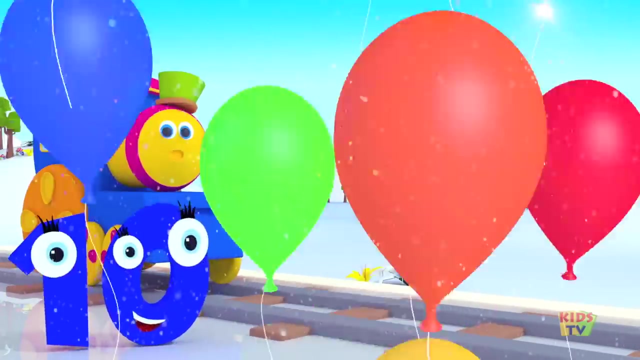 Bang, bang, bang, Bang, bang bang. Eight noisy drums. Nine, Nine ringing phones. Tring tring, tring, Tring, tring, tring, Nine ringing phones. Ten, Ten pretty balloons. Pop, pop, pop, Pop, pop, pop, Ten pretty balloons. 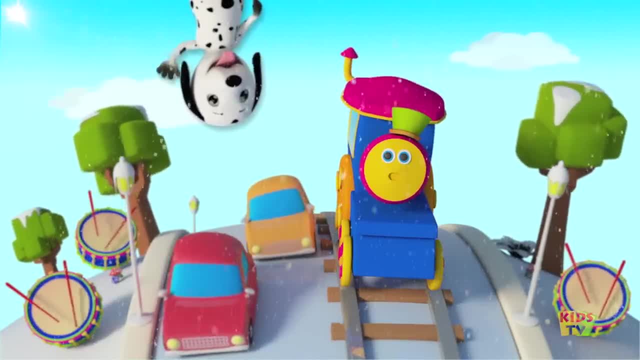 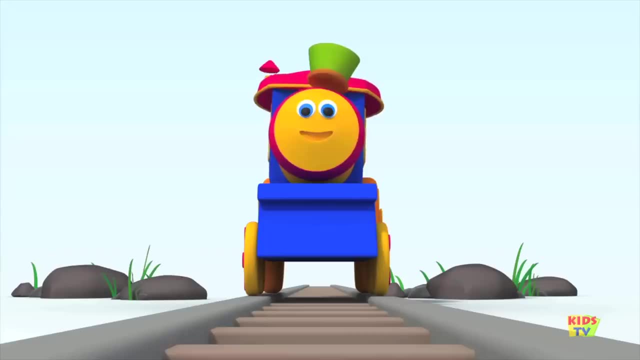 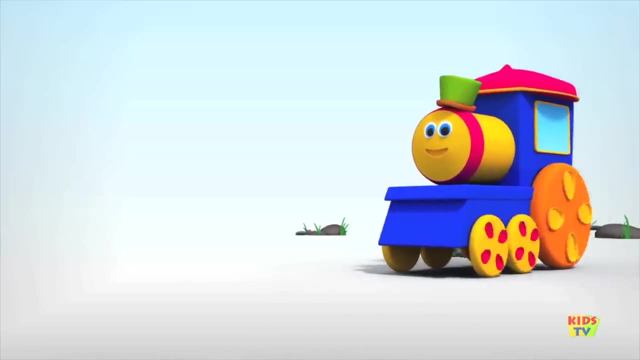 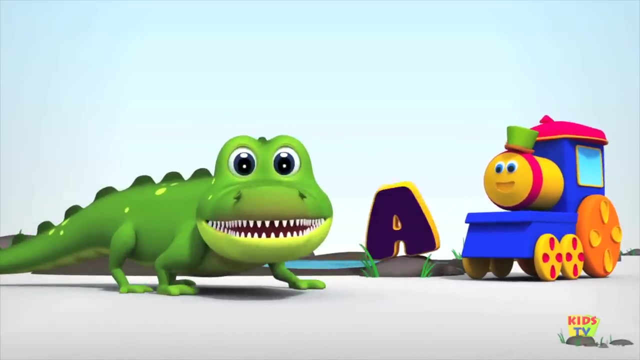 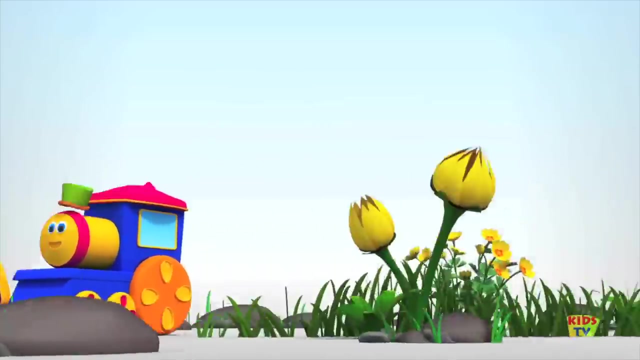 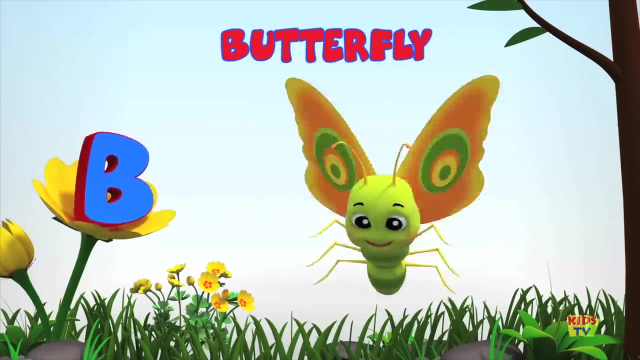 That sure was fun. You can come back anytime for the numbers counting ride. A, a, a alligator, He's so big and green. B, b, b, a butterfly, She's pretty like a queen. C, c, c, a caterpillar. 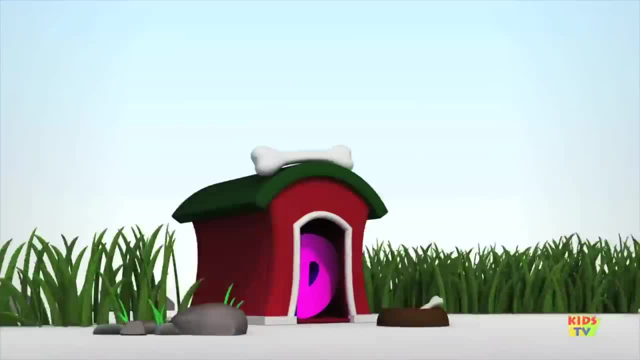 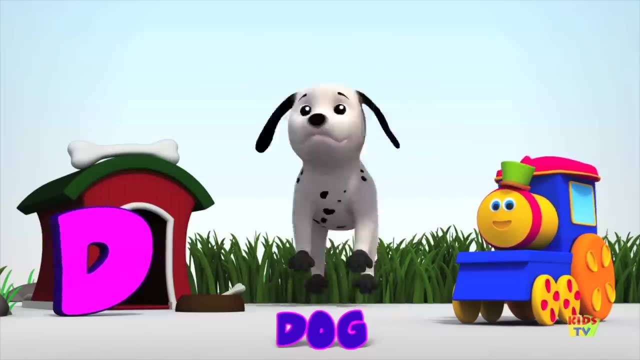 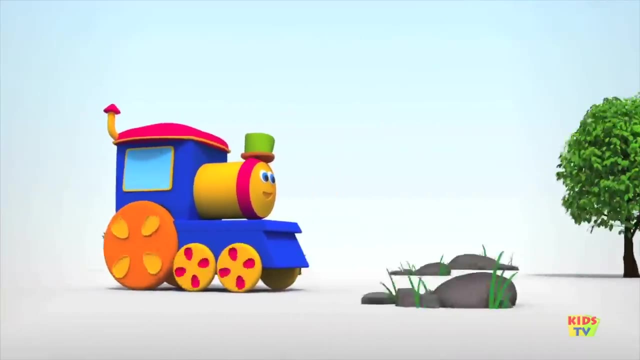 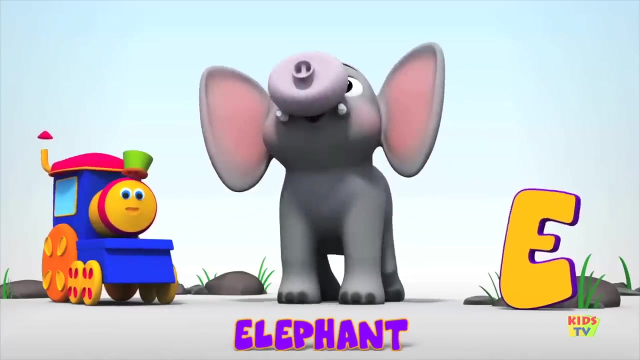 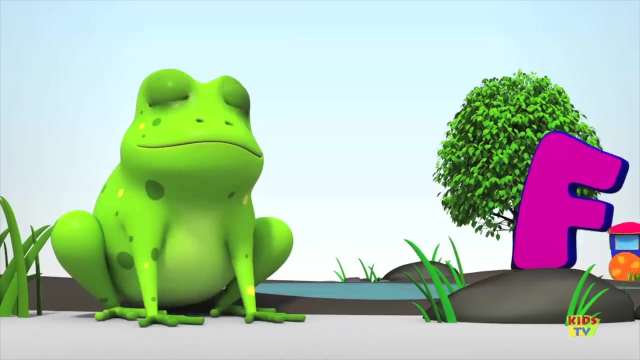 Oh, how slow it crawls. D, d, d, a dog, Look at him, hop on his paws. E, e, e, an elephant. His trunk goes on and on. F, f, f, A frog, His tongue sticks out so long. G, g, g. 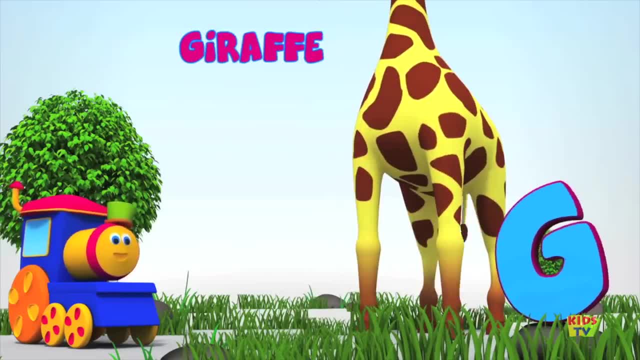 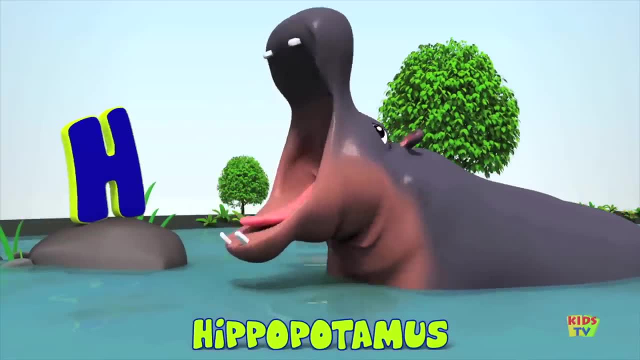 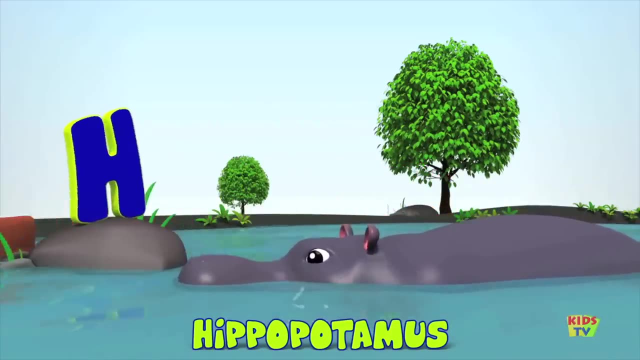 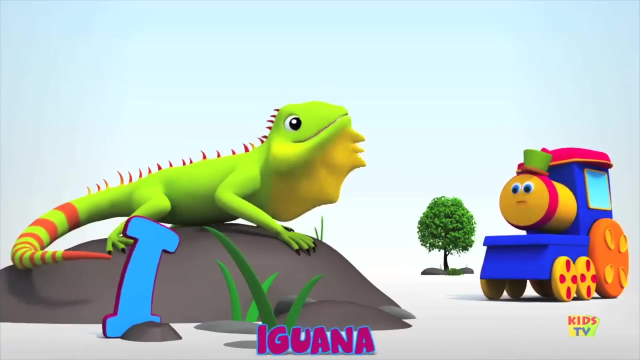 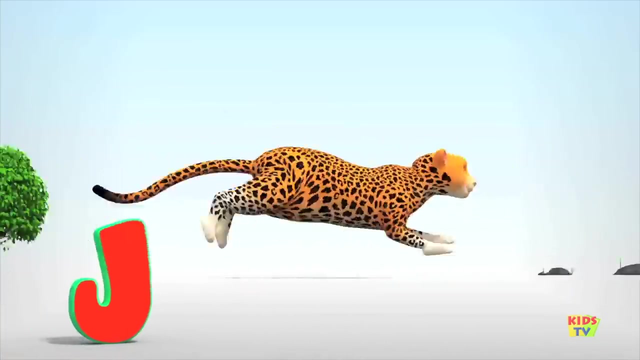 Giraffe. I can only see him halfway. H h, h, A hippopotamus. She can lie in the river all day. I, i, i an iguana. It looks like a little dinosaur. J j j a jaguar. He's got a thousand spots and more. 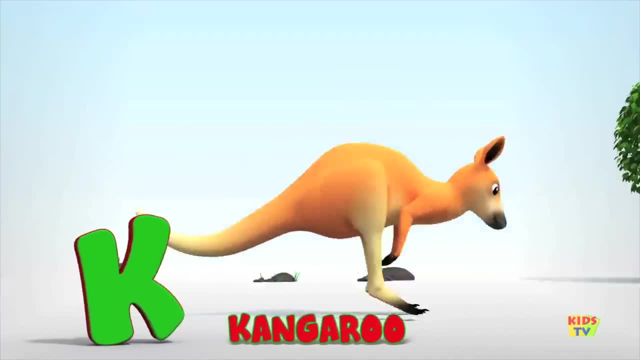 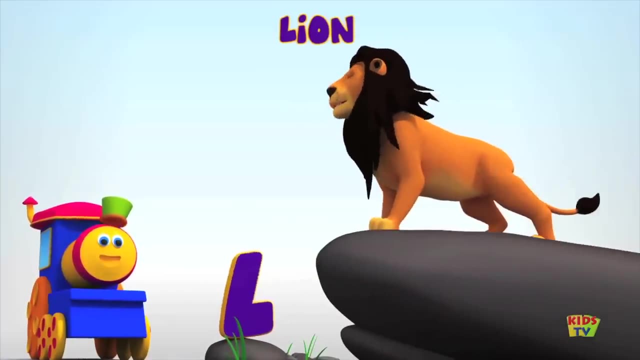 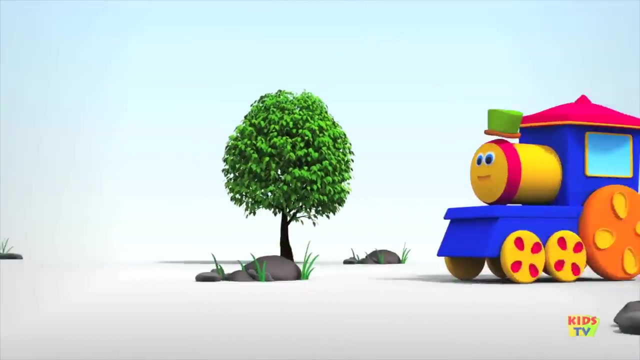 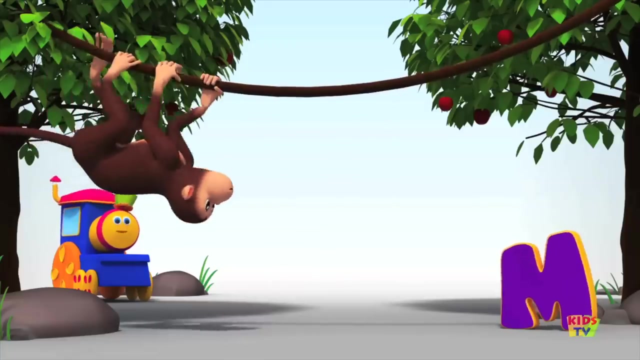 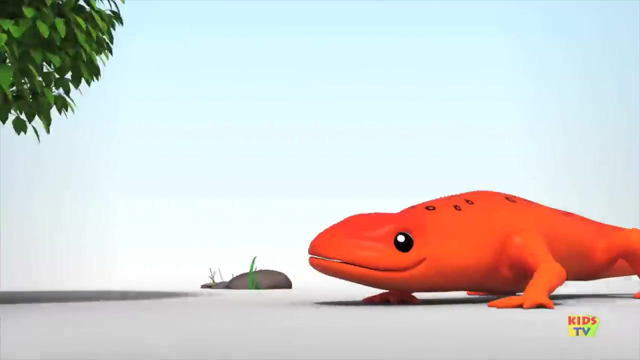 K k k a kangaroo. Look at him, hop around. L? l l a lion, King of the jungle. he's crowned M m m a monkey. Doesn't he love the trees? N n n a newt. 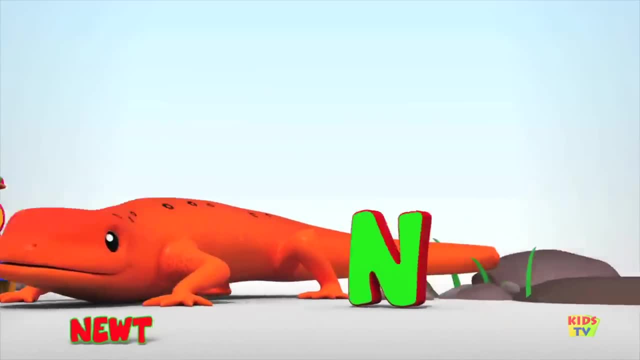 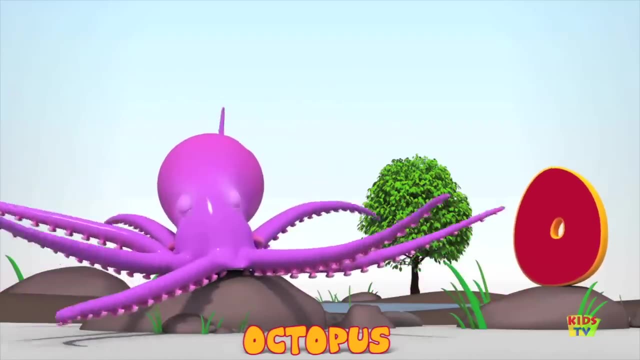 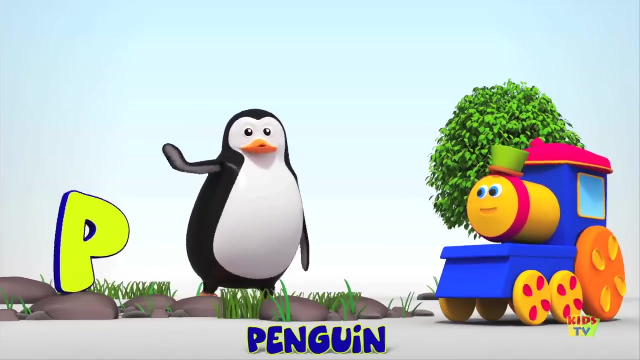 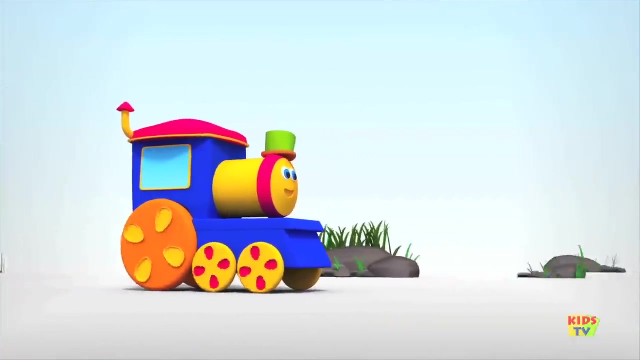 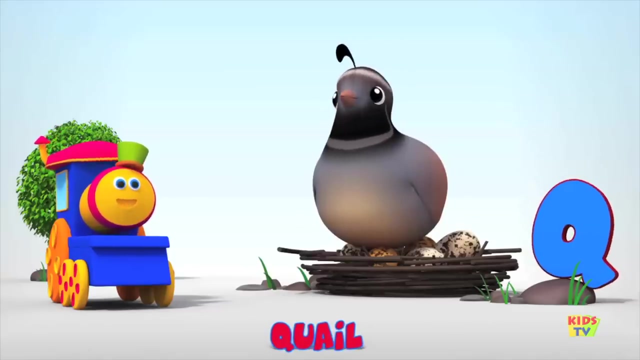 Careful, she's going to sneeze. O o o. an octopus. She sure got a handful of arms. P p, p. a penguin. Isn't it funny how he walks Q, q, q a quail. 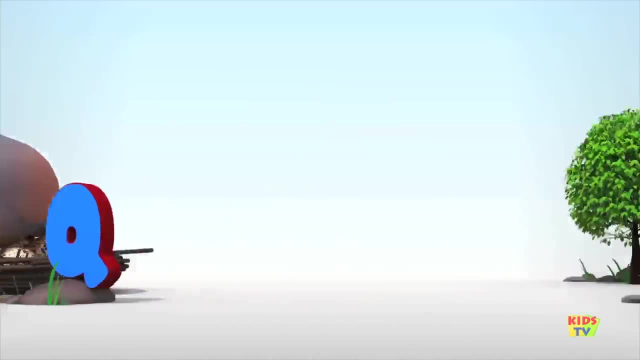 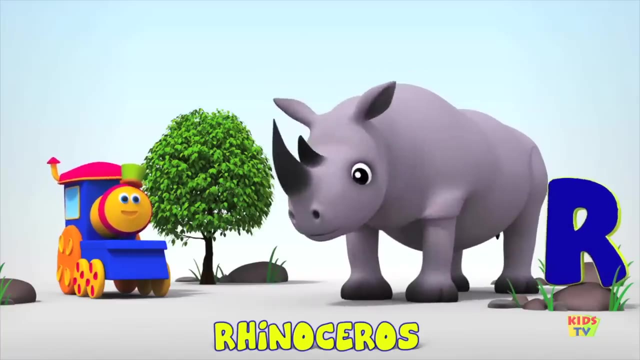 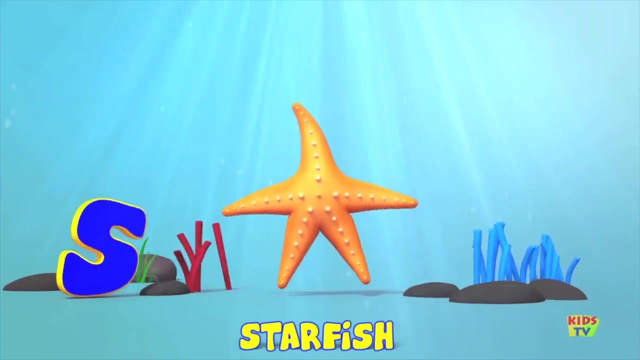 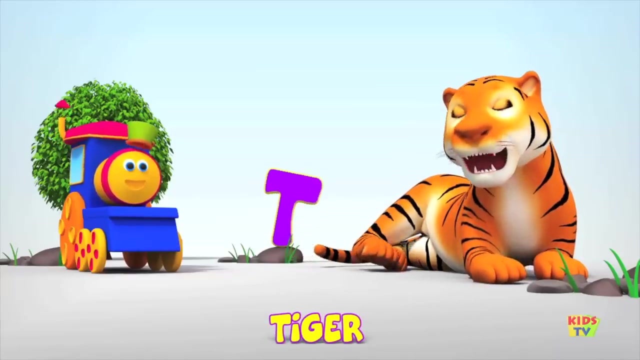 Those are eggs. she's sitting on R r r a rhinoceros. We better be careful of that horn S s s a starfish. She can only be found in the sea. T t t a tiger. I think this one's feeling sleepy. 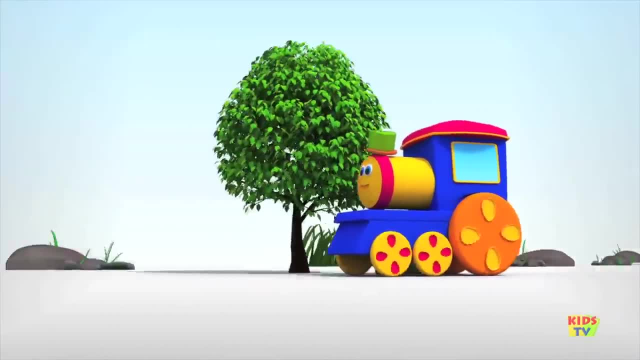 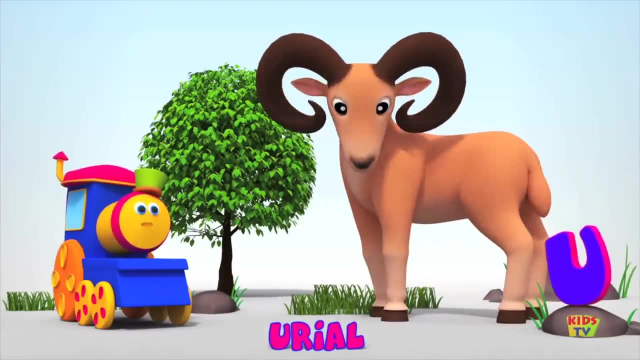 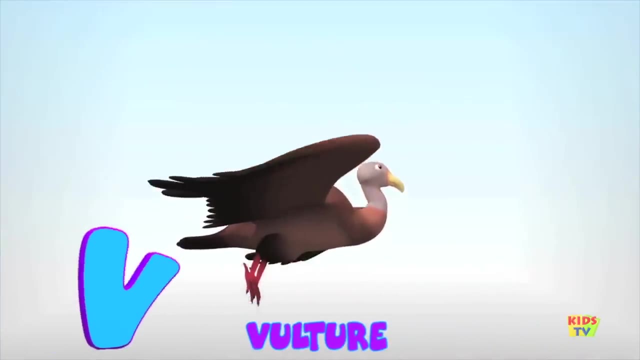 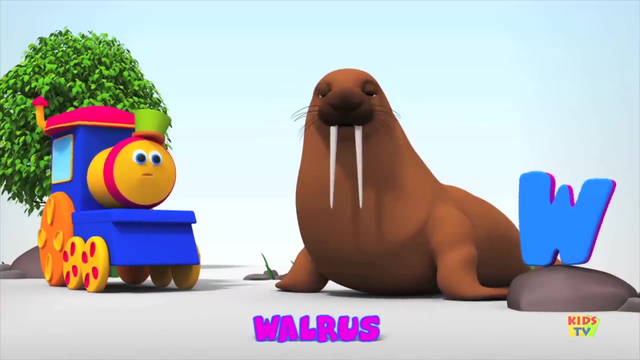 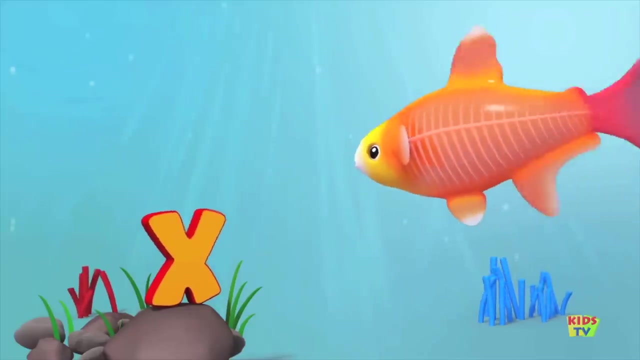 U u u a Uriel Its horns, do catch your eyes. V v v a vulture. She can fly so high in the skies W w a walrus. I wonder how its teeth grew. X x x. an x-ray fish. 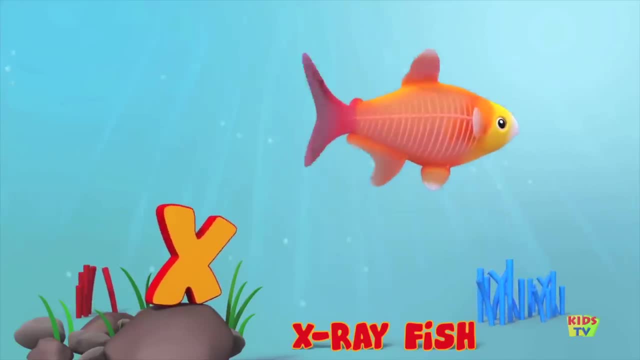 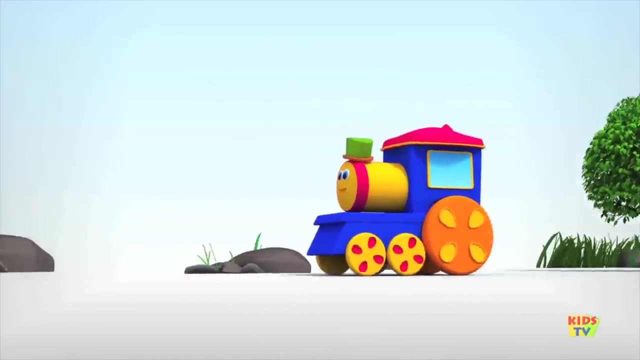 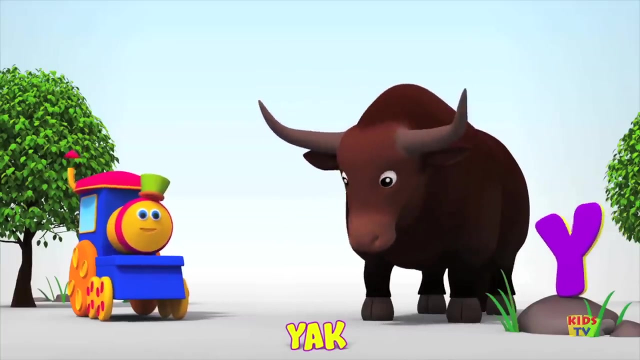 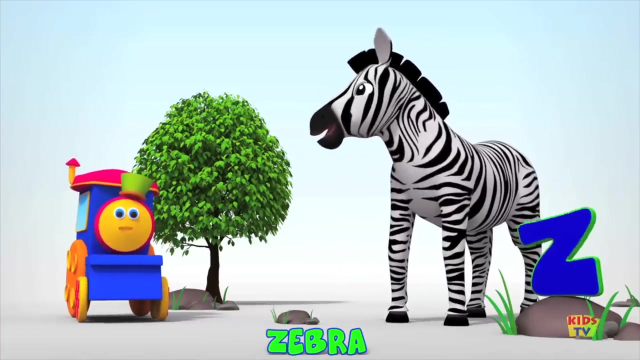 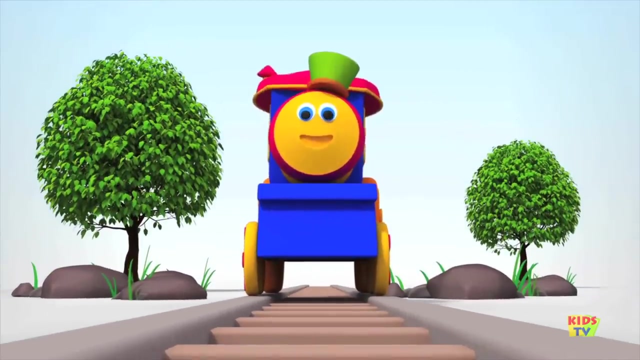 You can almost see right through Y y y a yak. I think she feels very cold. Z z z a zebra. He looks like a striped horse. That was the Animals ABC song, Wasn't it fun? Then come back soon with Bob the Train. 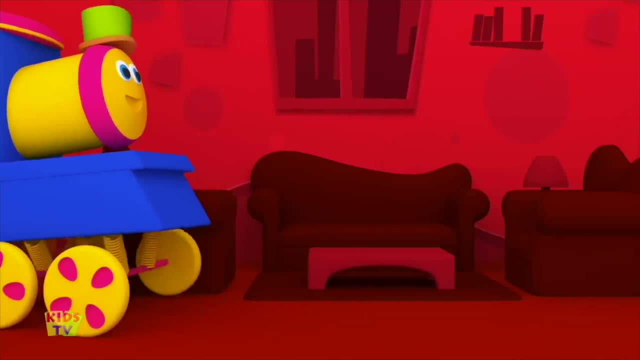 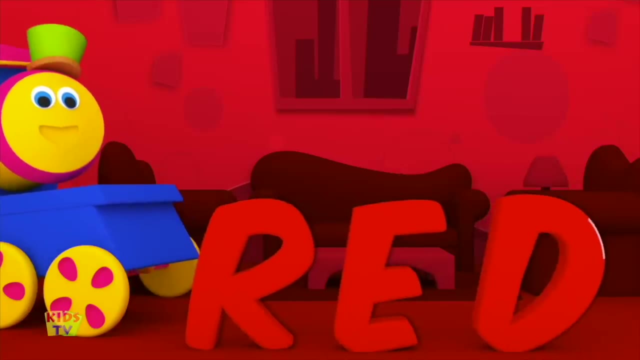 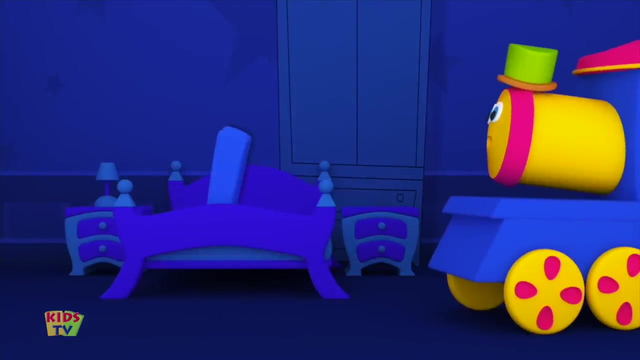 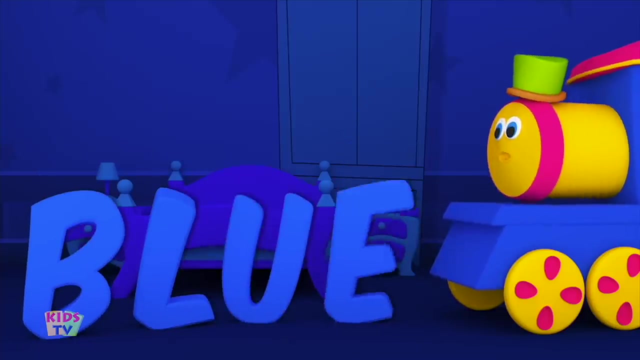 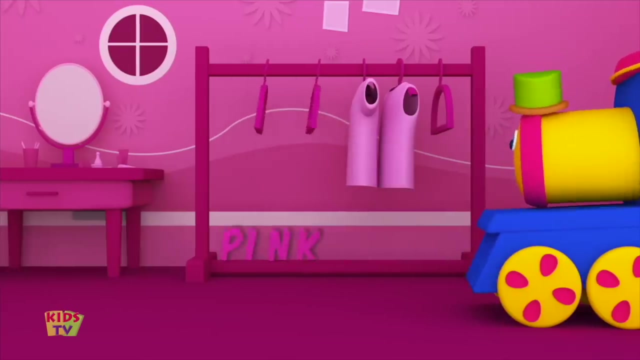 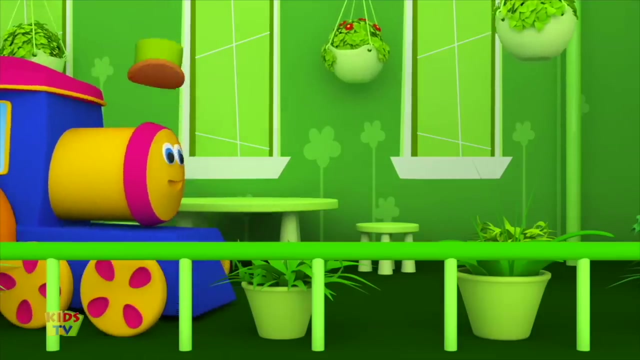 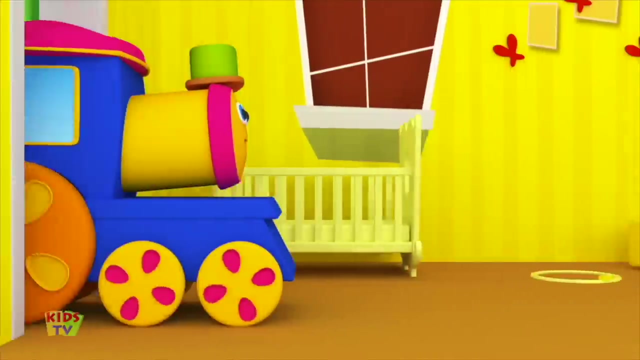 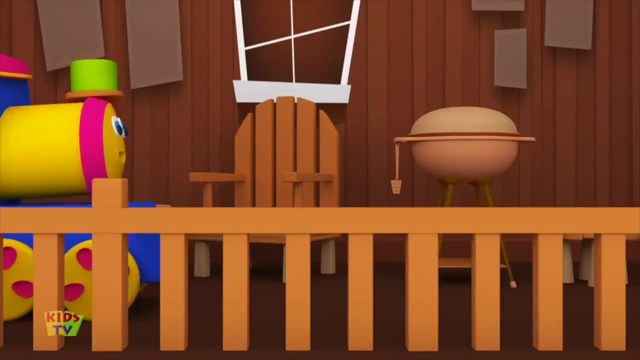 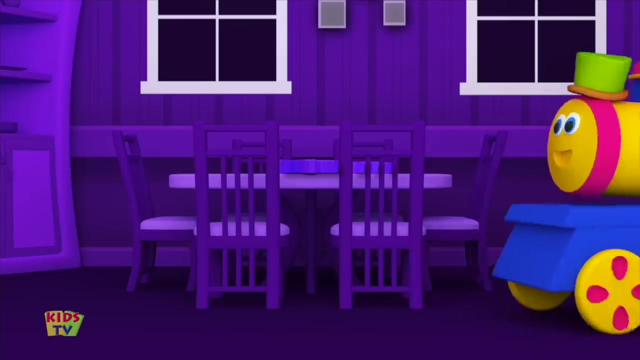 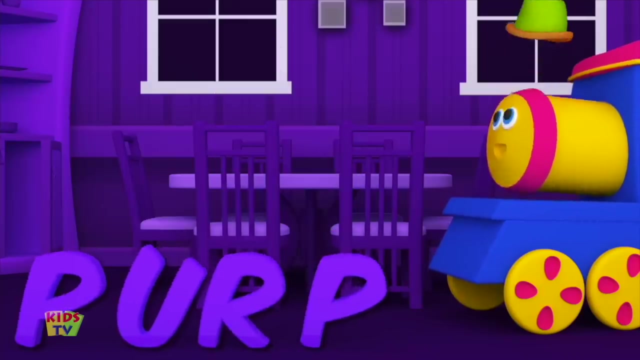 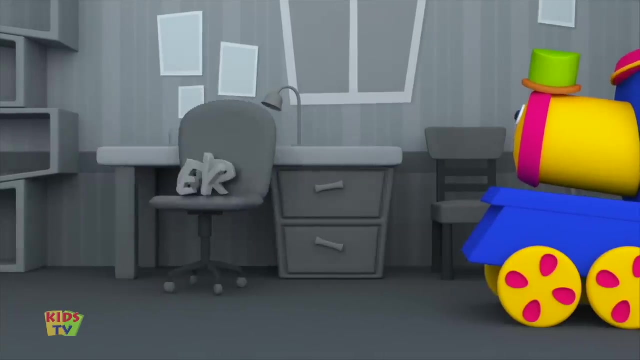 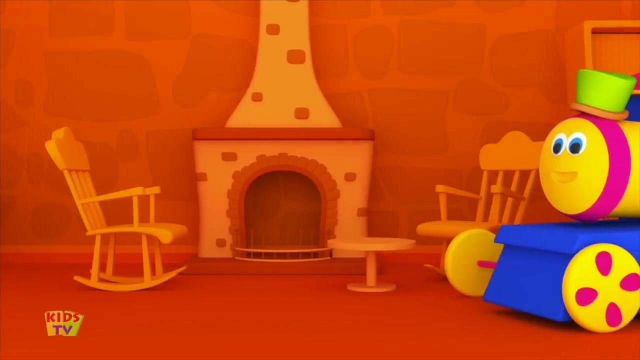 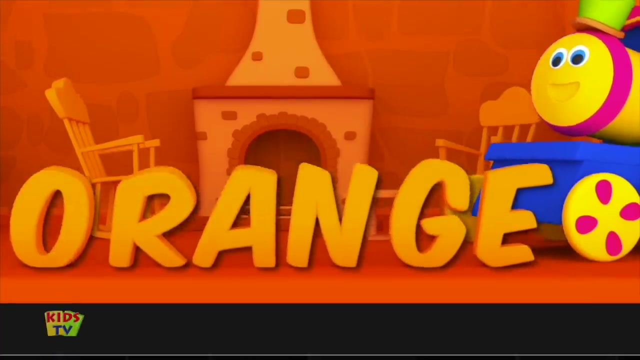 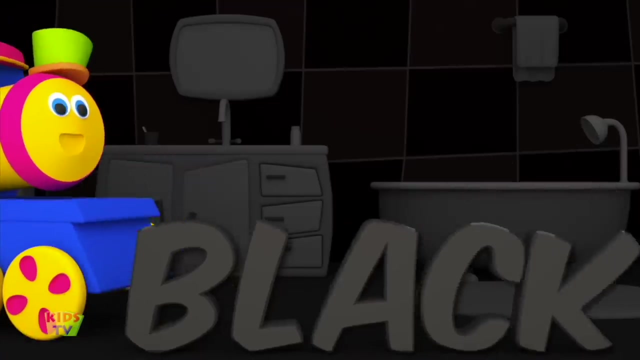 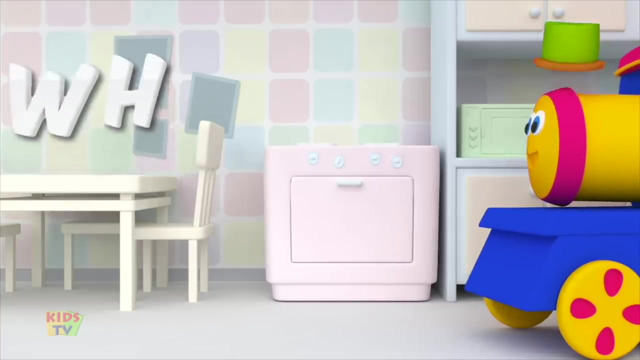 Red, Red, Blue, Blue, Blue, Blue, Pink, Pink, Pink, Pink, Pink, Green, Green, Yellow, Yellow, Yellow, Yellow, Brown, Brown, Blue, Blue, Blue, Blue, Blue, Purple, Purple, Blue, Blue, Gray, Gray, Orange, Orange, Orange, Orange, Black, Yellow, Red, Blue, Red, Black, Black, Yellow, Red, Green, White, Yellow, Blue, Yellow, Blue, Black, Blue. 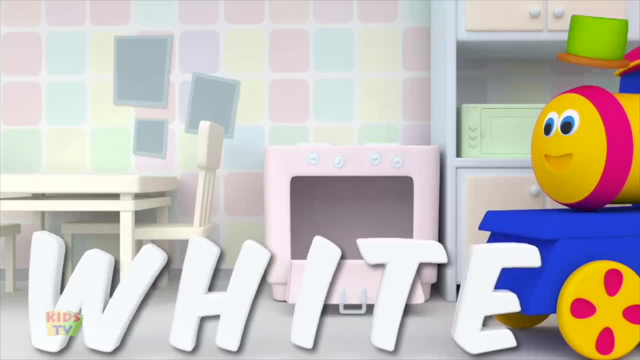 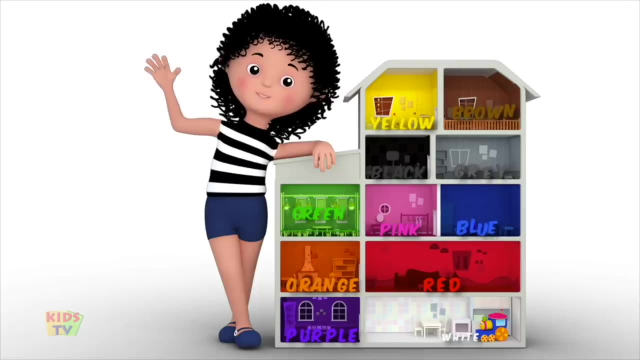 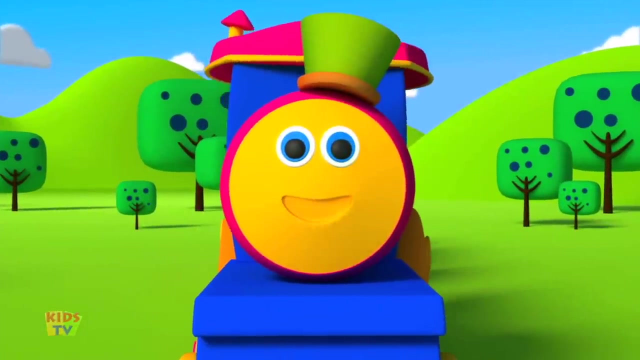 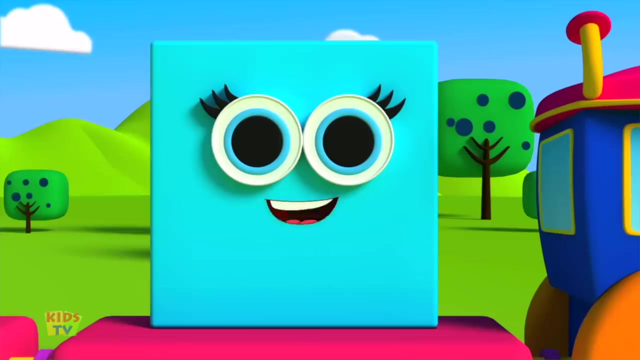 Blue, White, Red, White, White, Blue, Yellow, Blue, Red, White, Blue, Blue. Hi, kids, how are you doing today? Let's all get ready, because today we're going to play With colorful shapes and have lots of fun. Let all shapes introduce themselves, one by one. Square is my name. my four sides are just the same. 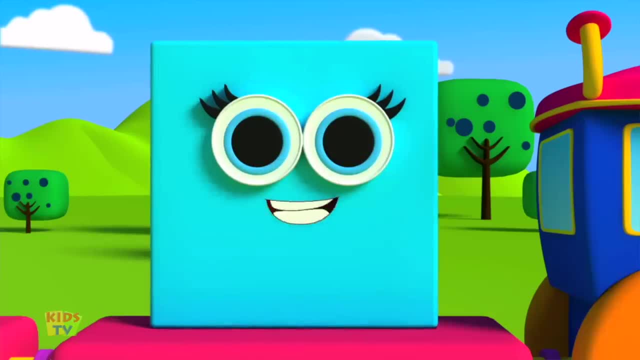 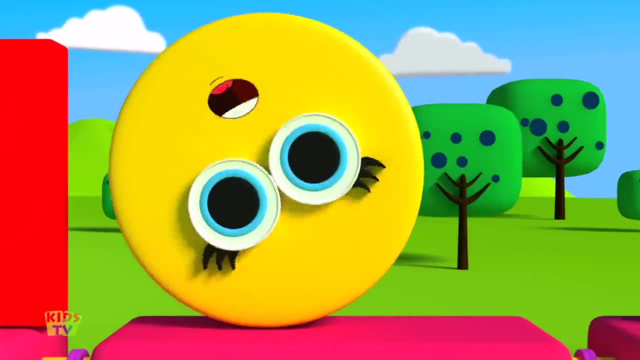 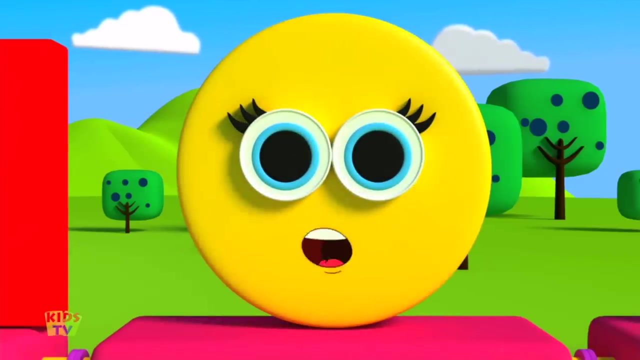 Turn me around, I don't care, I'm always the same. I'm a square. Circle is my name. watch me turn round and round And soon you will learn my outside edges never end. I'm a circle. I'm a circle. Rectangle is my name. my four sides are not the same. 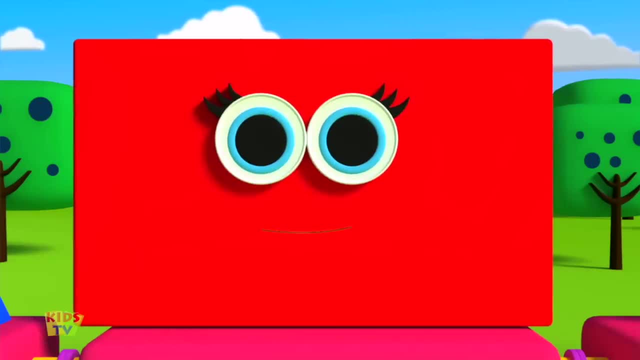 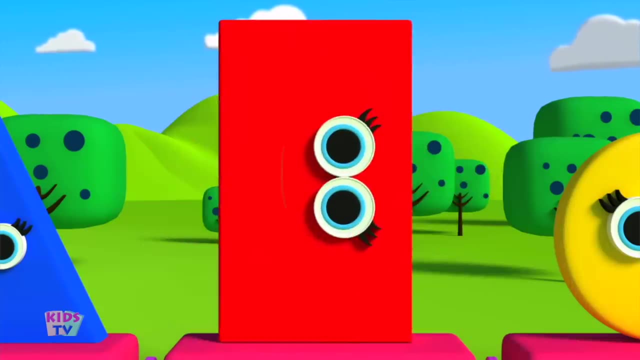 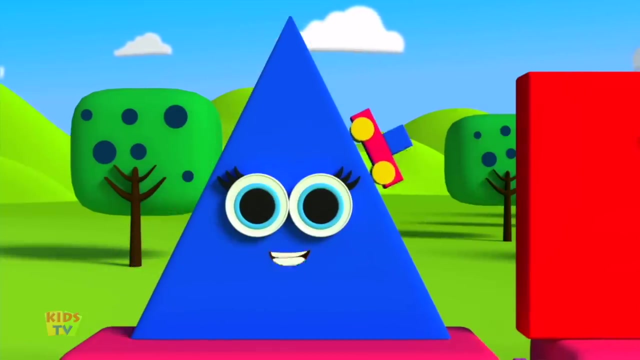 Two are short and two are long. Count my sides and come along. One, two, three, four, Four, Four, Four- Triangle is my name- up the hill and to the top Down the hill, and then you stop Straight across, tell me what you've got. 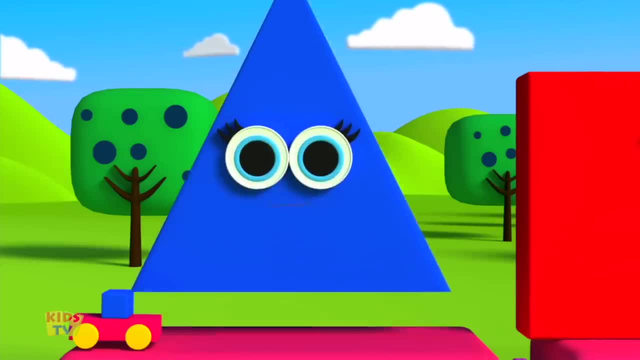 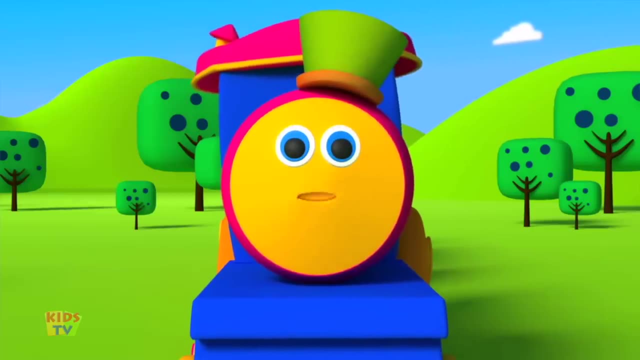 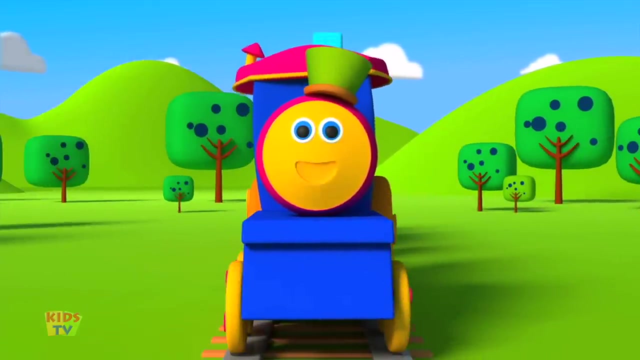 A triangle. yes, I'm a triangle. Okay, kids, now let's go Play with shapes and build something more. Now let's show our wonderful skills: A beautiful house of shapes we will build. My name is triangle. My four sides are the same. What's my name? 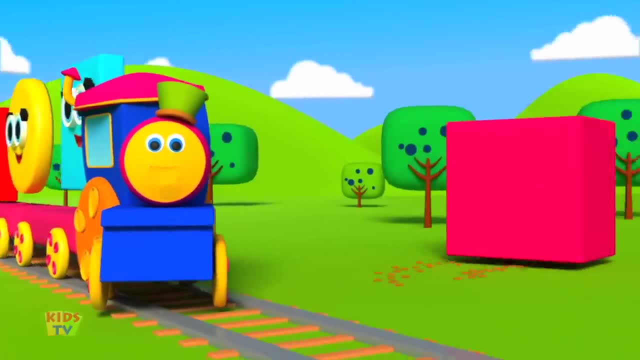 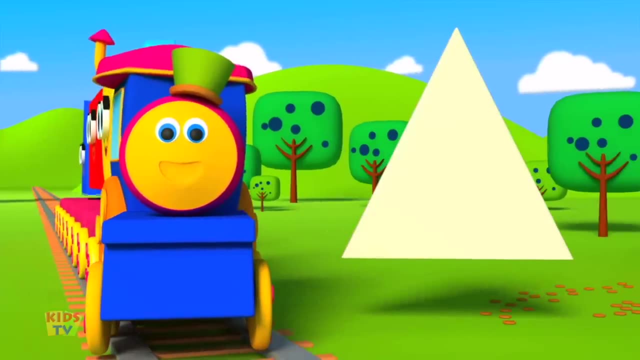 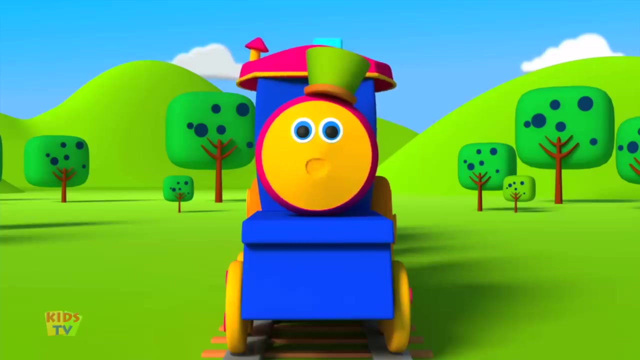 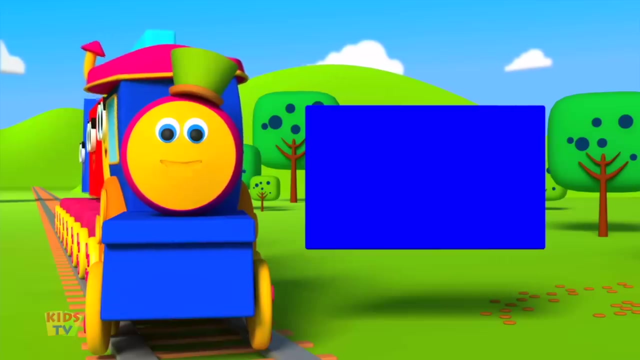 Square? Yes, let's put it there. Now. look aloof and tell me the shape of a roof Triangle: Yes, let's place it at a perfect angle. We're going strong. Now name me a shape with four sides: Too short, too long? Rectangle: Yes, a rectangle it is. 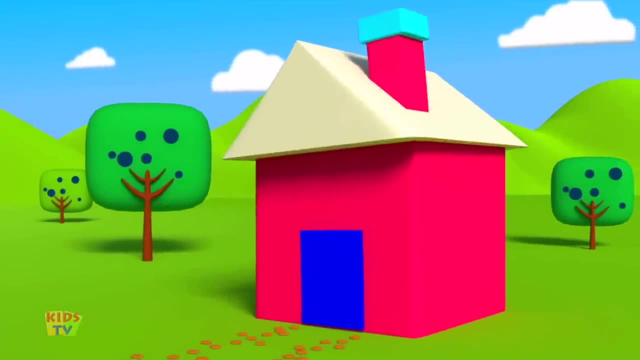 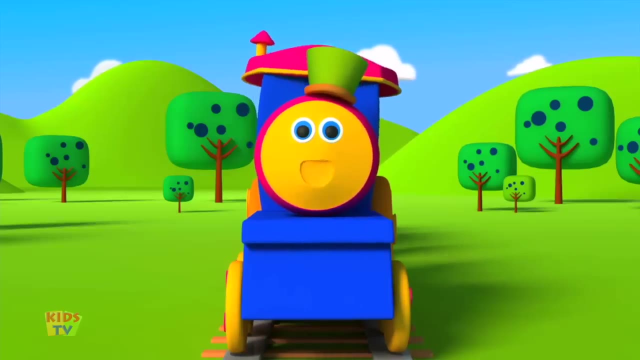 Rectangle, And such a beautiful house we have built, Yes. Well, that was fun. Now let's make another one. We might want to go someplace far. So let's all of us build a car. Yes, Which shape? goes round and round with no end, Can you tell? 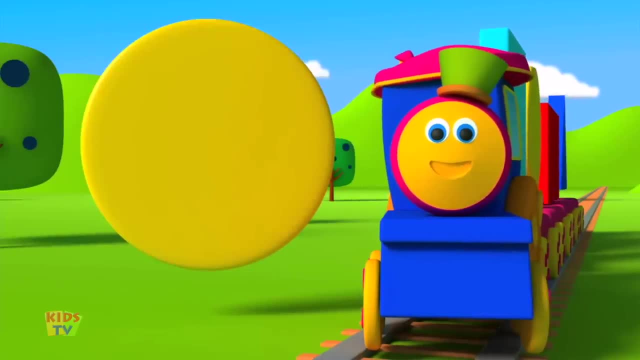 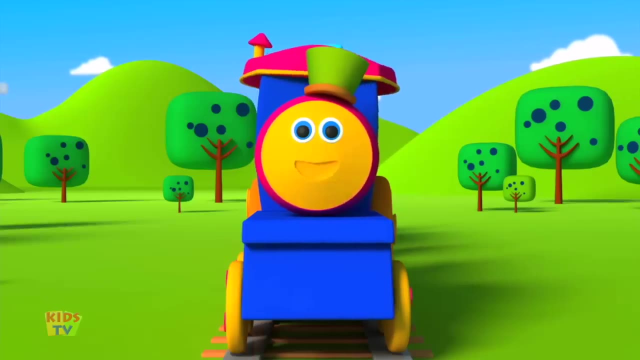 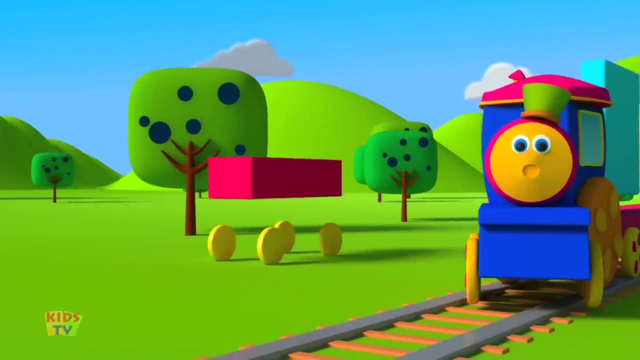 A circle? Yes, a circle it is. Let's place it like this: A shape with two long sides And two short sides. We need for our ride Rectangle. Yes, it's a rectangle, And let's place it so. Which shape with four equal sides Shall we place on the top? 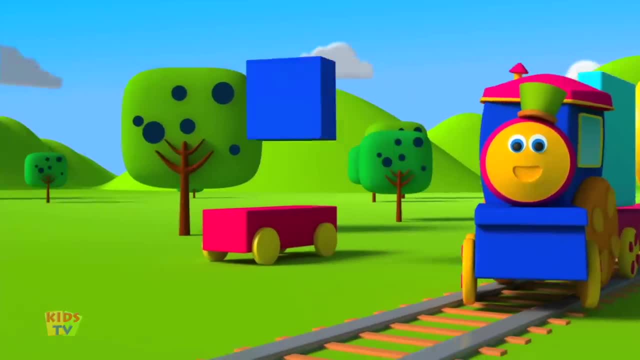 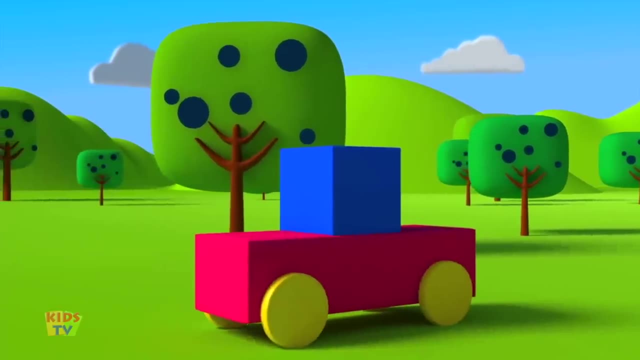 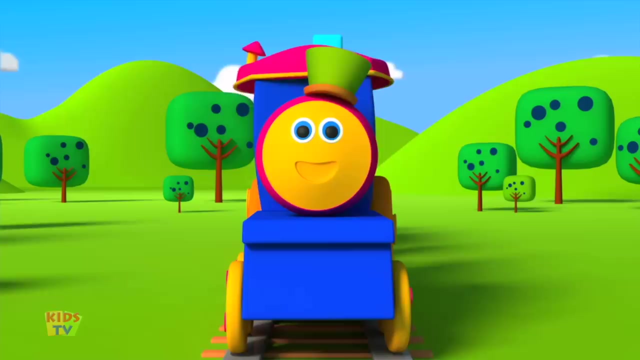 A square. Yes, it's a square In place. let it drop, Using all the shapes. A wonderful car we have made. Yay For resting. let's make a tree. Let's make a tree. Why, kids, don't you agree? Yes, Let's start with a rectangle this time. 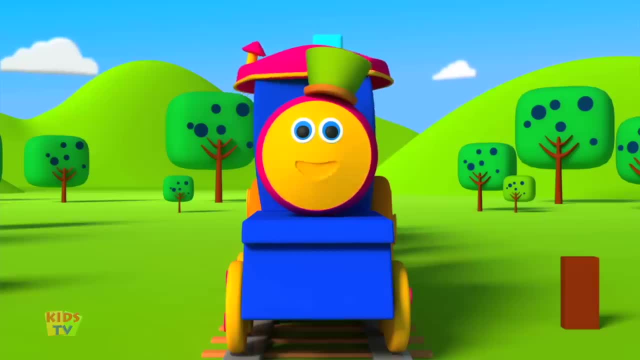 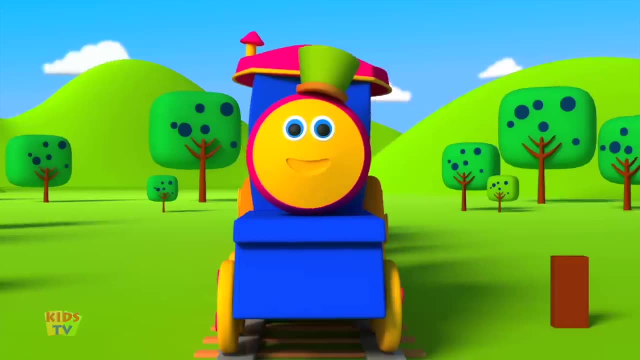 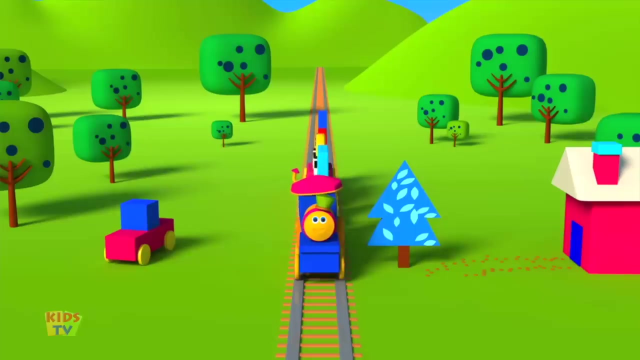 Now doesn't that look fine. Which other shape should we use? Circle, rectangle, please tell us. Okay, some triangles we shall choose. Wow, that looks like a beautiful tree, Kids, don't you agree? Yes, Kids, now let's make a tree. 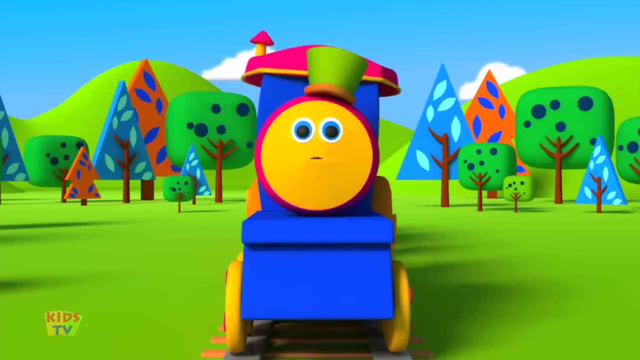 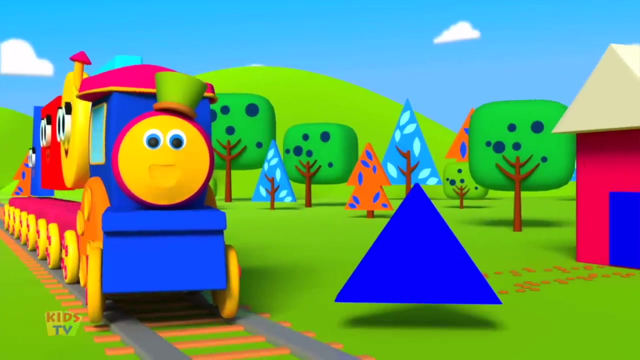 Let's build something more. How about a pretty little seesaw? Yes, on a seesaw we can play all day. Okay, which shape should we start with now? A triangle will be perfect for our seesaw. Now we need a shape with two sides short and two sides long. 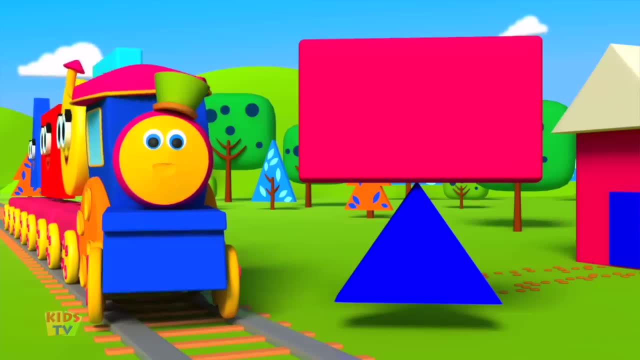 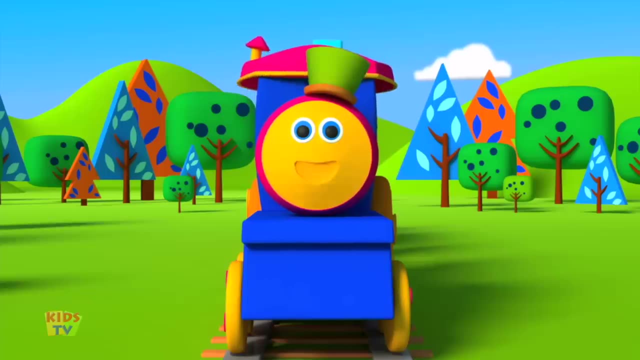 Yes, let's build a rectangle along. Now let's gently place it down. Look, we have made a seesaw on our own. I'm having so much fun today. Seesaw, hooray, hooray. We need to sit and eat somewhere. 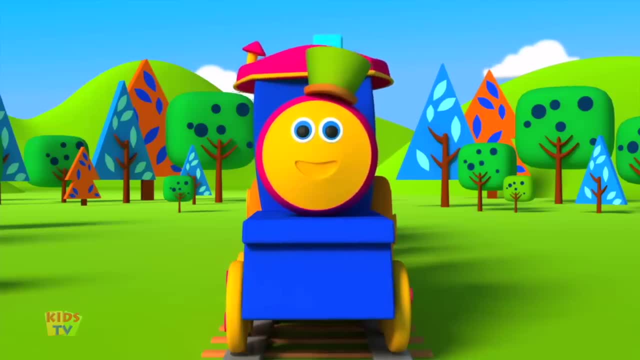 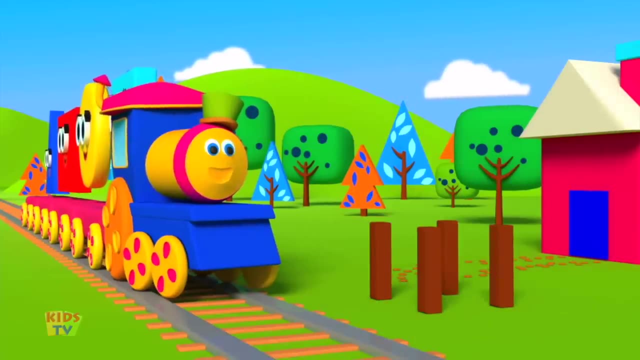 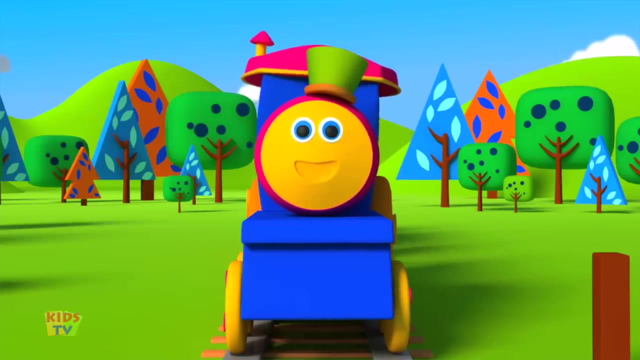 Let's build a table and some chairs. We'll use four rectangles for the legs. Let's place them all at this angle. That looks great. Thank you, rectangle. Now let's take a shape that's round Kids. can you tell me where that can be found? 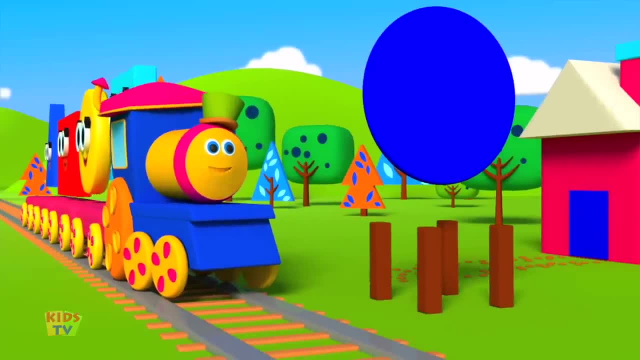 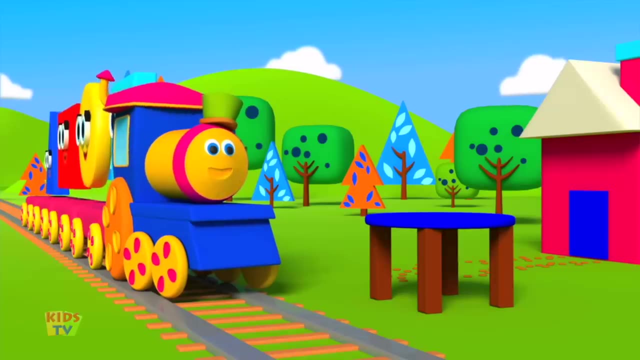 A circle. Yes, it's a circle. Let's place it on the top. There's our lovely table, Even prettier than from a shop. Now let's call squares and rectangles to build our chairs. That looks wonderful. Now we can all sit somewhere. Thank you, shapes. 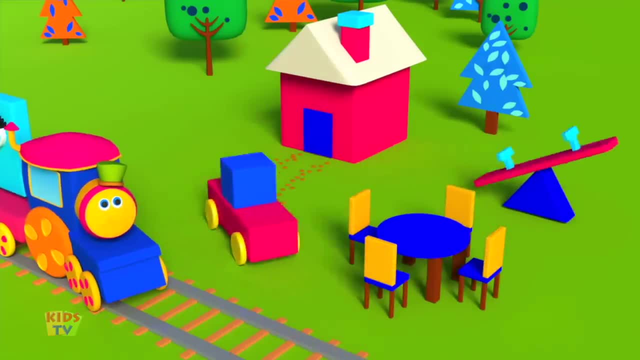 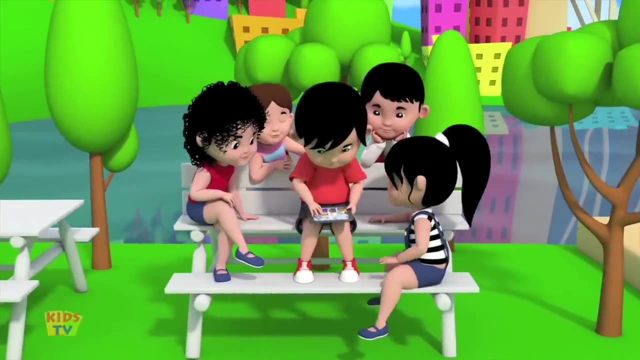 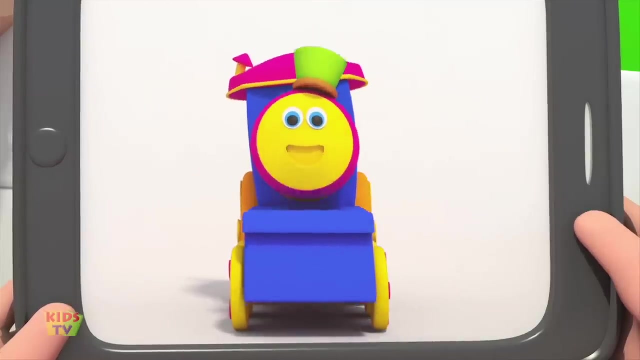 I had so much fun today. See you next time for more fun and play. Hey, kids, good morning to you. Hope you're all doing wonderful. Last week you mentioned the holidays were getting pretty boring. Do you want to go on a treasure hunt involving the alphabet? 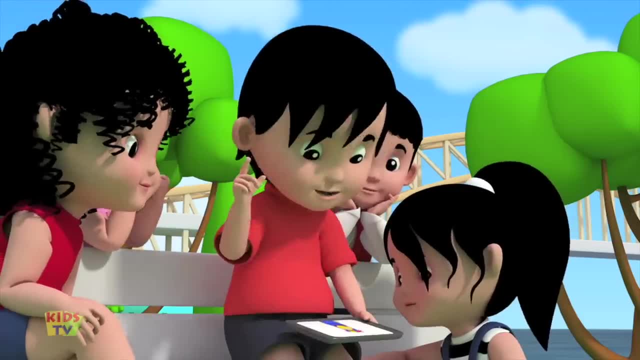 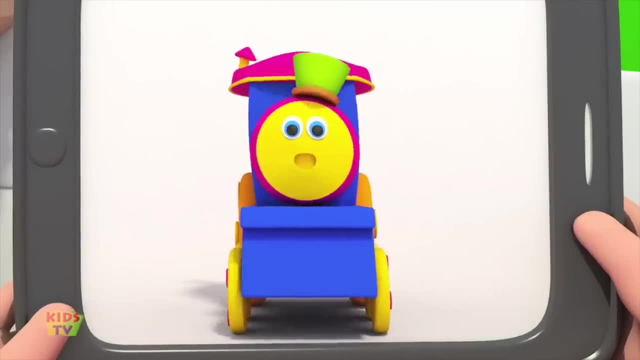 An alphabet adventure. Yay Shh, it isn't over yet. All the 26 letters of the alphabet have gone into hiding. They've left clues, so you know where to look for them. So let's get on with it. You'll find me among sandcastles with a stick for a flag. 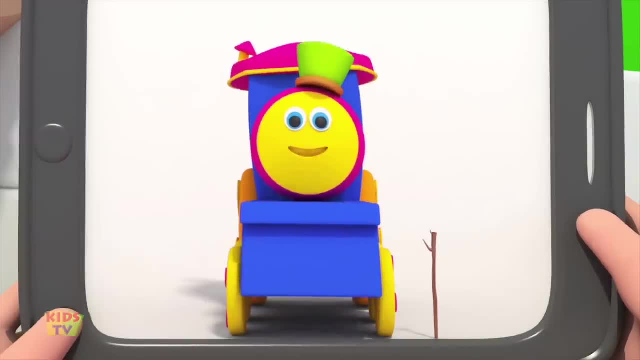 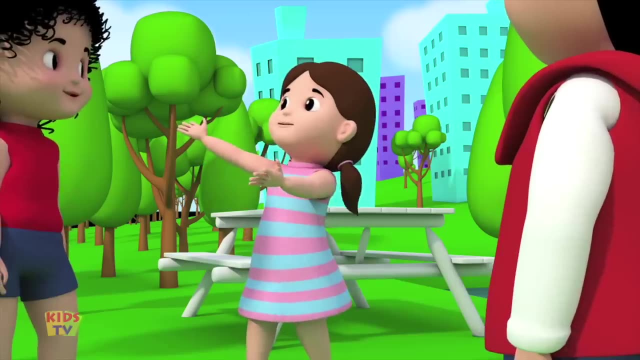 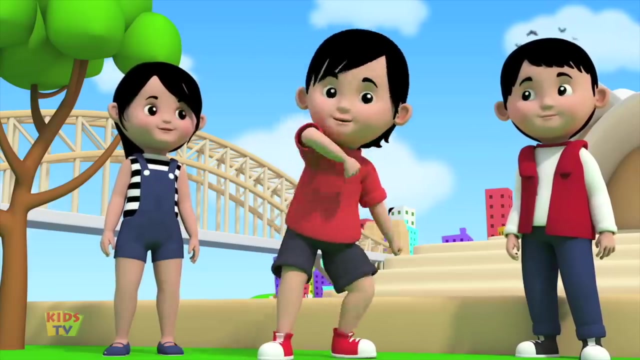 Looking for seashells to put in my bag. Bring a ball, if you must Well count on Bob to make the holidays more exciting. What was Bob saying about sandcastles and shells? That's our first clue. The beach, Absolutely. So let's head there, shall we? 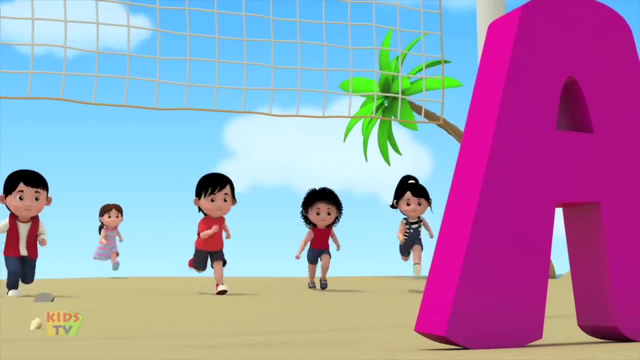 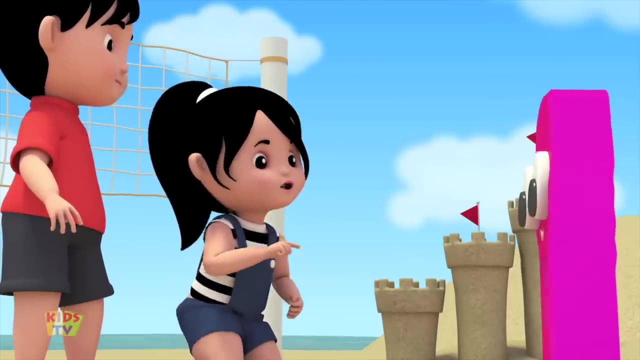 As soon as they reached the beach. they expected to see Bob, But were shocked. But were shocked to see someone else. Hey, we thought all of the letters were in hiding. What are you doing here? Don't tell us. the adventure has been called off because we were looking forward to it. 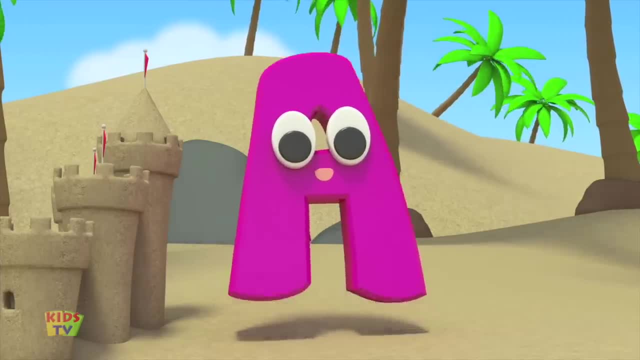 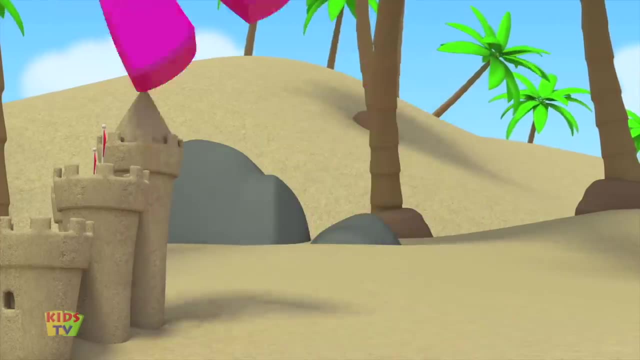 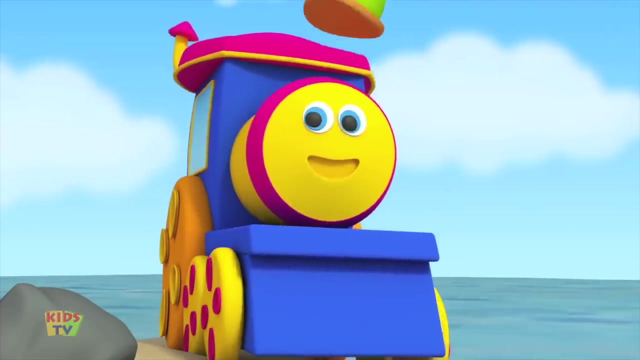 No, no, The treasure hunt is still on, But Bob needed my help with charting out the treasure map and all its clues. So let's go meet Bob. Hey kids, Bob, we missed you. I've missed you kids too, And great job finding me at the beach. 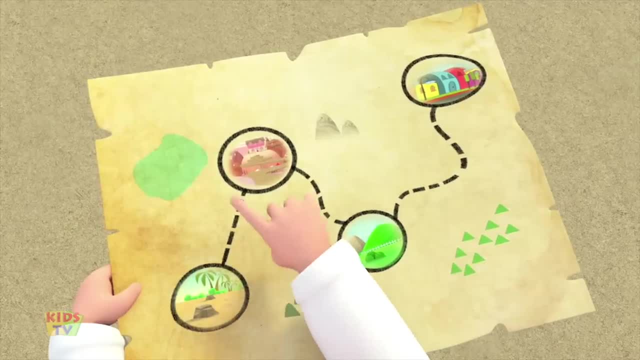 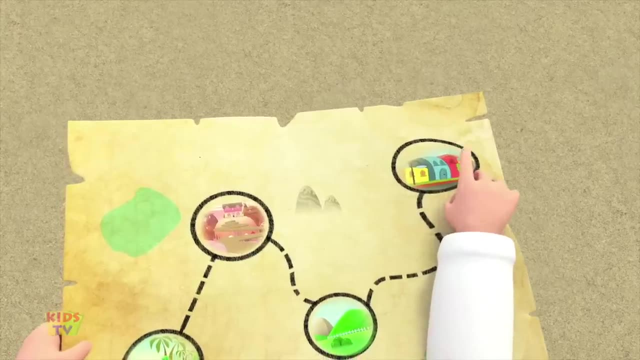 There you go, According to the map. from the beach we have to get to Chocolate Lane, Then to the phonics playground And finally to ABC Land, Where Z will be waiting for us on top of the treasure mountain. We have to find all the other letters on the way. 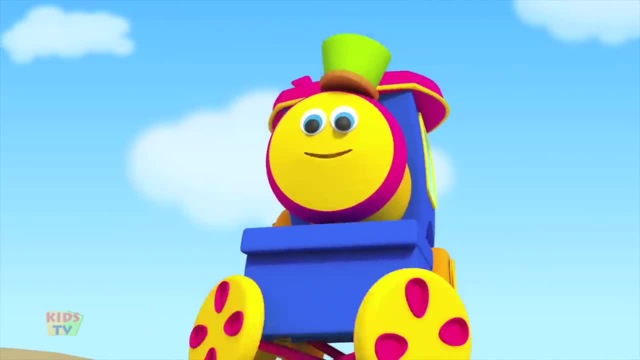 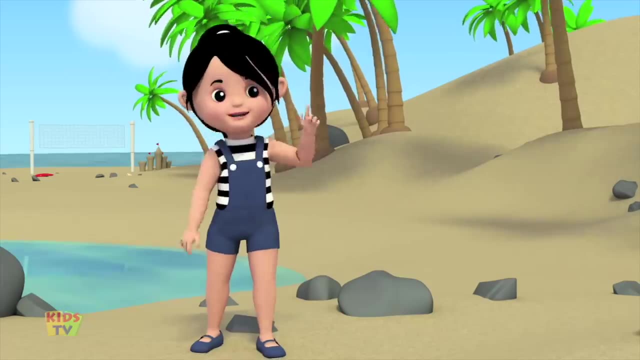 Well, let's get on with it then. In order to find B, you need to name at least three objects beginning with the letter B. Polly, would you like to go first? A boat, and I'd love to steer it. Jack, what would you like to name? 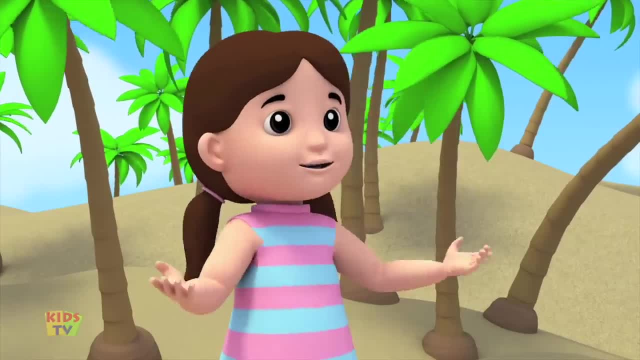 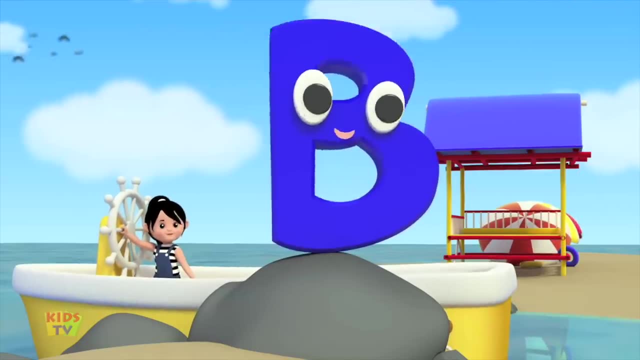 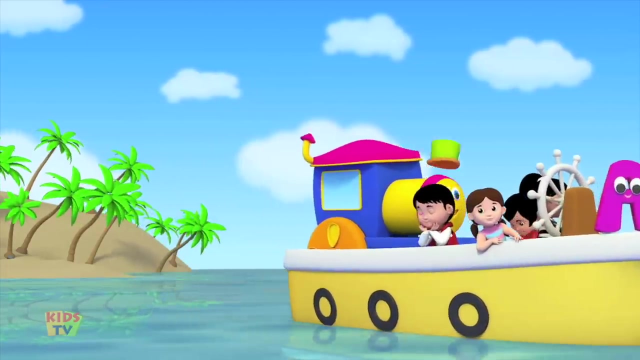 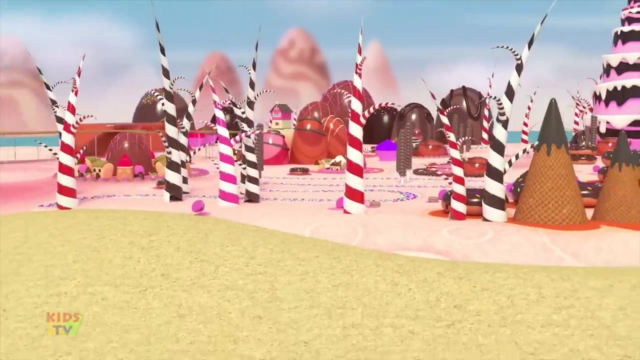 A beach ball. Can I go next, Bob? A balloon. Well, you got that right. Hey kids, great job naming the objects And let's go find the others. Yay, They all cheered and climbed onto the boat and sailed through the chocolate river Soon enough. they were on the shores of Chocolate Lane. 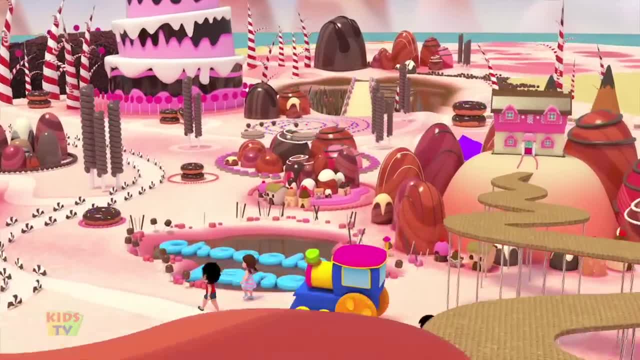 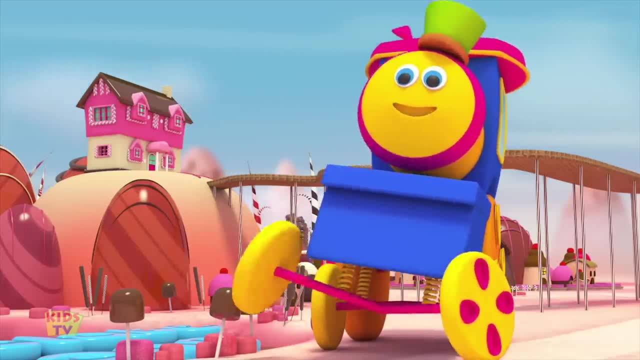 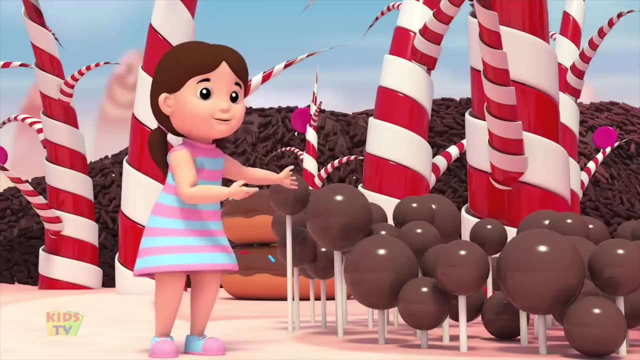 It's so beautiful. Okay, kids, ready for your next clue? Behind something pink and round, the letter C shall be found. Do you think C is hiding behind that bush of lollipops? They're round, But they aren't pink. It has to be round and pink. 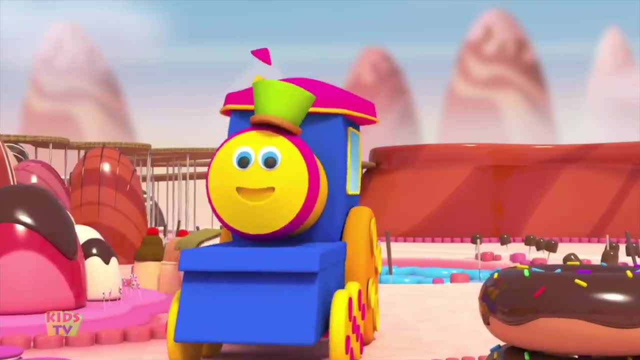 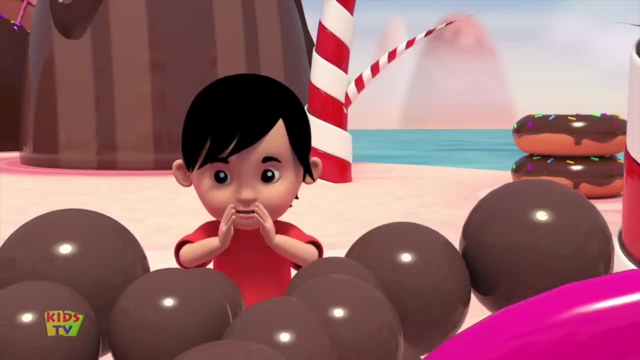 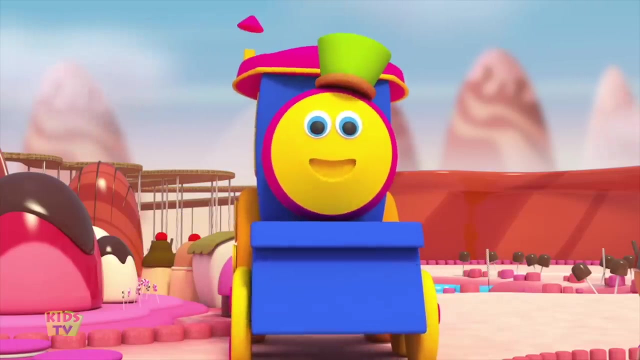 I'll give you a special treat if you can find it. Psst C. are you here? Hey kids, look Johnny's here And there's something on his arm. It's C. Good job, Johnny. Now we have A, B and C. 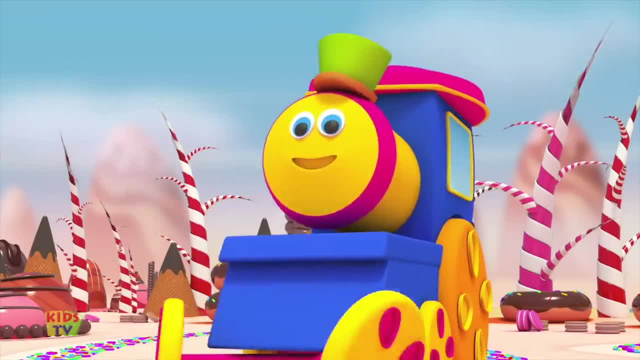 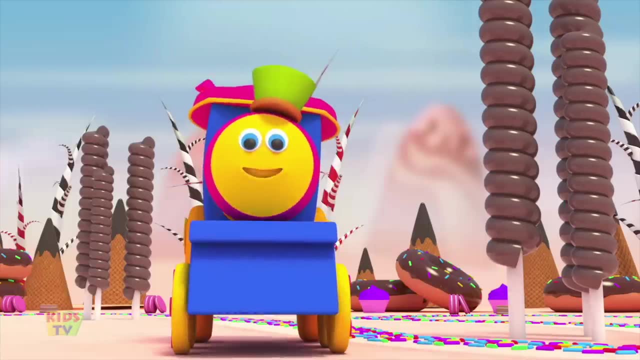 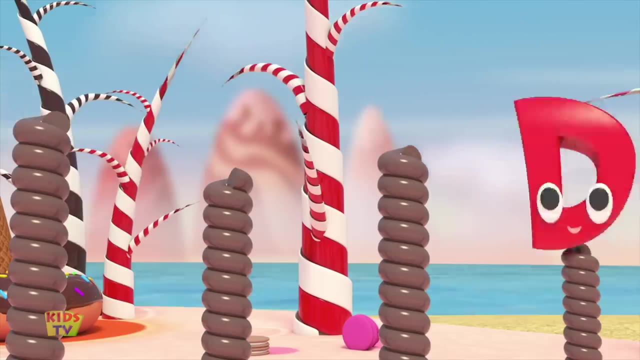 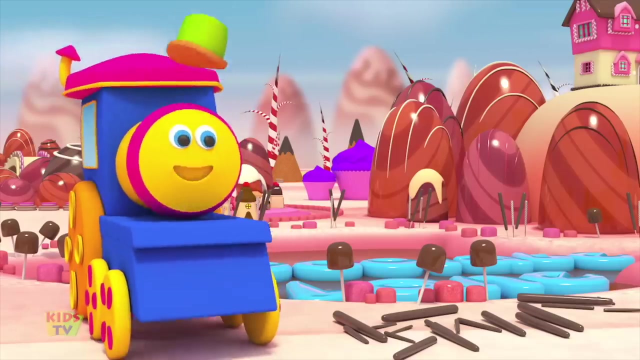 Let's find D Chocolate trees, big and small. Which is the tallest of them all? Find the letter D hiding behind the tallest spiral chocolate tree. Mary, take a guess. Um that one. Yay, You kids are doing absolutely wondersome. We've kept a few chocolate sticks of different shapes and sizes. 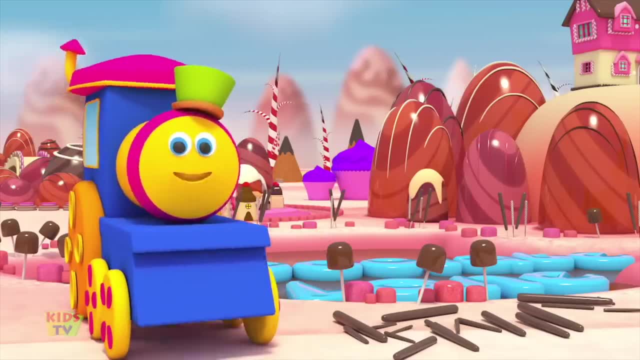 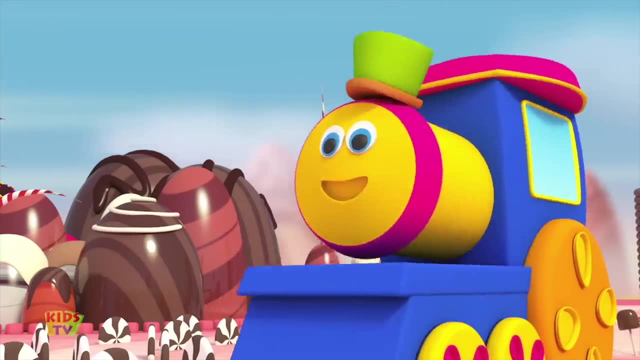 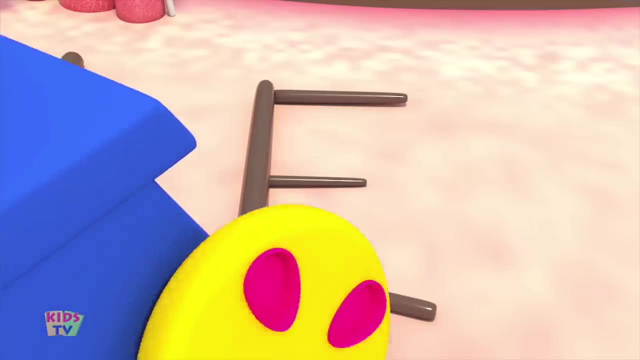 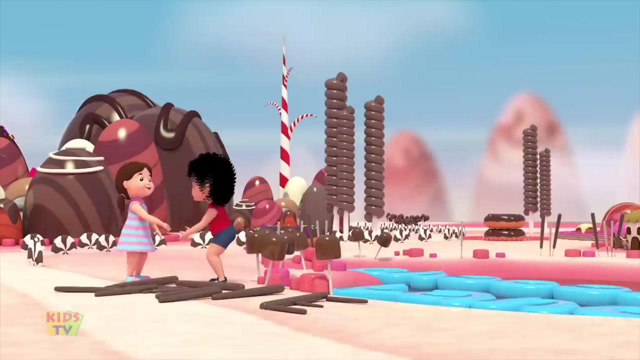 Using those sticks, you kids have to create the letters E and F. Remember, unless they're perfectly set, you won't find them. You will work in teams for this Wondersome. Now let's take a look at F. Uh-oh boys. 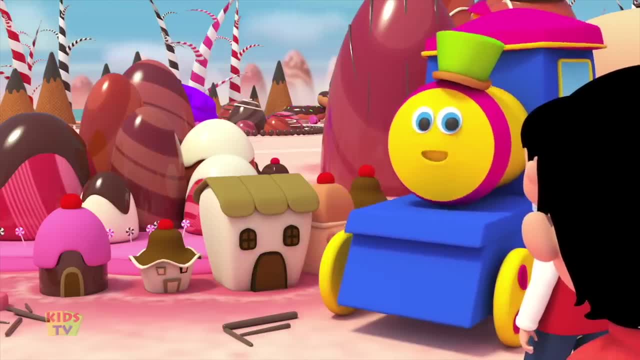 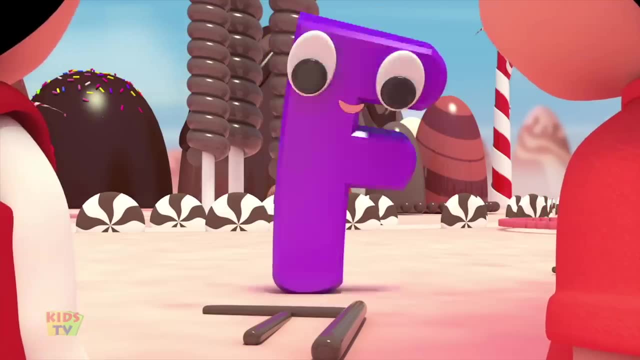 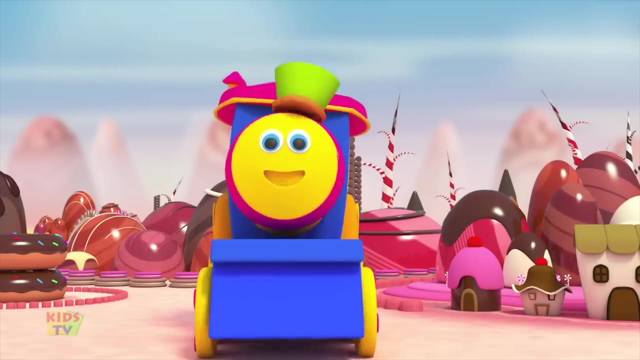 The F looks out of proportion. Do you think you can remember what it looks like and try again? Thank you, kids. I got real tired of hiding. Kids G, H and I are hiding in the burrows of the chocolate mountain. They're very tricky to get a hold of. 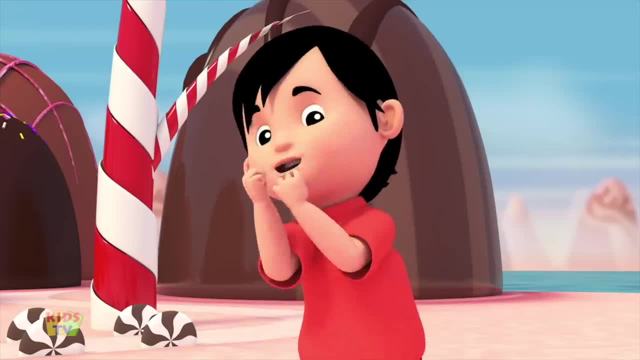 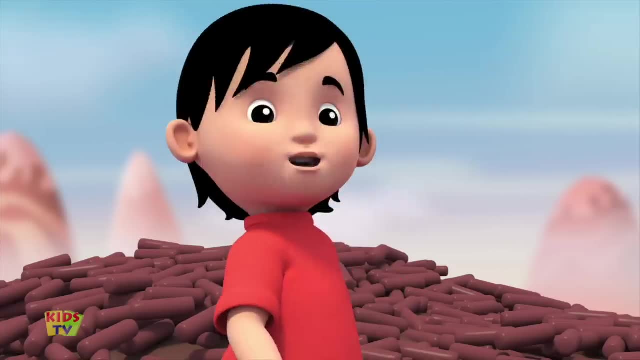 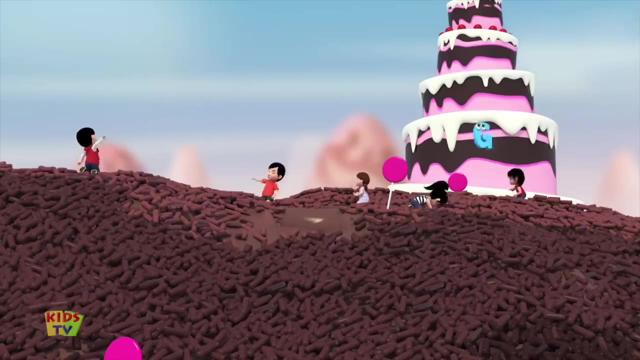 Do you think you can grab them all? Of course, I can't wait to get my hands on those little letters. So that's how you want to play? Very well, then, Come on, friends, dig in. Oh kids, I loved watching you try. 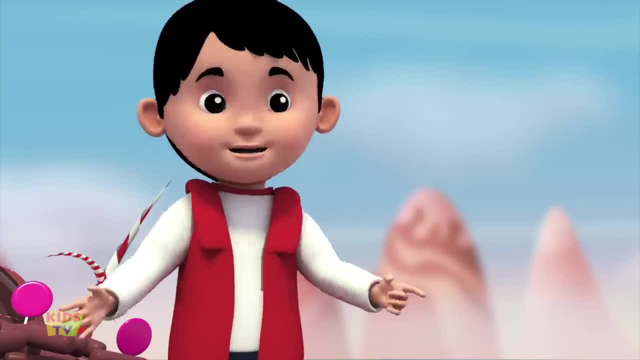 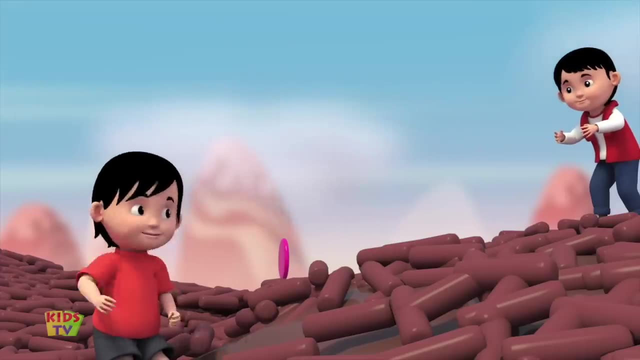 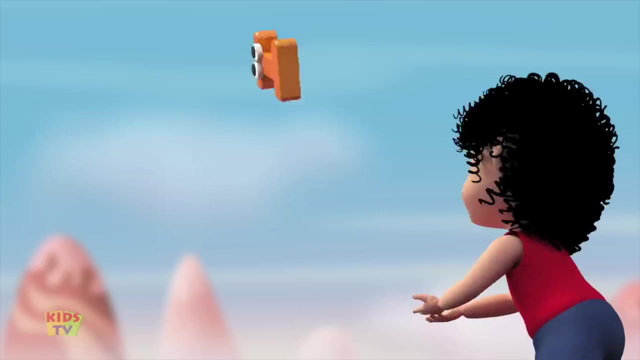 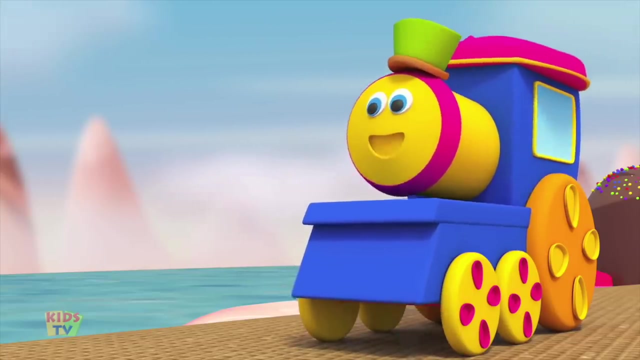 But you'll never catch the letters this way. I have an idea: Yay, Hooray, One, two, three. Great job kids. Up ahead there's an ice cream truck where you'll find J and K, But how are you going to find your way? 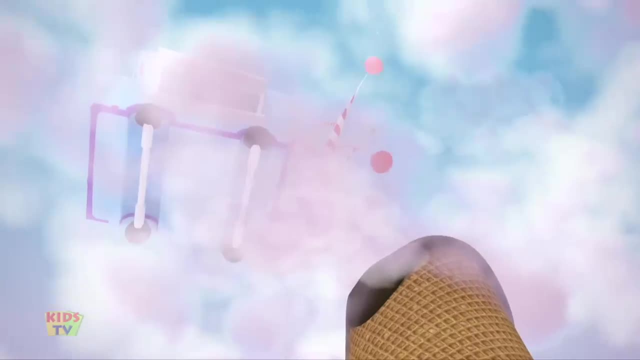 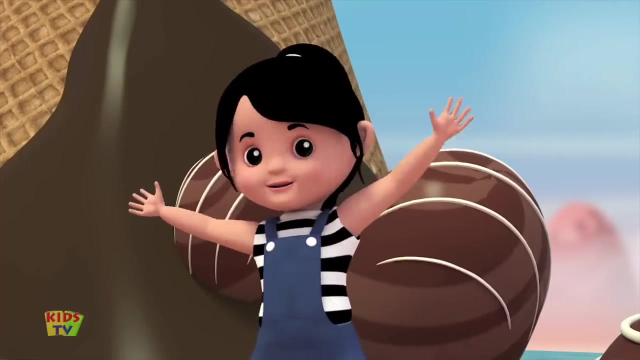 Suddenly all the kids looked sullen. How would they possibly get that high in the sky to find the letters J and K? Hey guys, In Chocolate Lane the shops are made of candy cane. In a land where hot dogs are so handy, the clouds are made of cotton candy. 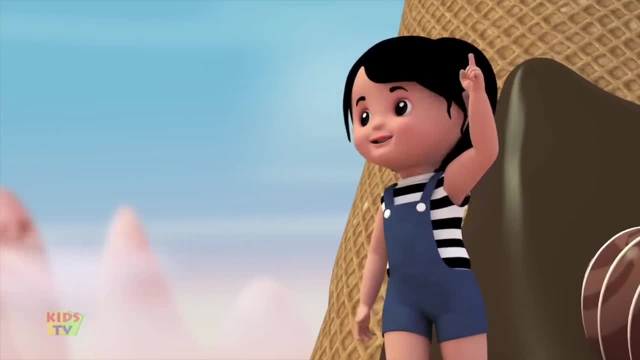 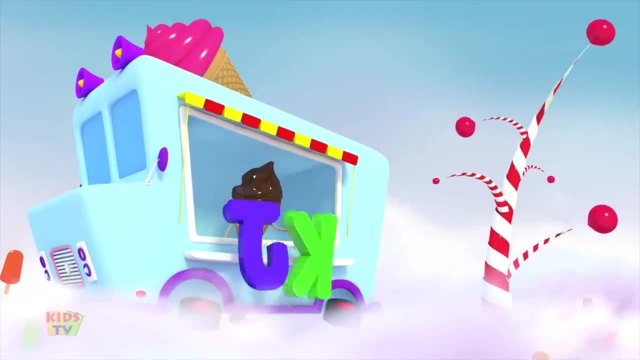 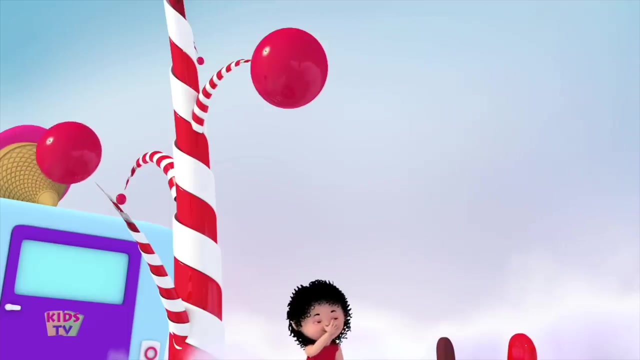 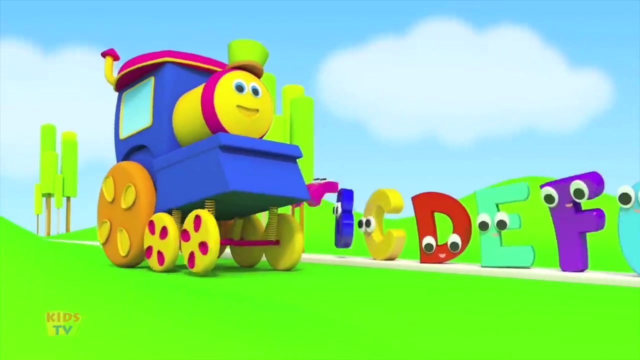 What do you say? we surf our way up to the ice cream truck in the sky. That's brilliant, Polly. Hi guys, Hi J, Hi J, Hi J. Okay, kids, It's time to find the rest of the letters. 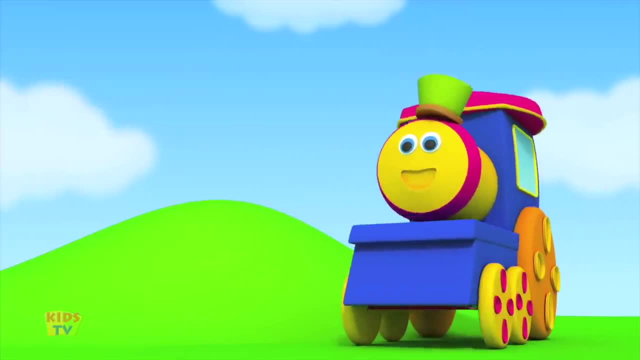 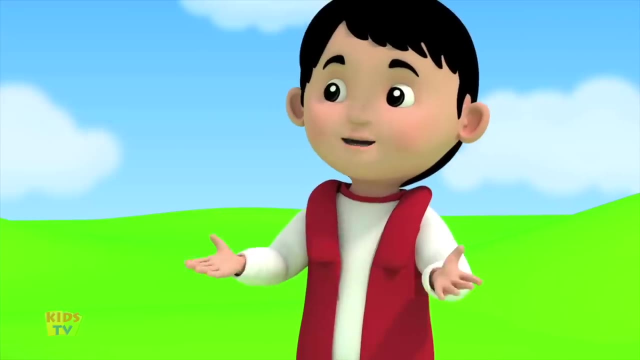 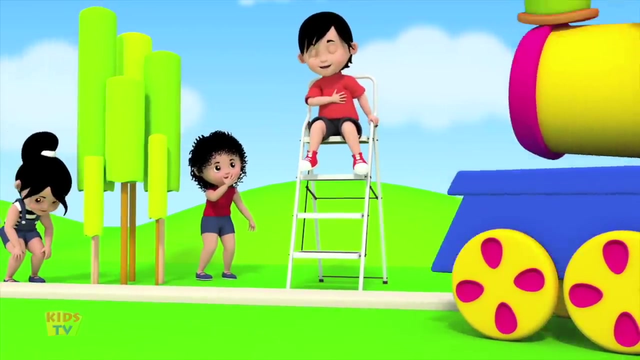 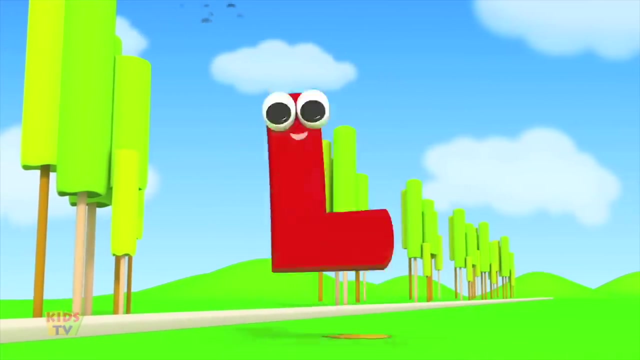 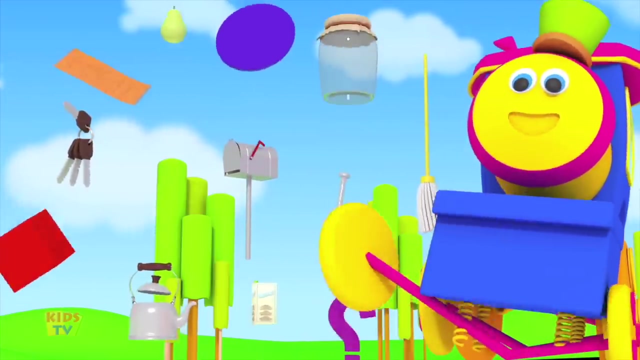 Let's start with L. Each of you need to name something that begins with the letter L: A lamp, Lemon, Lipstick, Ladder, A leaf, Hey guys, Hey guys, Great job. all of you Pick out the objects that start with the letter M. 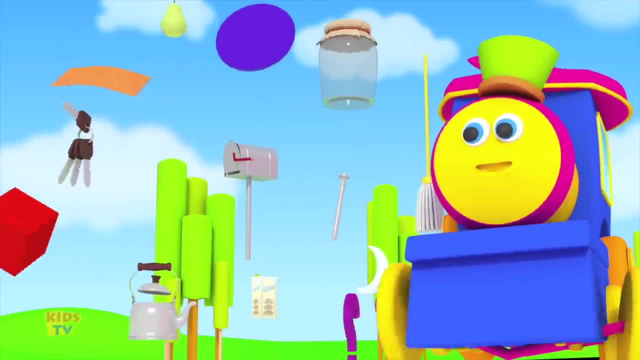 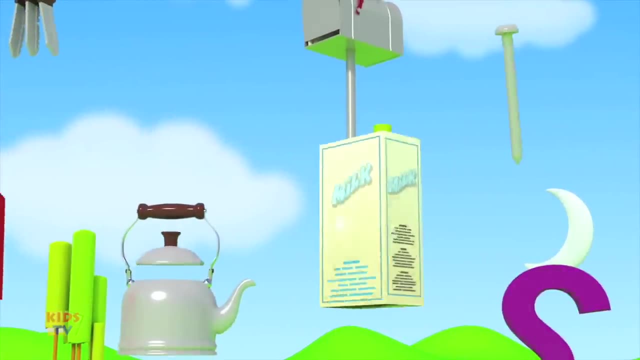 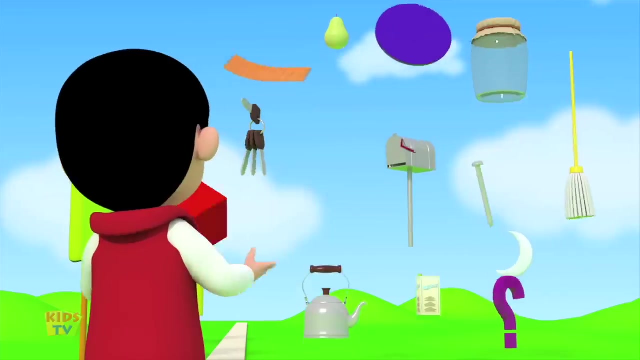 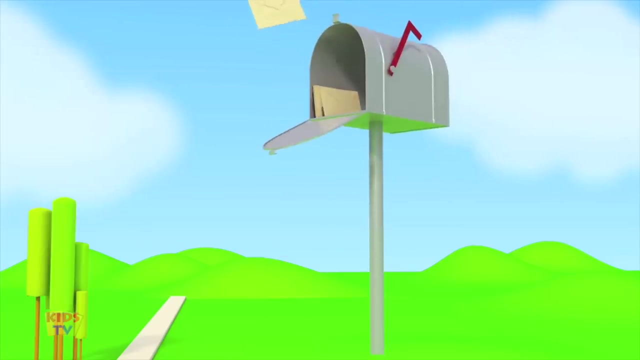 If you pick them all right, Mr M will join us. Are you ready? Let's start with little Jill first, this time, Milk Mop. I want to pick the moon Mat. Well, I pick the mailbox, Hooray. 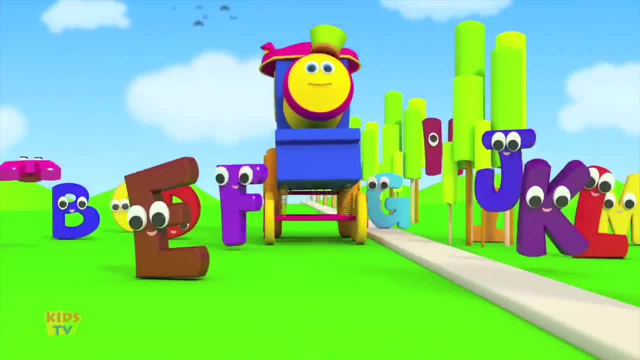 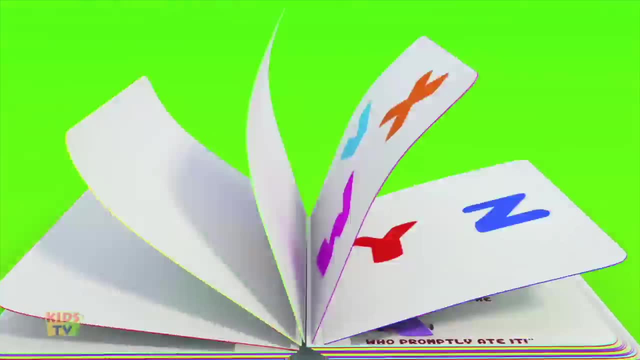 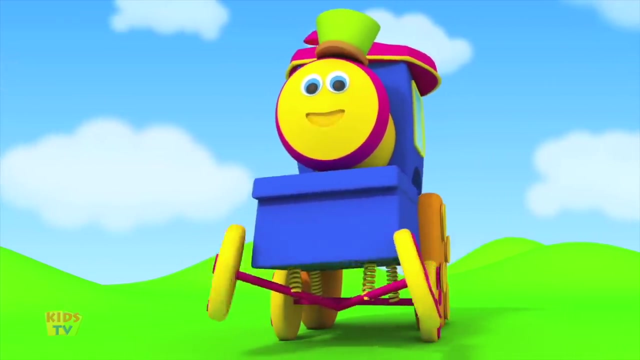 Kids. if you haven't realized, you've already found half of the alphabet. Here's a little story with a few words missing. There are images to match the missing words. If you guess them correctly, you'll find the letters N, O, P and Q. 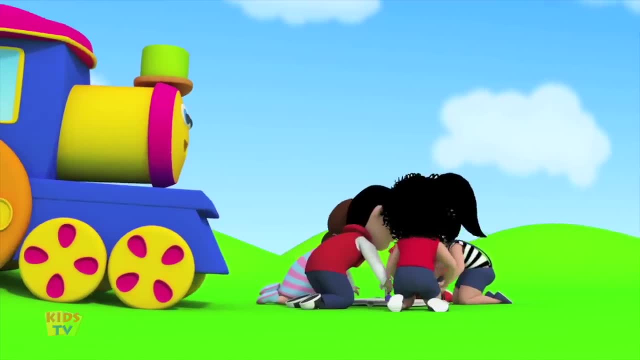 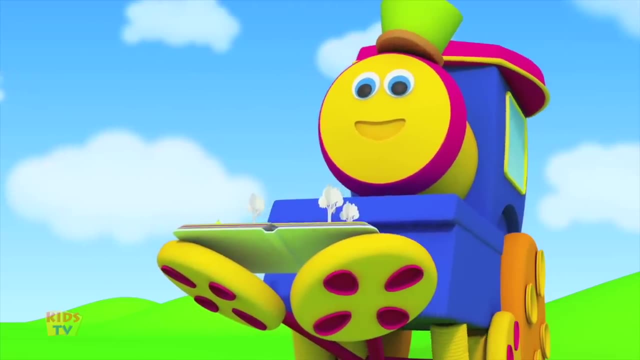 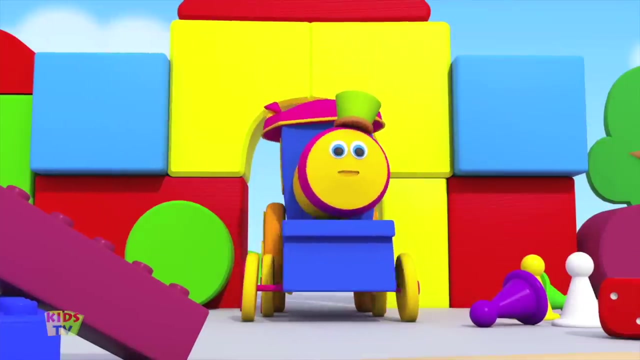 Yay, I love story time. After spending a few quick minutes on it and filling in the blanks, they handed the book over to Bob. They're absolutely right, kids. Yay, You kids are absolute geniuses. So let's see if you can find the next three letters just as quickly. 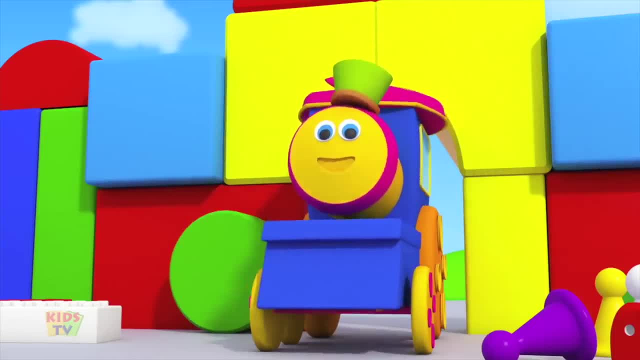 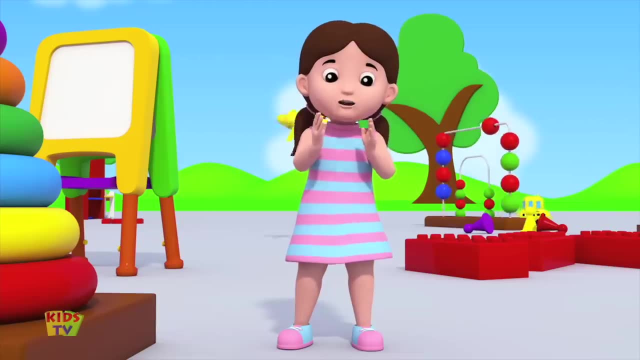 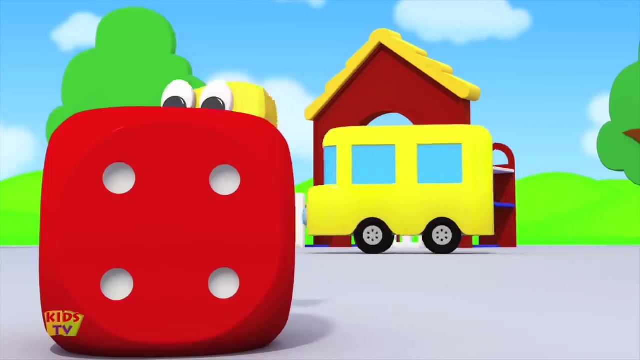 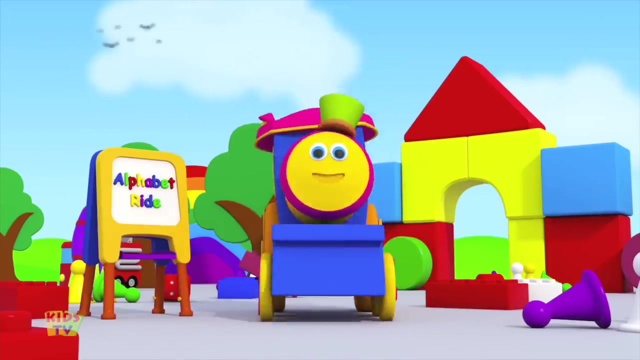 They are behind shapes. You can see them everywhere. You just need to look closely and find shapes that begin with the letters R, S and T. R is for rectangle, S is for square, T is for triangle. Well, kids, are you ready for the last leg of this hunt? 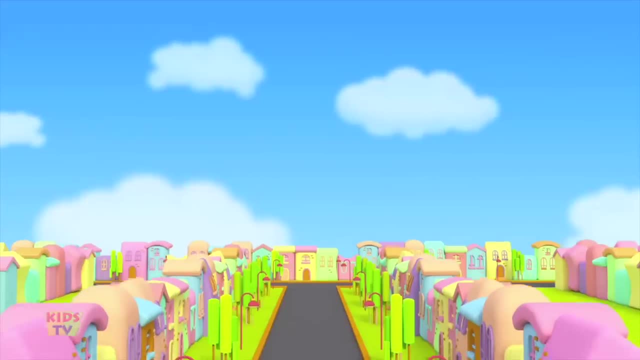 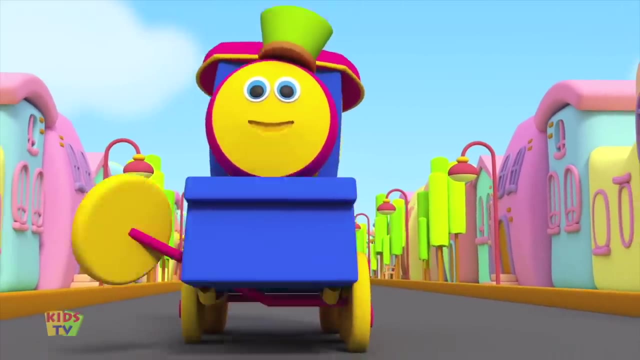 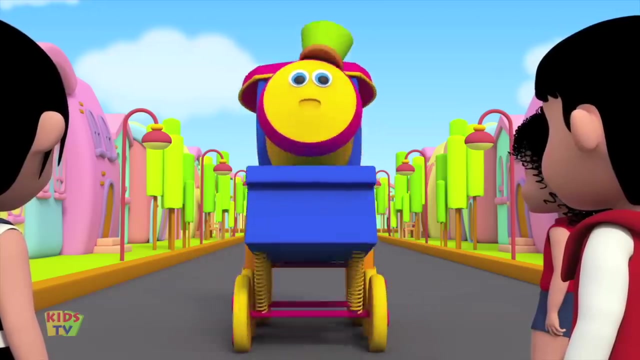 Let's go. They all followed Bob and reached the alphabet's adventure land. Well, kids, here we are, The land where all the adventures started. It feels good to be back here. I've made this simple for you: There's just one task and you'll find all the letters together. 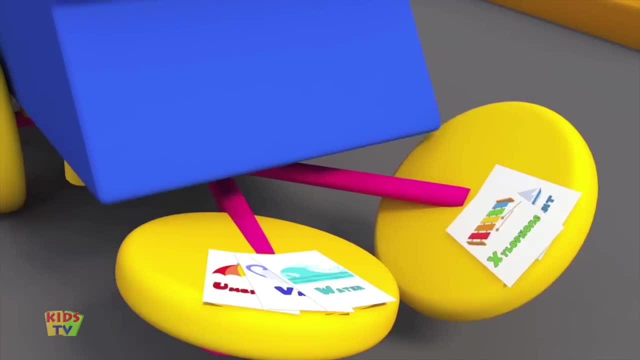 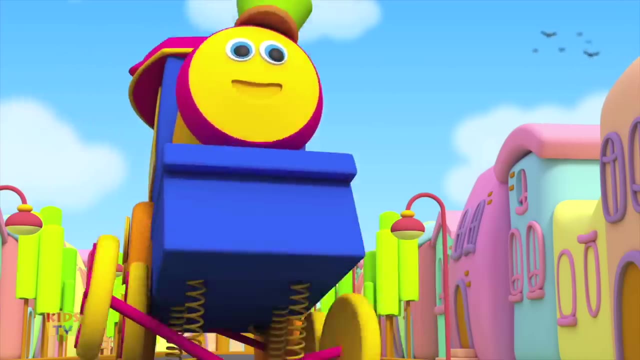 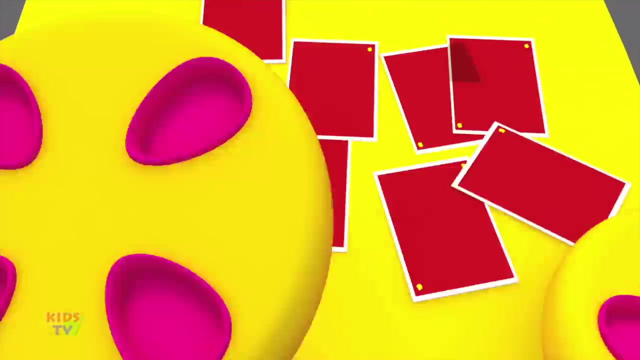 What is it, Bob? It's a memory game. Cards with objects drawn on them are placed upside down. You kids need to match the cards And when you do, you would have found the letters corresponding to the image. Bob put ten cards placed upside down, shuffled them a bit. 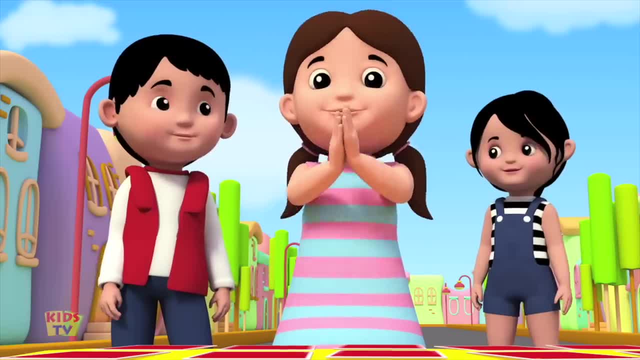 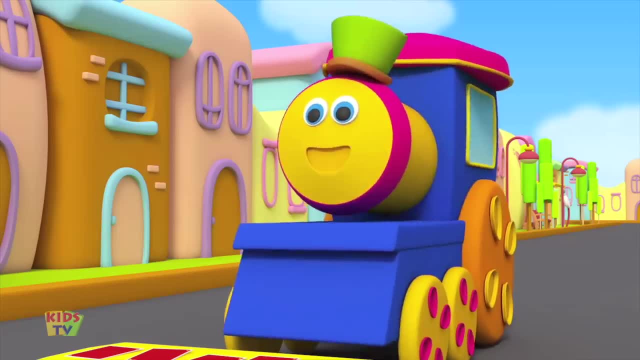 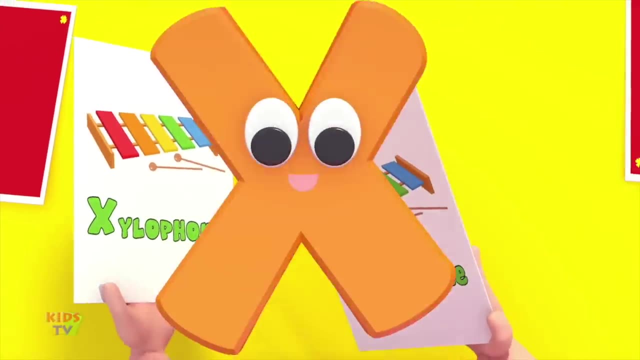 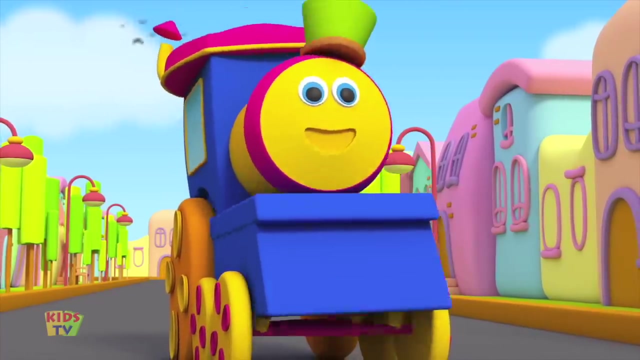 and asked the kids to take turns in picking them out. The kids were able to find all the letters. Oh Yay, Good job Jack. Oh my God, We found them all. Great job everyone. Now are you ready to finally meet Z? 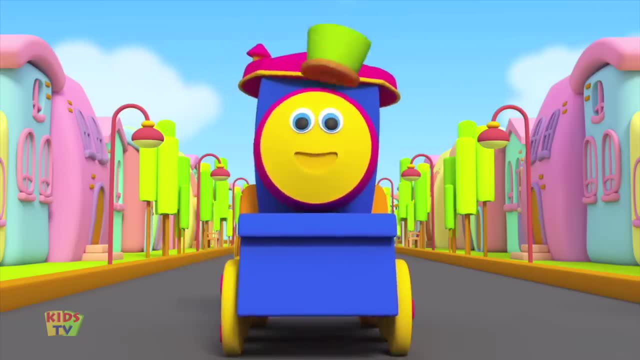 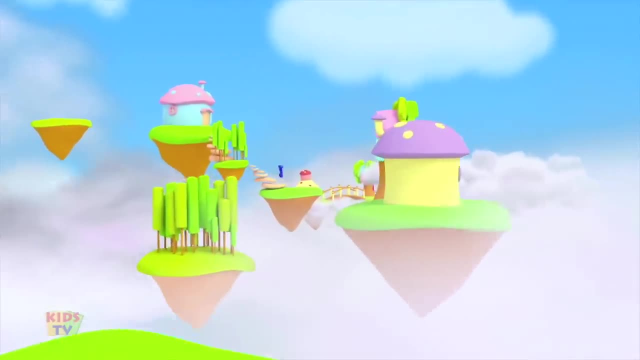 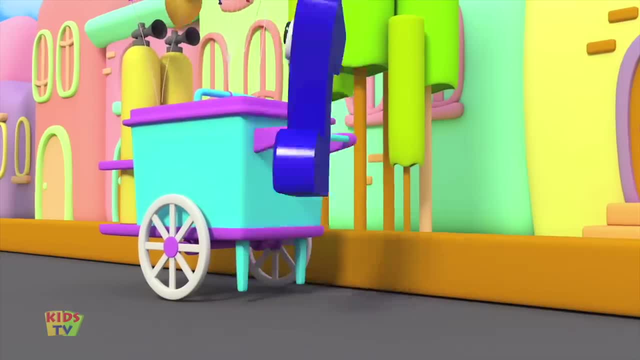 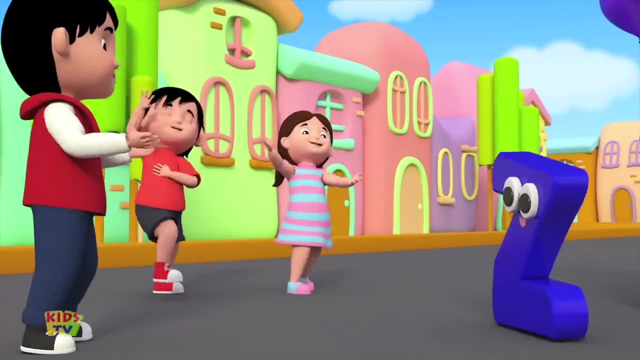 Ha, ha ha, Easy Z. I'm so happy to see you all here, Bob, like you said, your little friends are really very smart. Thank you, Z, And I'd like to thank you all for putting together this hunt for us.